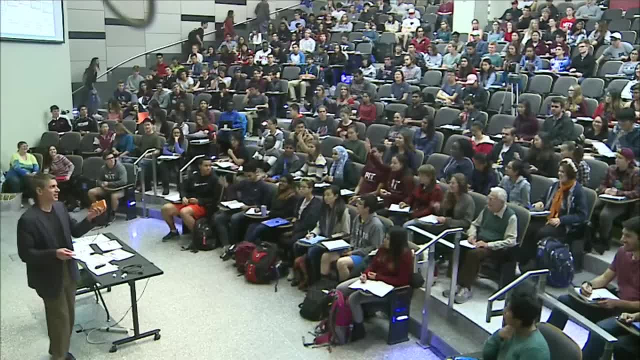 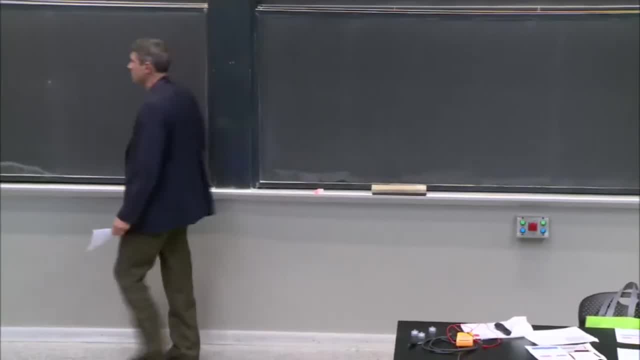 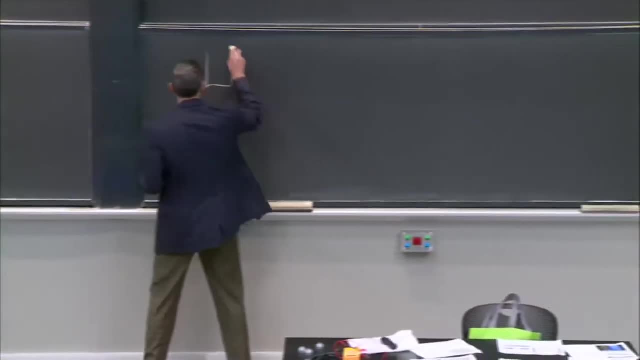 it before, but you've never had one this accurate as the 3091, right? Yeah, Oh, you never know when you need a voltmeter. You should always carry it with you with the periodic table. Now, on Monday, this is what we had I'm going to. this was a conduction band. 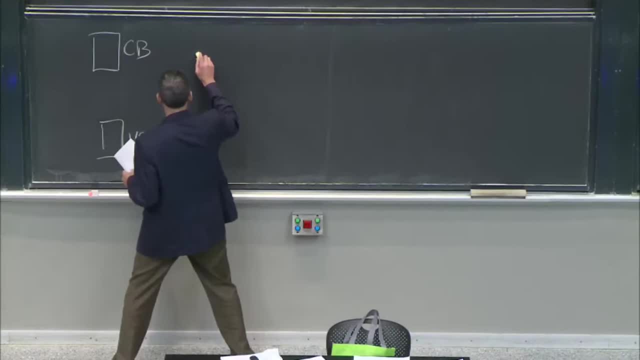 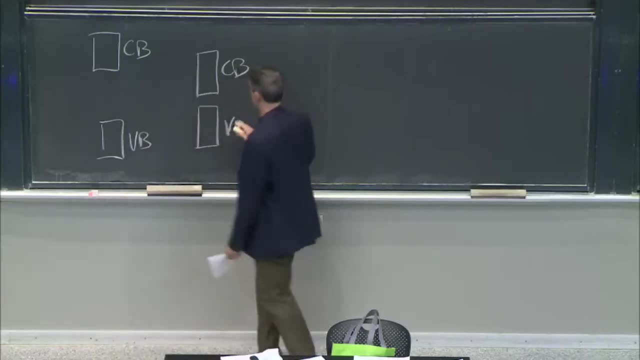 This was a valence band, And then we had a conduction band and a valence band that were a little bit closer together, And then we had this case where maybe it's it's it's filled up somewhere in the middle of a band, And remember the valence band. 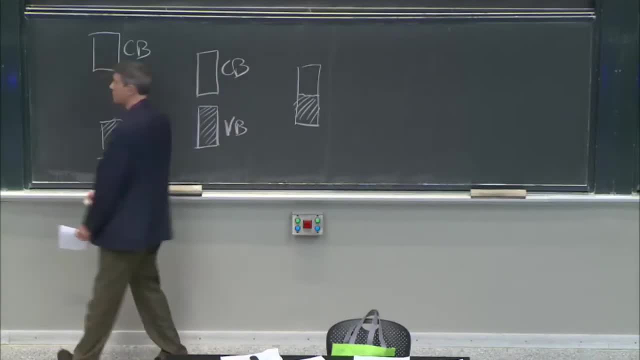 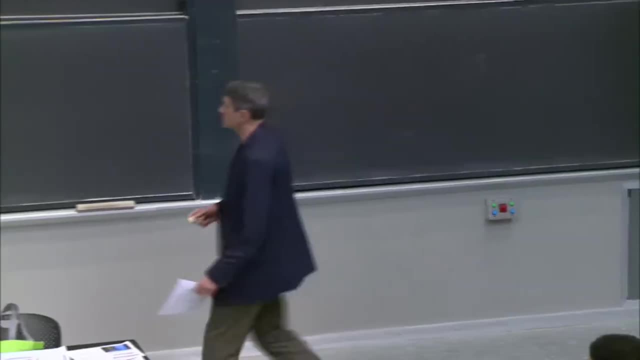 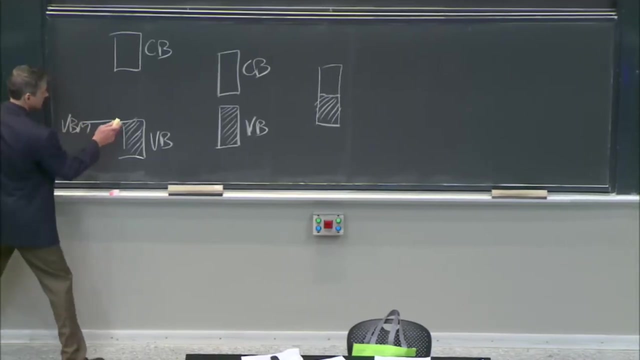 is filled with electrons and the conduction band is not right In in the simplest picture. And this, this, this, this difference in energy between this VBM right, That's, the VBM, the maximum level of the valence band, and the CBM, the minimum level of the conduction band. 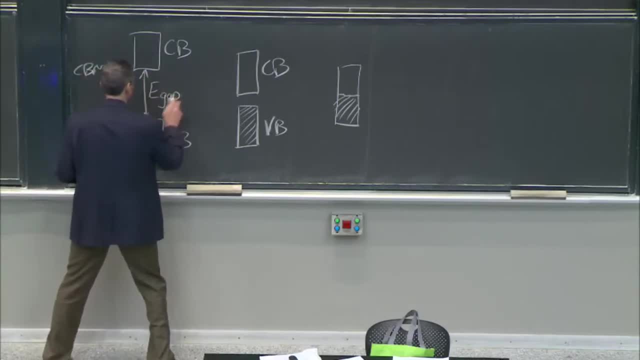 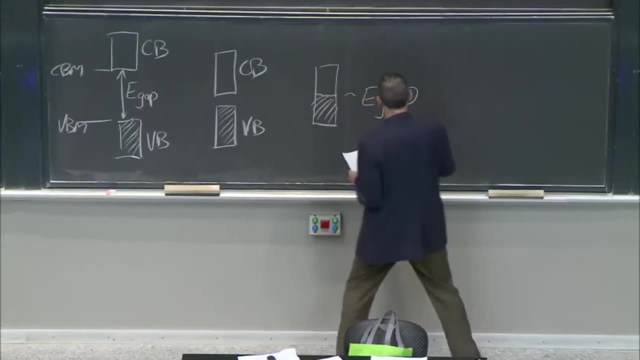 right. So the energy difference is the gap of the of the material. right Here you can see, energy gap equals zero. Well, in this case it's a metal or, if you want, it's a conductor, And we'll talk about. 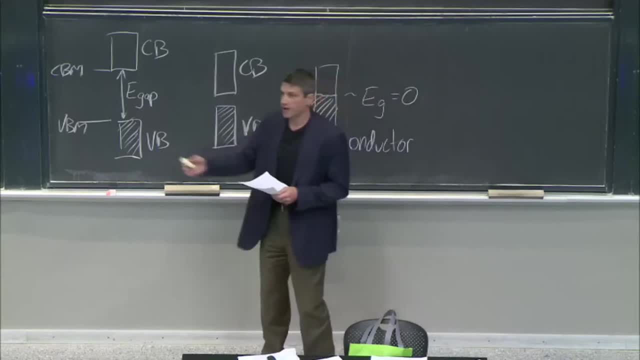 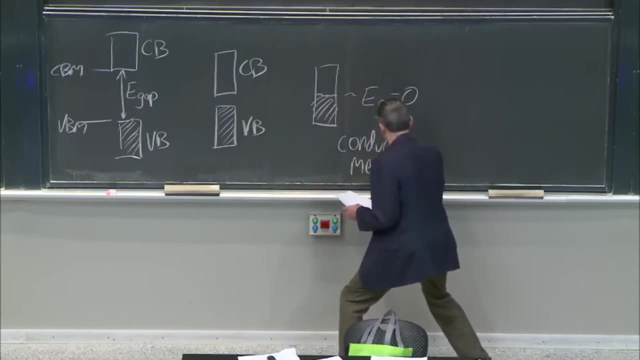 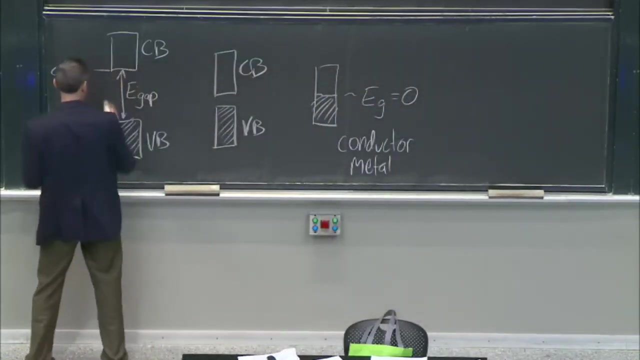 why it's a conductor- more on Friday, but a little bit today- why metals are conductors Today. I really want to focus on this case. right, So that's a metal when there's no gap in the material. If the gap is large, then that is an insulator. insulator, right? Oh, what do I mean by large? 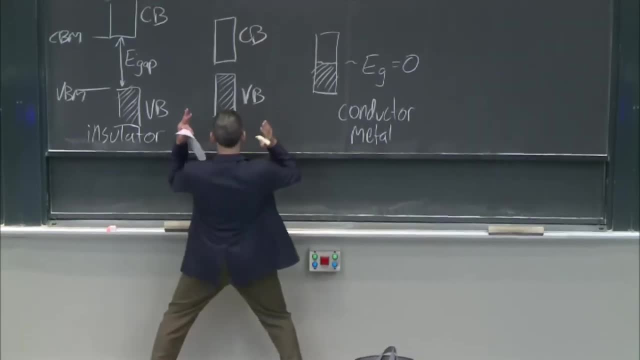 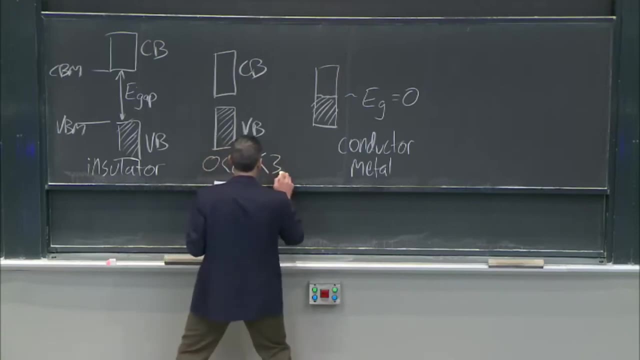 Well, what I mean is it's not in the range of this special case, which would be, say, zero, less than the gap, less than around 3.5 electron volts. This is the case that I want to talk about today. I want 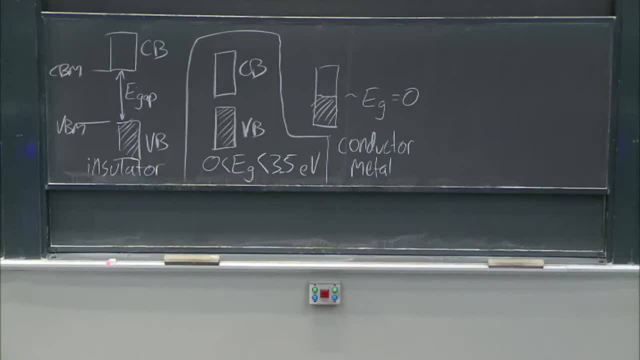 to spend today talking about semiconductors. Those are, those are called semiconductors. Um, let's write that here. Semi conductors, Uh, sometimes semiconductors. sometimes you'll see them called metalloids. Oh, that you know. 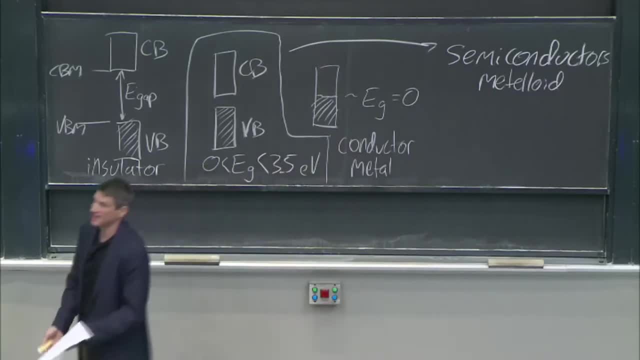 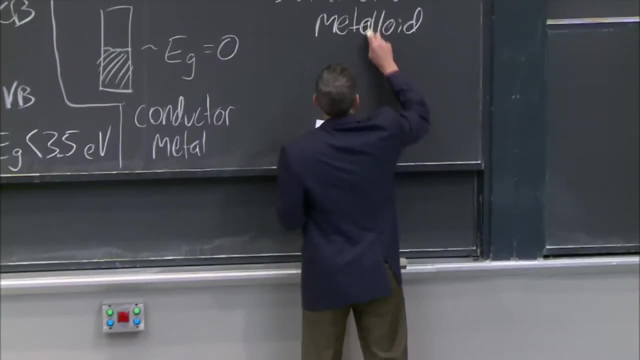 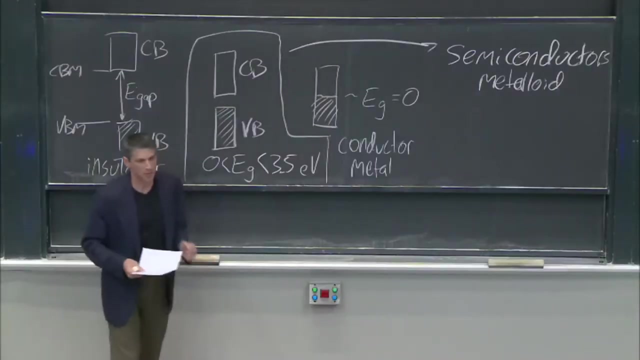 sometimes you'll see them called insulators with small gaps. They're all kind of right And and the reason, but so metaloid, thank you, Or okay. Now, the reason why we classify these and why this range of gap is so important is what I want to convey to you. 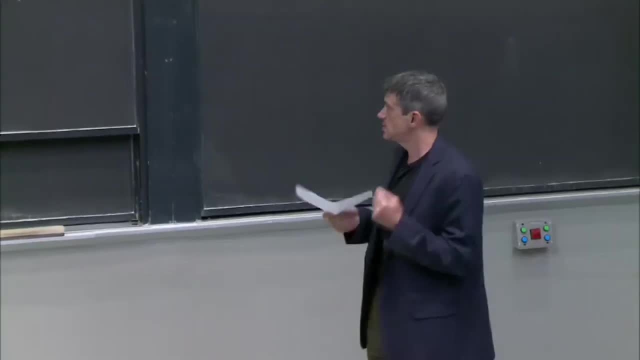 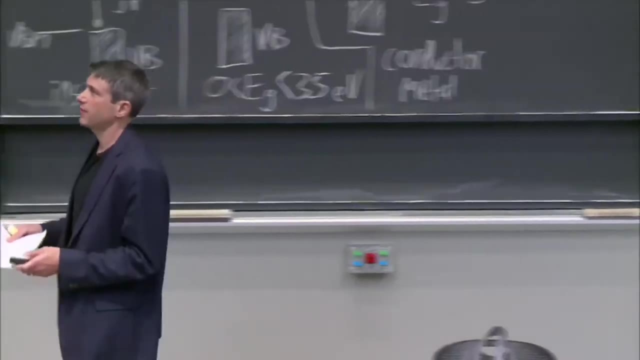 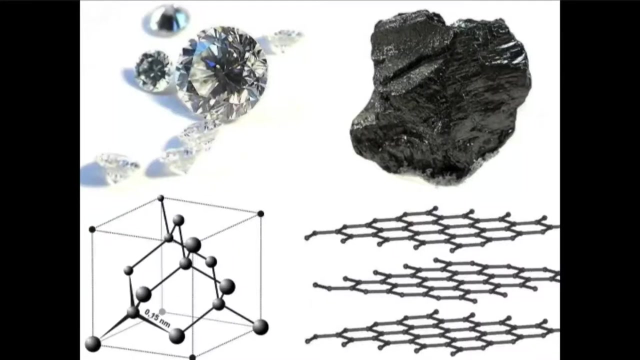 today. These are really special materials, these semiconductors. Okay, Now, before I do that, I I want to. I want to just clarify one thing, Okay, And I'm going to use diamond and graphite as an exam, as as a an example. on Monday, what we did is we- we talked about the concept of bands with a 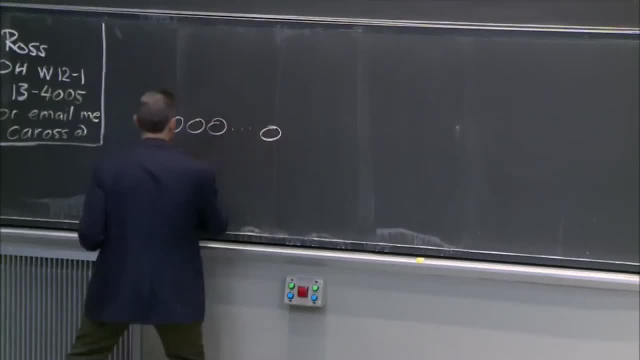 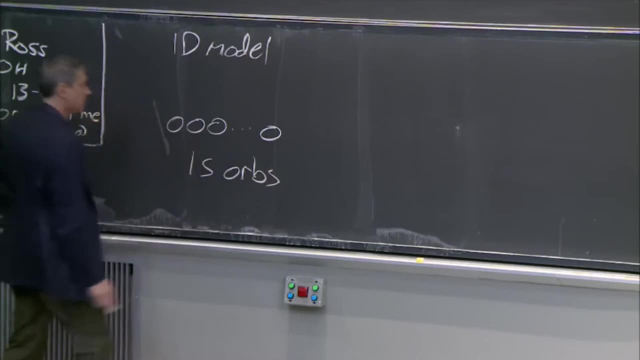 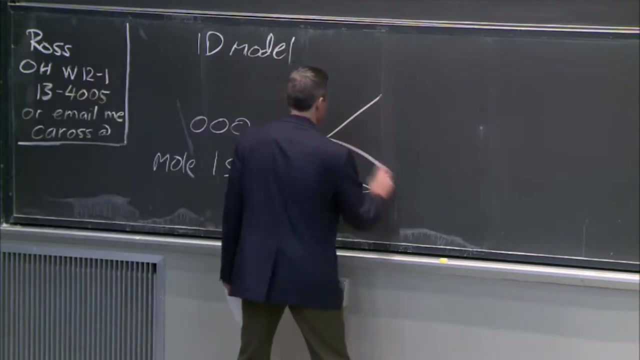 very simple: one D model right. This was a one D model of S orbitals. one S orbitals. I said, well, if I have a mole of one S orbitals then that goes into a band And I called it a one S band right. 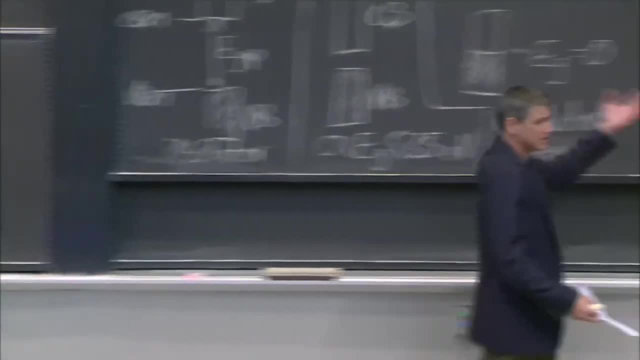 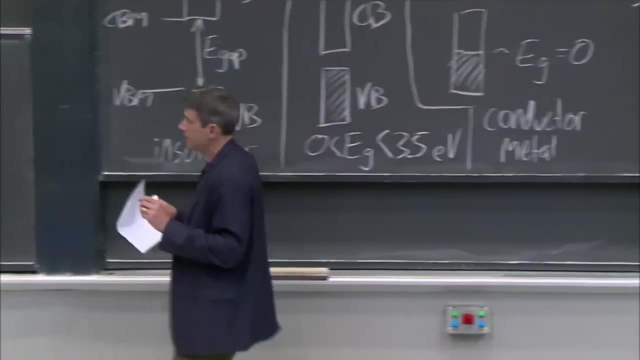 And we say: well, if you fill it in different ways, that is what determines the properties. But I want to be clear, And I stress this on Monday, I want to stress it again: All right, Whether this forms this and then the next. 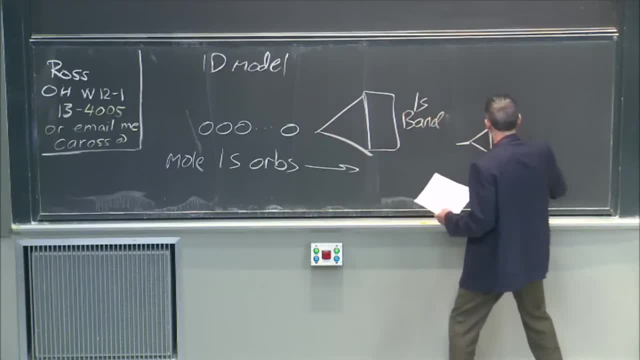 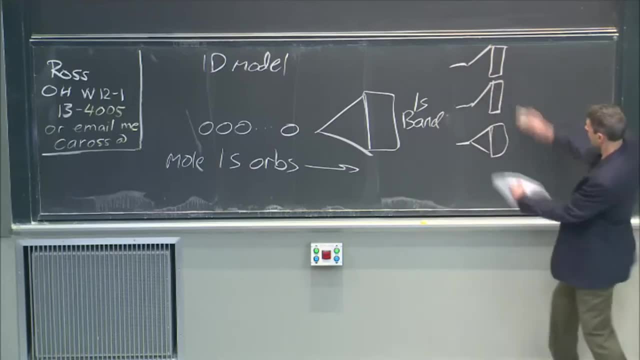 step. you know whether you get like a one S that forms a band like this and then a two S that forms a band like this and then another one, you know maybe two P like this or whether there's breaks in them or maybe these kind of overlap. So you get like overlap and you get sort of 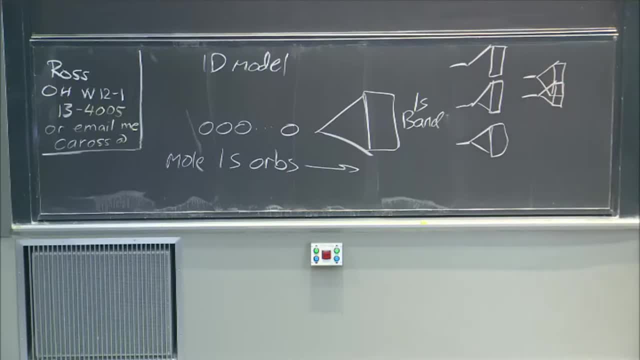 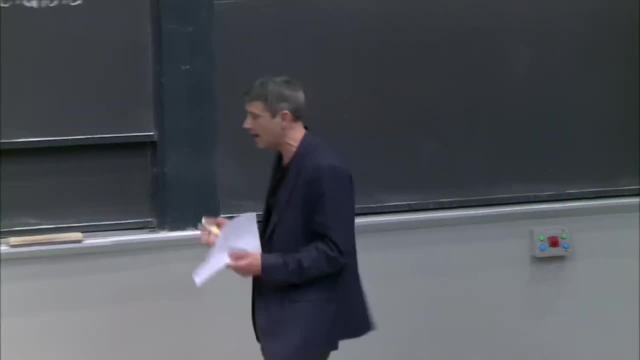 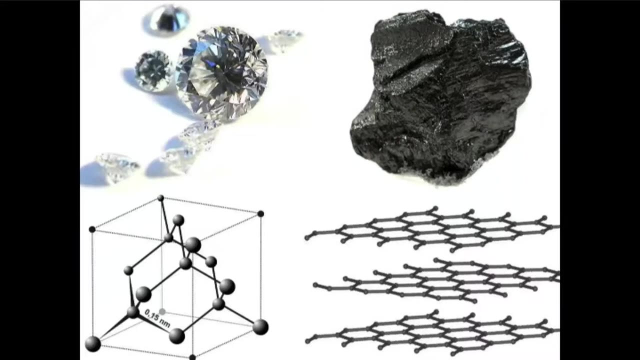 something like that. right, All that depends on more than just those atomic orbitals. It depends on more. It depends on how these things are bonded. This is such a great example. I've got the same element here: It's carbon. There's nothing else in. 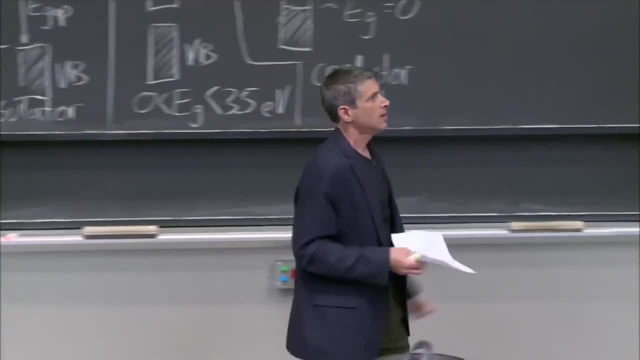 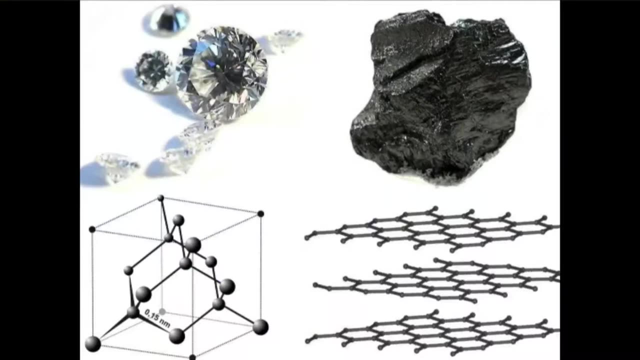 this system, carbon, pure carbon. everywhere is carbon, But on the one hand, I've arranged it in a certain way And on the other hand, I've arranged it in another way, and their properties couldn't be more different. Right And so so, like you know, just to take this, you know, just to take this, you know. 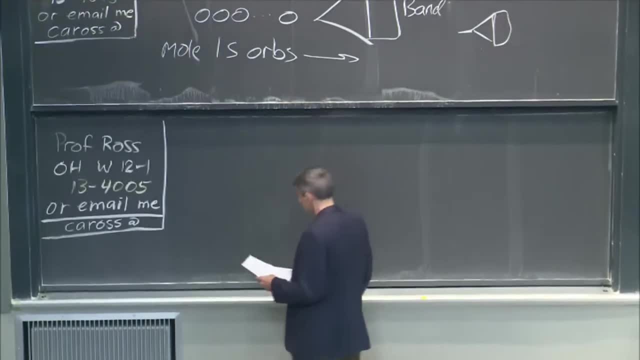 Right, And so so, like you know just to take this, you know just to take this, you know just to take this, you know a little further, right, If I, if I think about diamond on the left, diamond is an insulator. 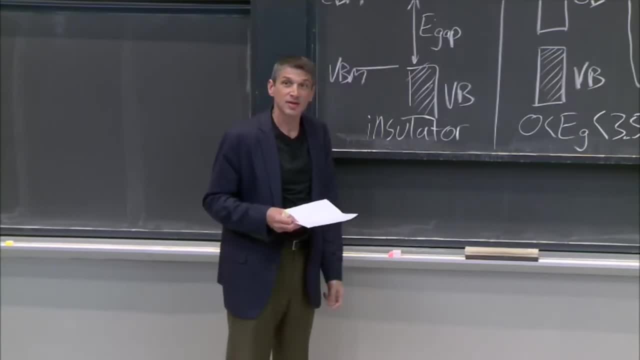 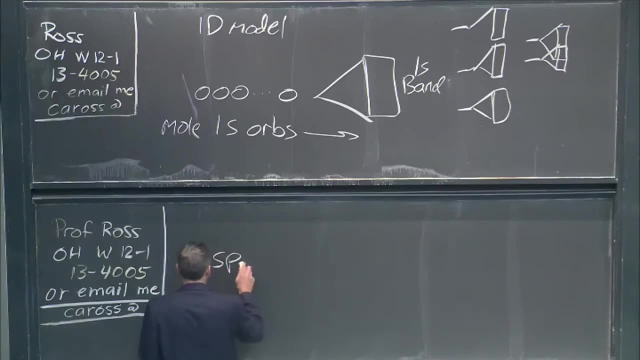 Diamond has a gap of five and a half electron volts. five and a half electron volts, It's an insulator. right Now you say: but okay, that makes me think of methane. Remember methane? you had these SP3 states, SP3, SP3, SP3. 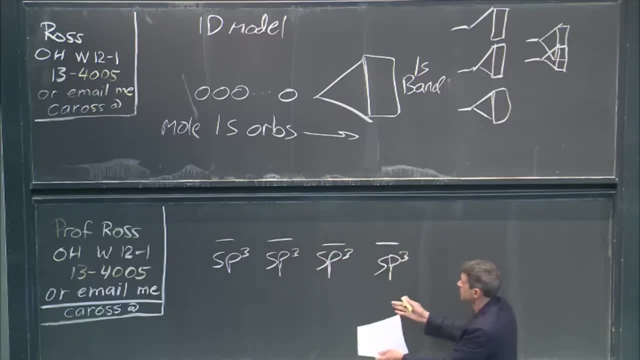 Okay, And the reason it formed SP3 is because all these H1, 1S states came along right. H, H, H, H. These are 1Ss, 1S, right, And so carbon came along. and it said: well, if I arrange, if I got four of you here like this and I 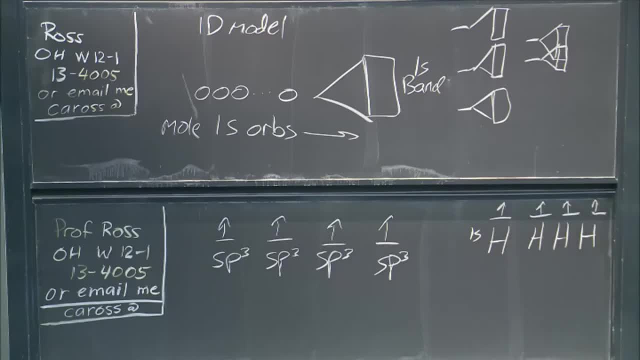 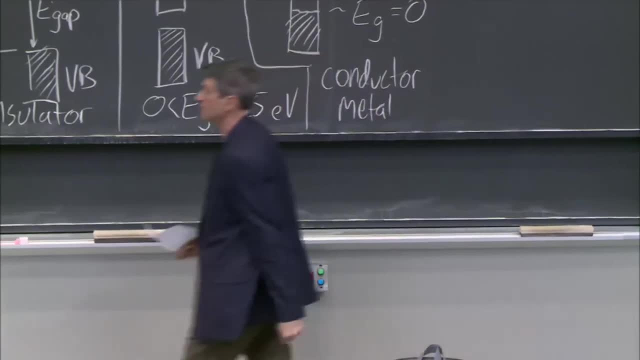 arrange myself. if I arrange my orbitals in such a way that then I can arrange the atoms so that they're minimizing repulsions, That gives me methane. That gives me the ground state of methane. But the only way to do that is to have four. 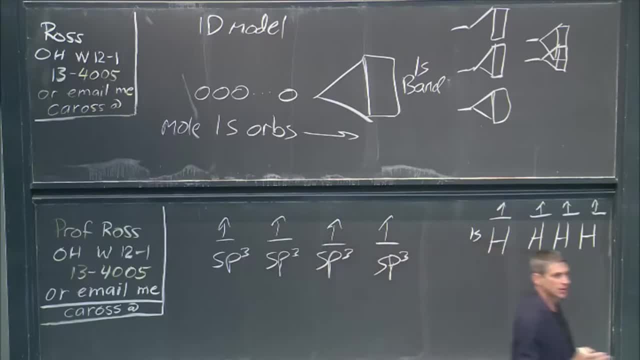 equivalent orbitals. Those are hybrid orbitals. We talk about this when we talk about hybridization, The idea being that if I took one of these and one of those, right, So now you can imagine how it's going to look. You know all this. now, right, There's a. there's a 1S orbital of hydrogen. You know that those will form a sigma and a. 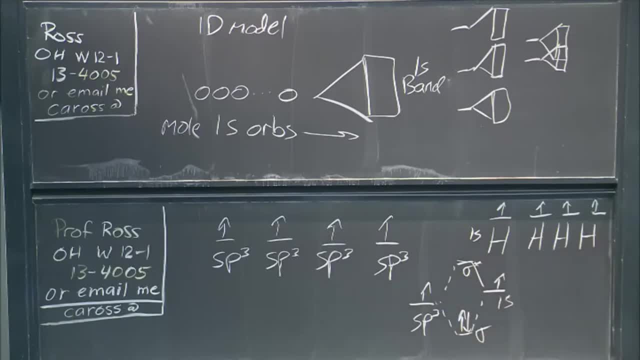 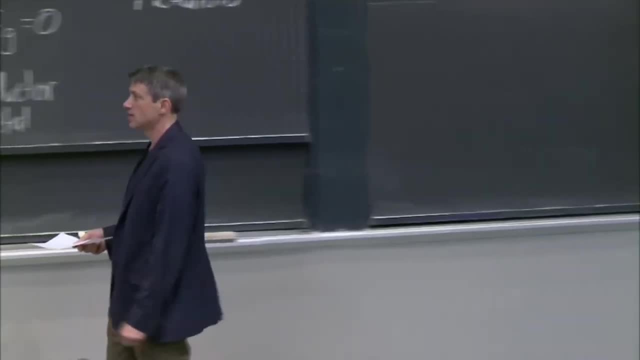 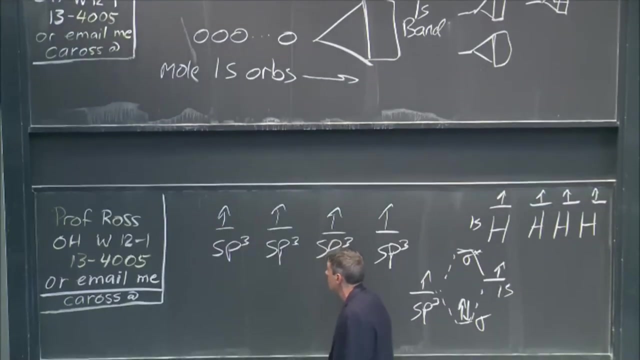 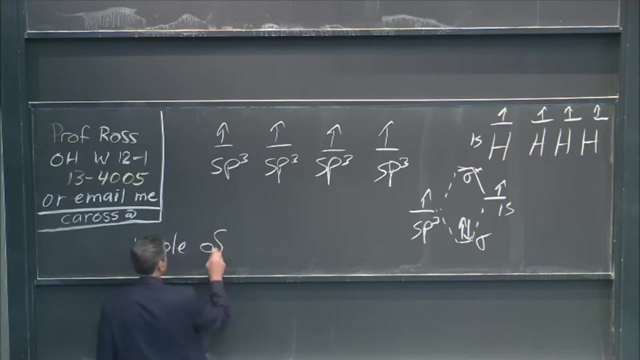 sigma star and occupy the, that bonding orbital. That's the idea of methane, That's the idea of molecular orbital theory, with some hybridization right, And it's going to form those bonds along each direction. But now I'm talking about something different. I'm not talking about such a simple case. I'm talking about one mole of SP3. 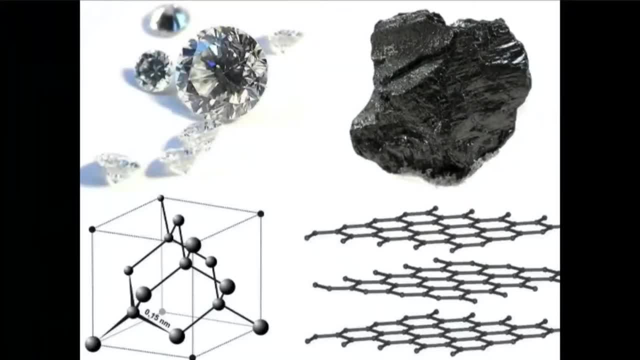 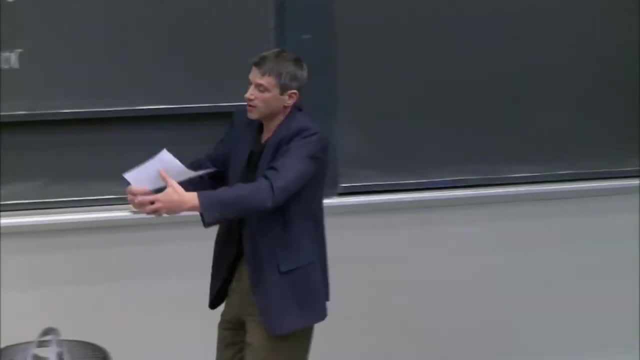 That's what diamond is. Look, the carbon atoms have done the same thing. They've said: hey, wait a second. Okay, There's four hydrogens. It's like 10 to the 23rd carbons- all in one small space. How can we organize to lower our energy? 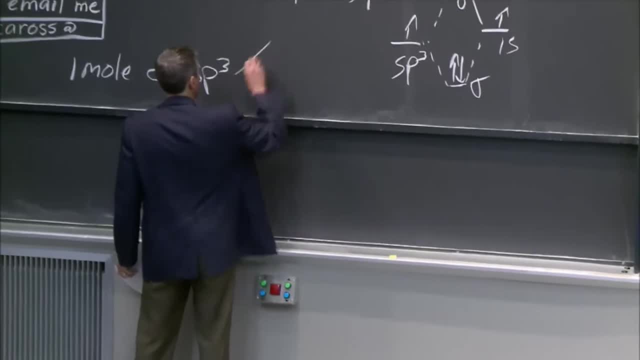 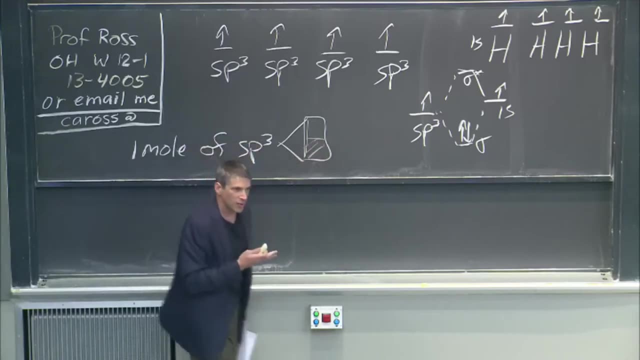 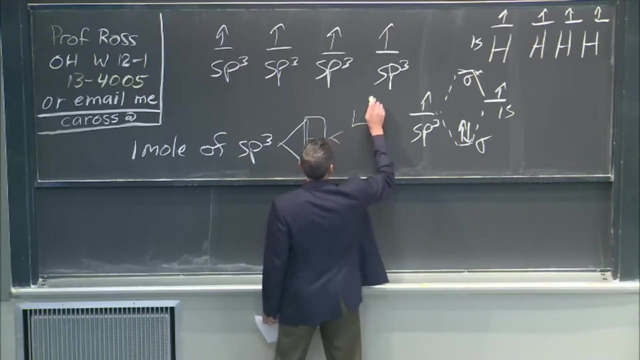 And so they form. Well, we know this, that it's going to form a band, but it doesn't just form a band and then half fill it. That's not what diamond does. No, actually diamond breaks this apart so that you have. 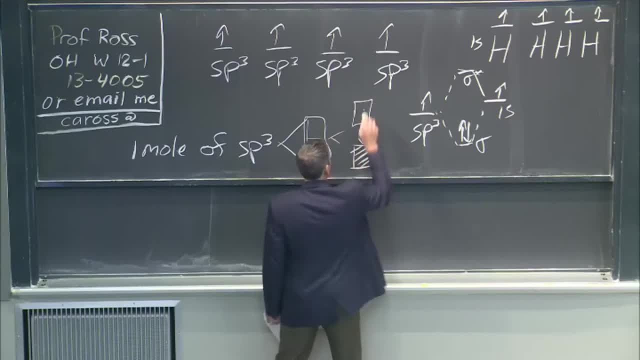 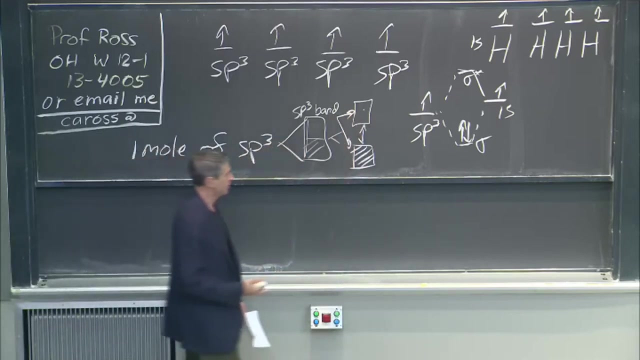 a huge gap and those are filled and that then those are not. So this is not. the SP3 band in diamond breaks apart into a valence and a conduction band. The valence band is full, The conduction band is empty. Why? 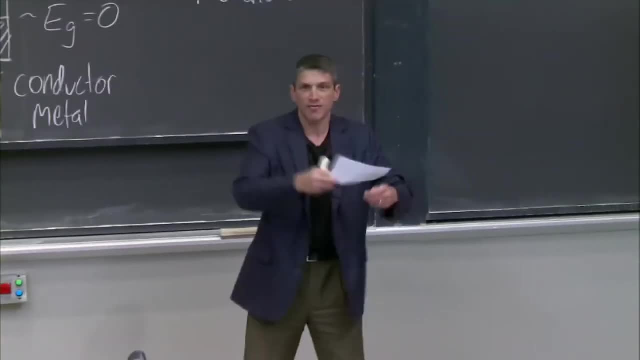 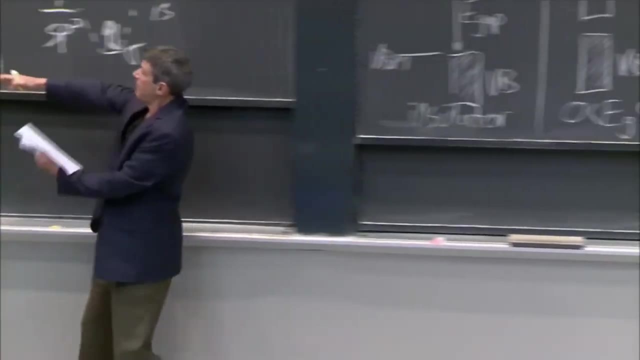 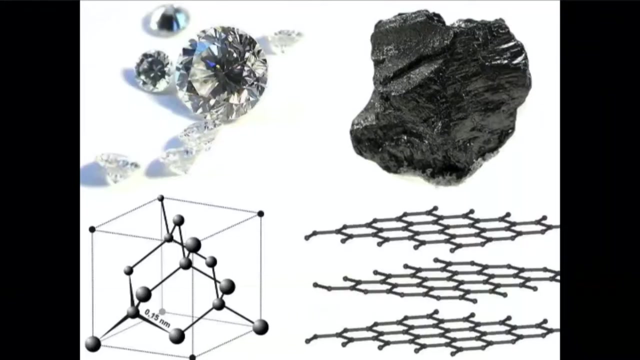 Well, you don't need to learn the specifics of how to get from there to there, But I wanted to show you how complicated this is. I won't ask you whether the SP3 band splits or not. I just wanted to show you how dependent this is, because now, look, you can understand this now, right? 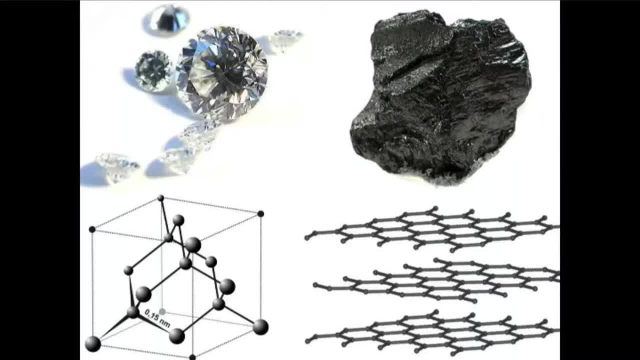 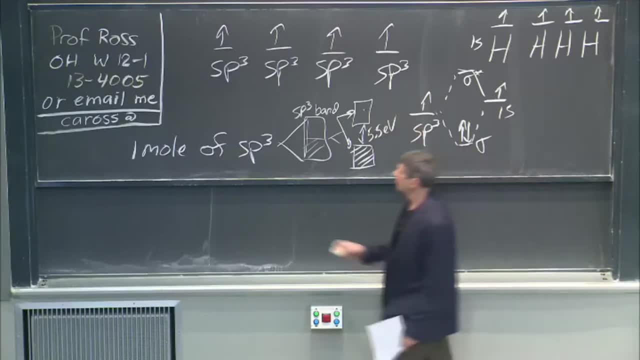 So I got four electrons per atom going here There's a huge gap and then nothing in there. That's diamond: 5.5 EV gap, One mole of SP3 in diamond. Now it depends on the structure. If I had just put them together in some amorphous soup with no whole amorphous, that's a word that's coming. 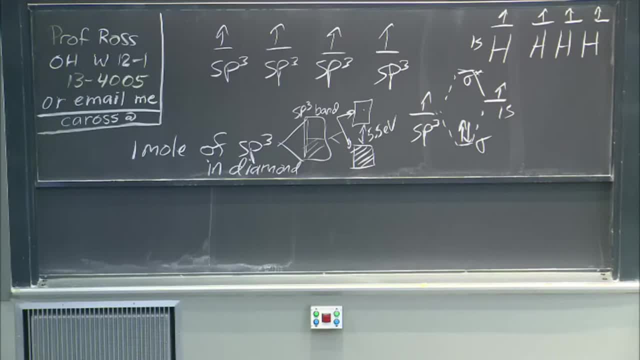 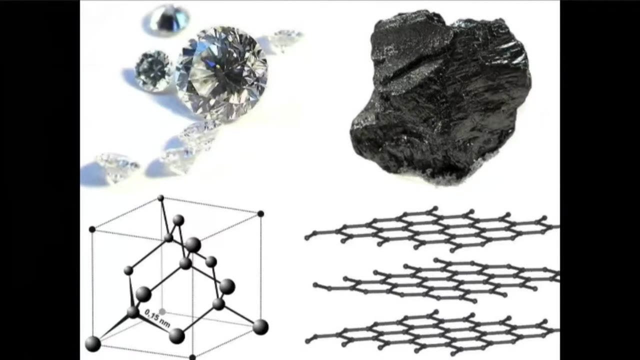 Later. But if I just put them together with no order, I wouldn't get this. This splitting. They did graphene, which is one of those sheets, and make stacks, and you got graphite- It's another form of pure carbon. In that case you've got your SP2 bonds that form in the plane and those also split and they fill. 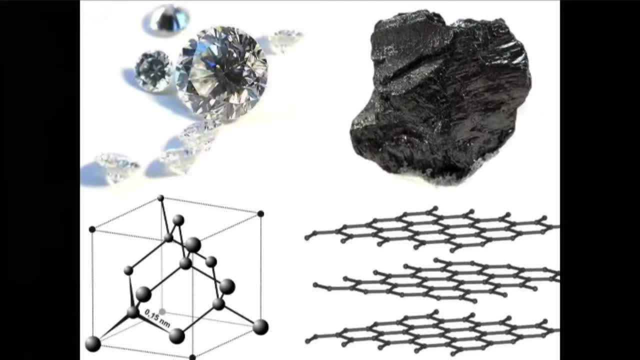 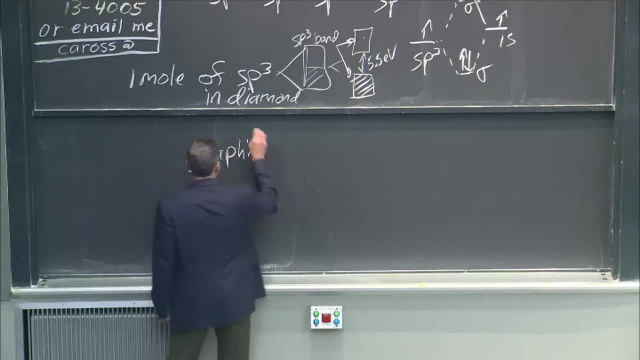 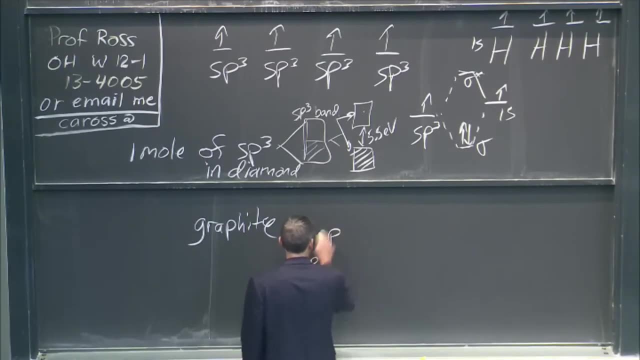 But now you've got your PI bonds right And those don't split. So in graphene right. So in diamond In graphite, what you get is you've got your SP2s right, You got a mole of those and you got your P electron. 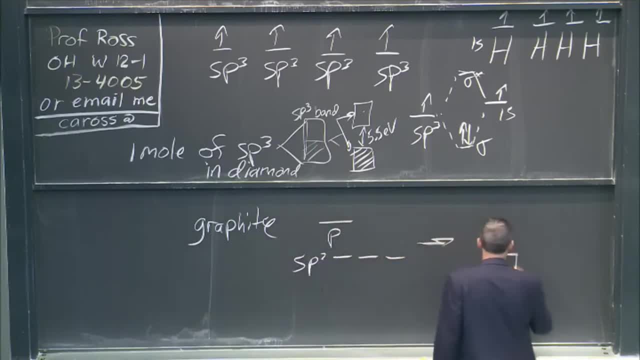 Remember those. right Now you do a mole of that and you got the same thing. But see, now you got these are the SP2 bands, SP2 bands. It also split And remember I've got my electrons here, my SP2 electrons and those there. 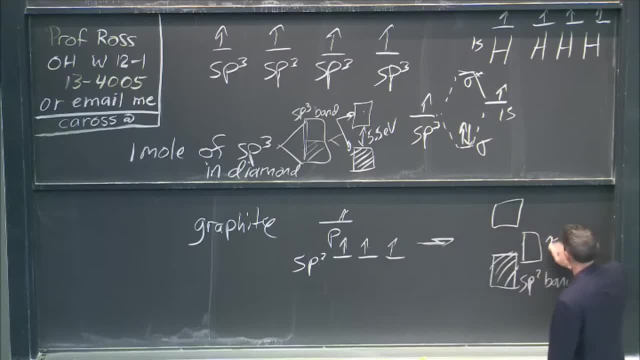 But now I've got The PI bands that didn't split. graphene Graphite is a metal. You can understand it by by looking at the bands of these materials. Now again, let me emphasize: I am not going to ask you to know when something splits, like this or not. 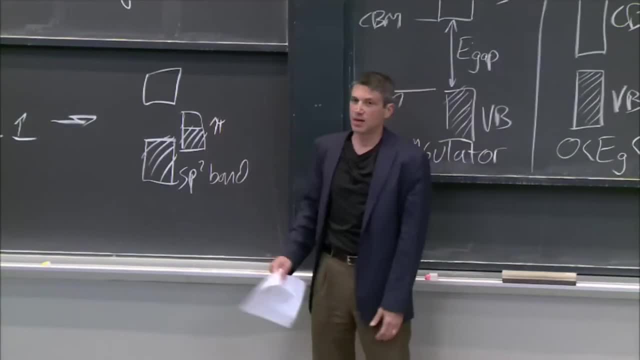 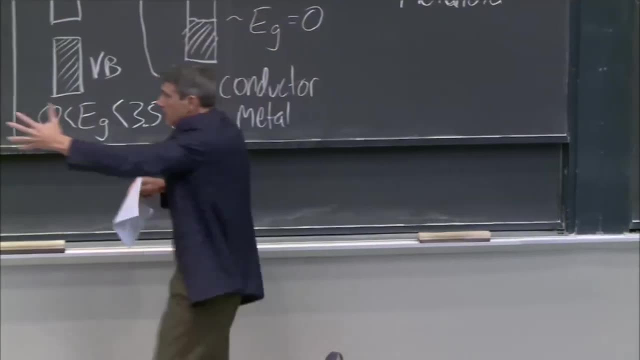 Why didn't the PI band split into two, like these did? When do two? when does an S and a P become a single band, versus an S band separated by a P? I'm not going to ask you to know that, But I wanted you to see it. 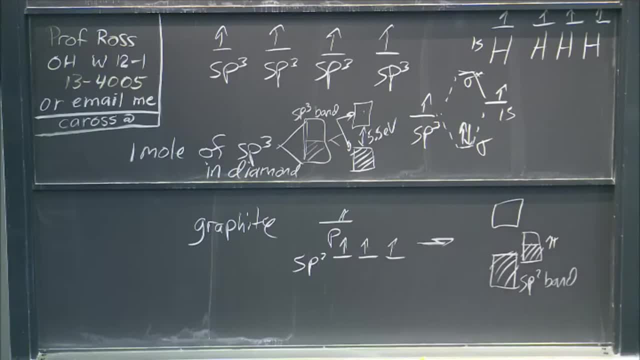 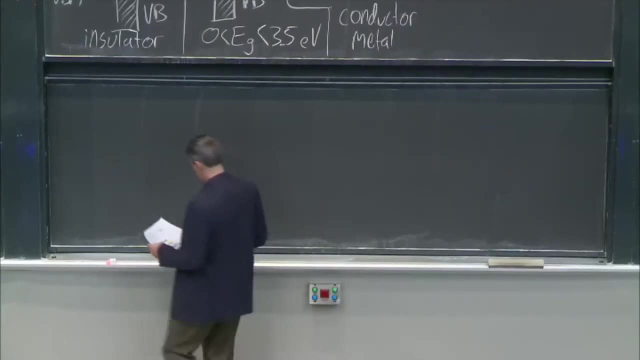 It doesn't just depend on the initial states. It depends on the structure of those atoms, Depends on how those atoms are bonded together. Good, OK, now what about this semiconductor? What about this semiconductor? Well, if we take a semiconductor and we look at it- I told you this on Monday. 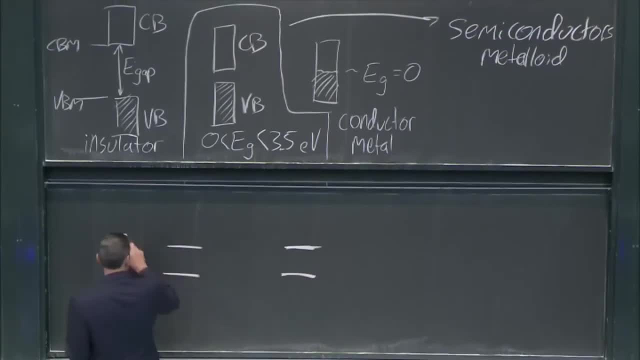 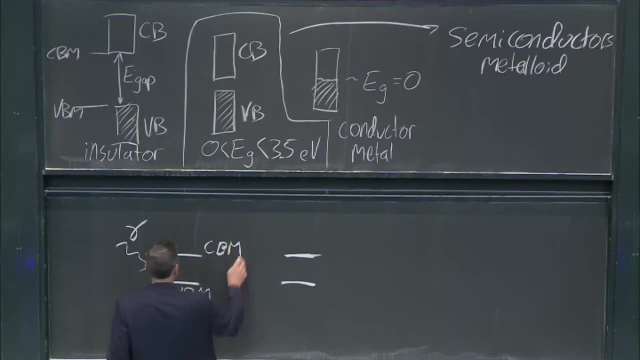 There are two things that you can do Right in your goodie bag. especially one is you can take an electron and you can shine the light on it and it's going to excite this electron up, just like in the Bohr atom Right. 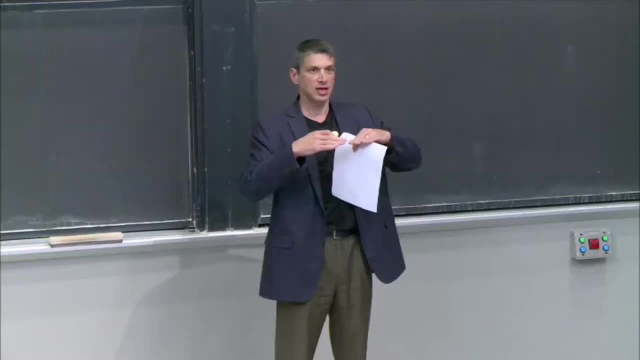 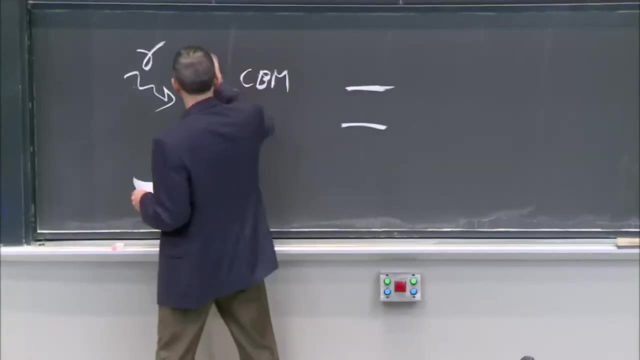 You can absorb photons if the photon energy is the energy between one state and another. We did a lot of this earlier. But see, in a semiconductor, Remember, I've got an almost infinite number. I've got a number of states here. 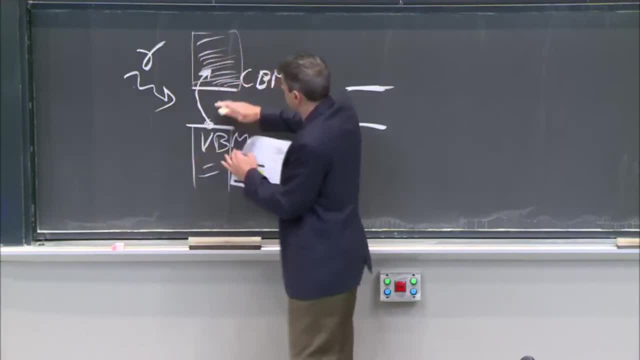 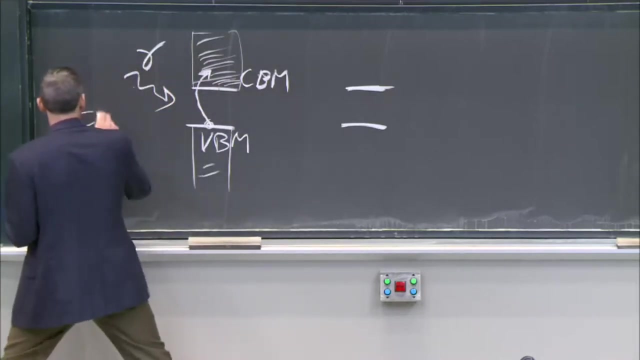 And so what I need is for that photon there's not an exact value, here There's a continuum, But here it's forbidden. just like in the Bohr atom, There's no states, There's no electron. So here the energy of the photon absorbed, let's write this out- absorbed. 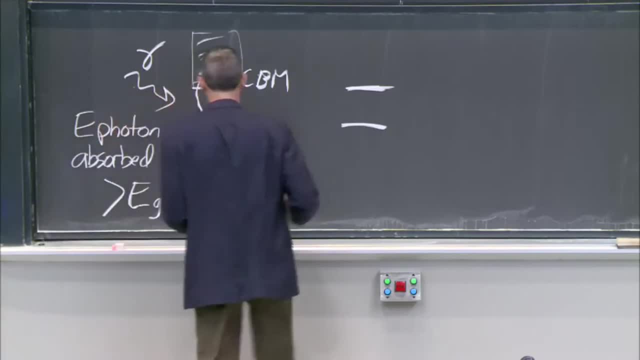 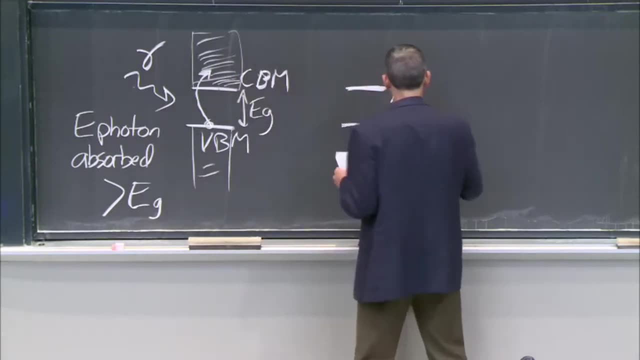 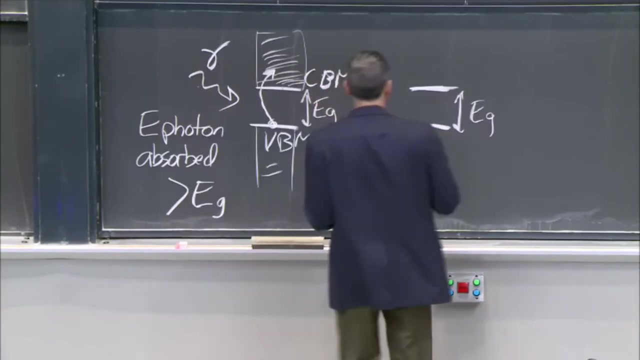 has to be greater than the energy of the gap. This is the energy of the gap. This is the energy of the gap. Now, by the same token, I can take the same semiconductor and run it the other way. I can put a current on it and feed electrons. 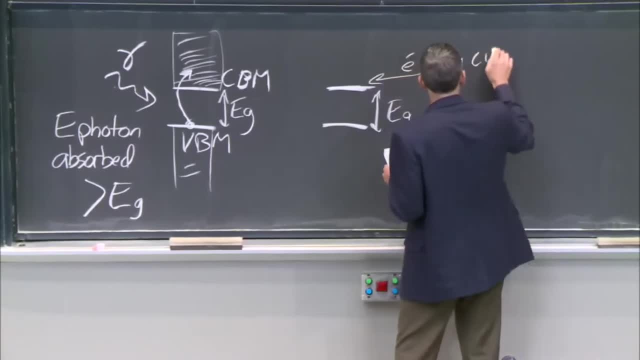 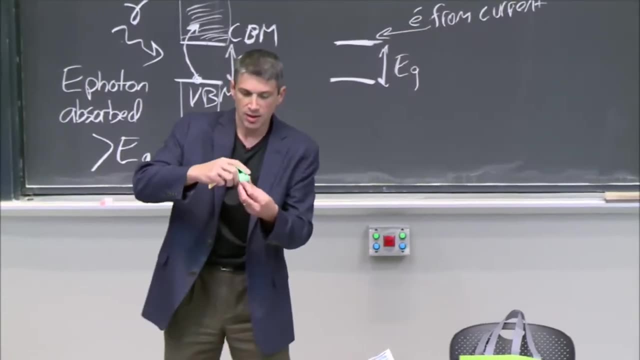 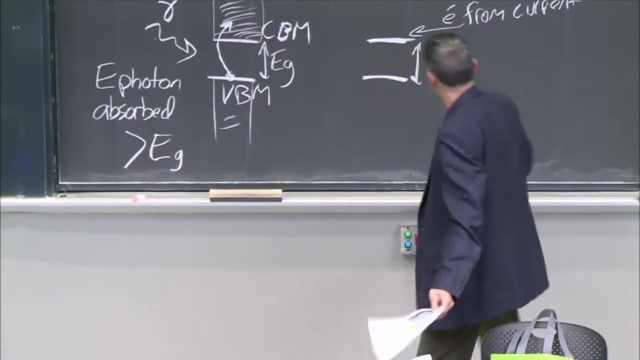 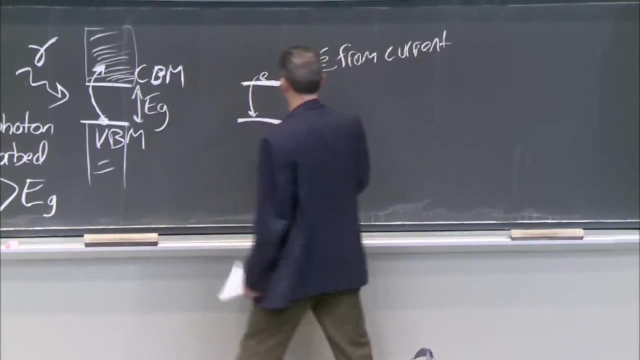 Electrons from current, So I can attach it to a battery. and there you go. This is a semiconductor Where I'm literally all I'm doing is I'm feeding electrons into its conduction band, But now, when those electrons fall down into the valence band, 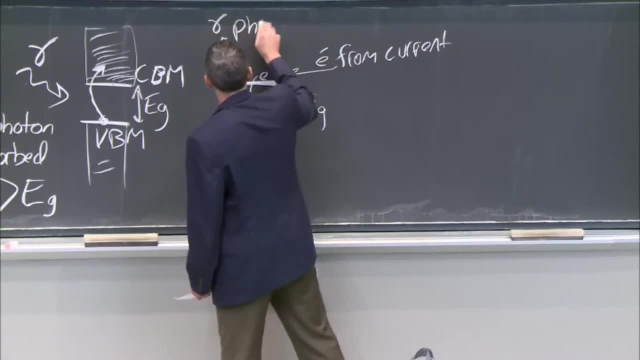 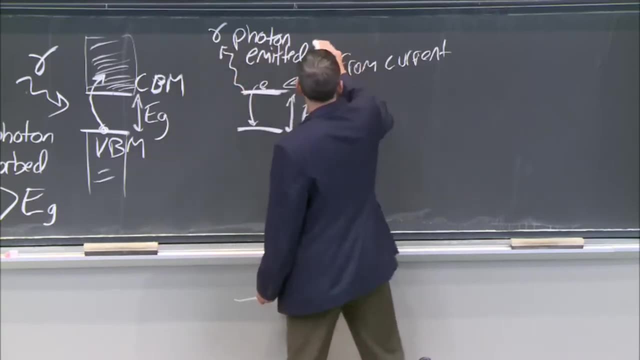 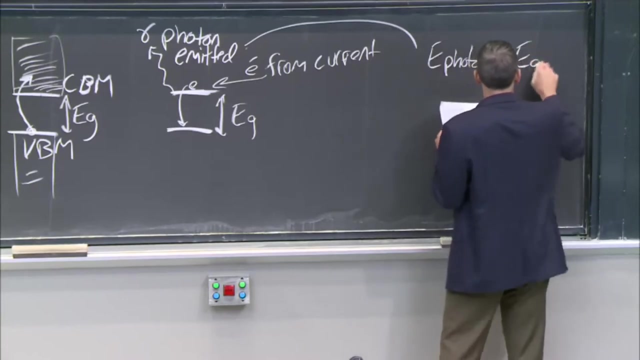 they emit a photon. Photon emitted And just so I have room with energy of the photon emitted is going to be exactly equal. So the energy of the gap. You can see that because these electrons, I might inject them into the conduction band anywhere. 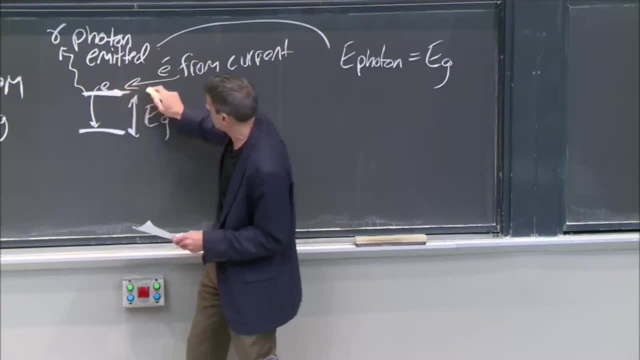 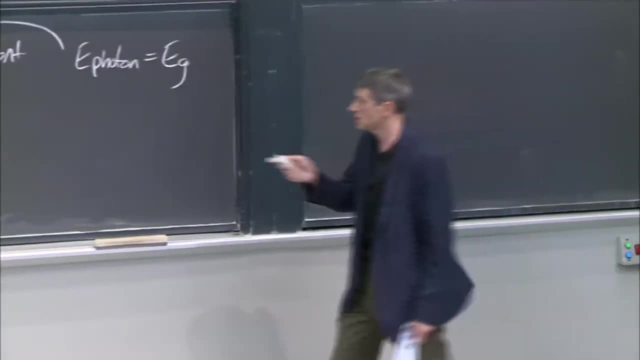 but they're going to wind up very, very, very quickly going to this minimum conduction band state. And that gets me to another important point, which is on the absorption side. I can overshoot this. Like I said, I can absorb higher than the gap. 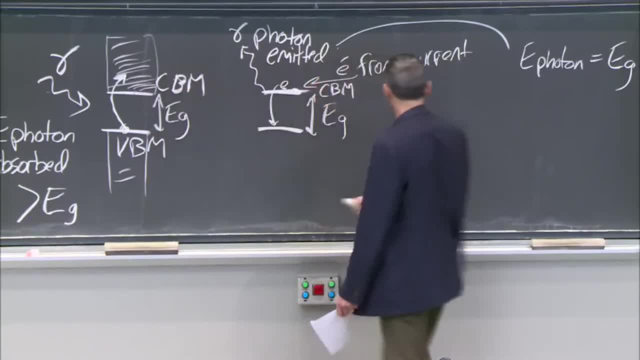 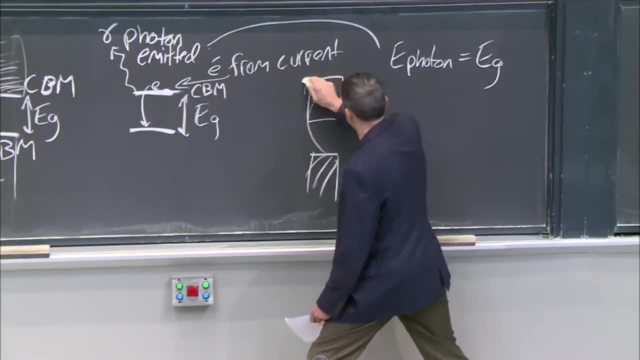 I can't absorb lower, But I can absorb higher And if I do, if I absorb higher than the gap, I can absorb lower. So let's say this is my state. Then that electron, so if my photon comes in and it kicks an electron up really high, 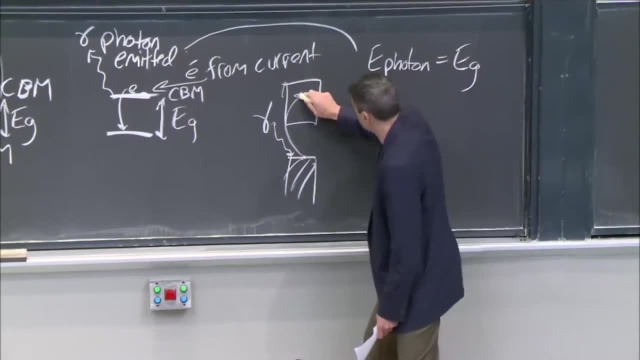 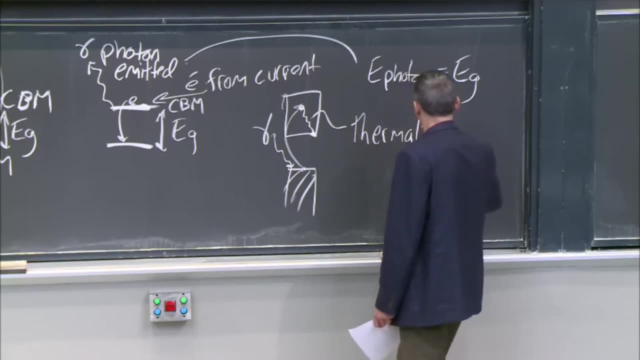 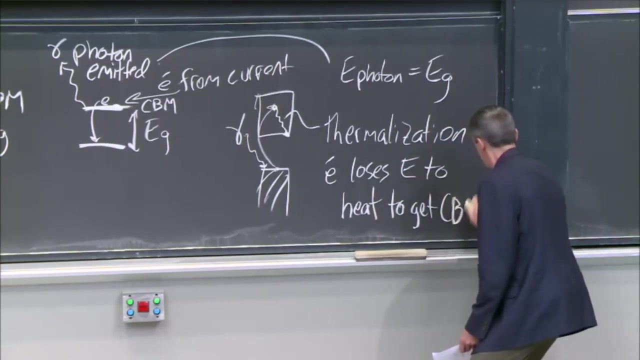 it's a high energy photon, then that electron very quickly will go back down And that's called thermalization. So what happens is that electron loses energy to heat And that electron loses energy to get to the CBM. OK, We'll come back to this later. 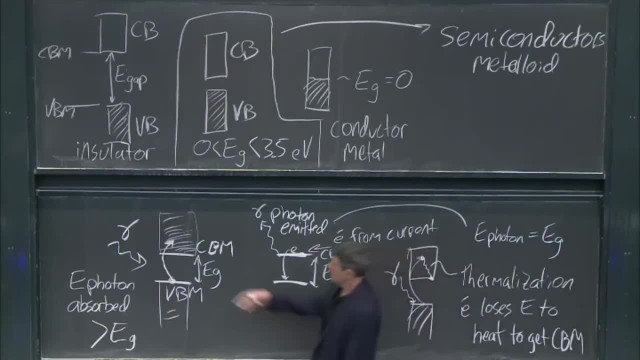 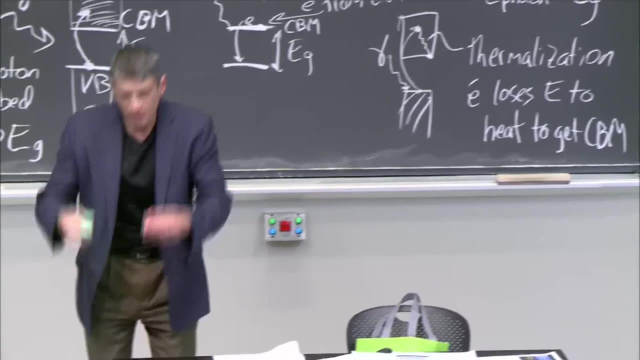 That's thermalization, So the electron can be kicked up by light to any level, But it's going to very, very quickly go to the CBM. That's why, when I inject it, that's why these are the same color, You know these are high quality LEDs, clearly. 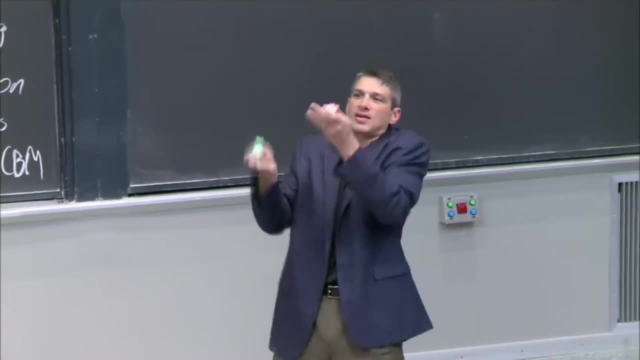 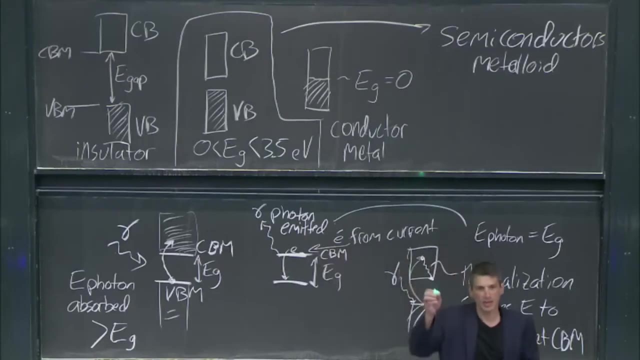 Well, they work. That's a good thing, And you know so. the batteries might be slightly different, The currents might be different a little bit. I might be injecting electrons at different parts of these conduction bands, But this is always green and this is always red. 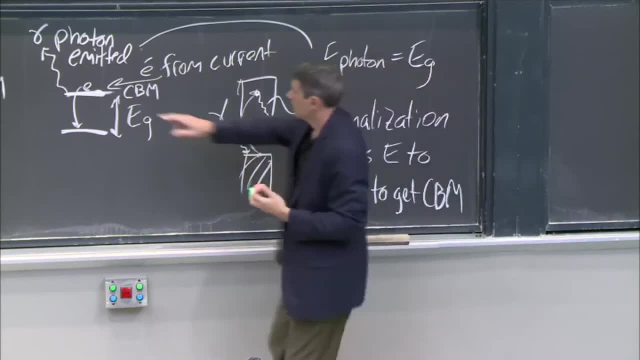 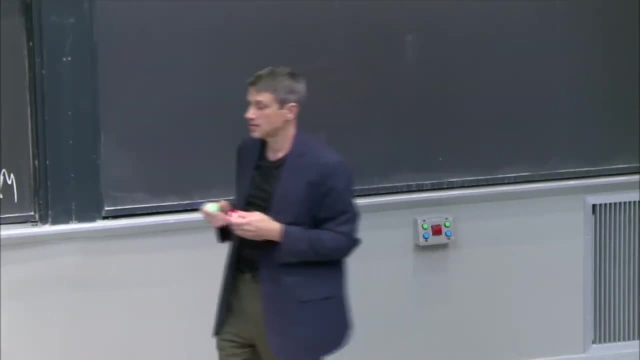 And that's because those electrons very quickly get down to the CBM and the VBM, And the CBM and the VBM are determined by the semiconductor inside, by the semiconductor inside. OK, Well, you've also got you know. so this: 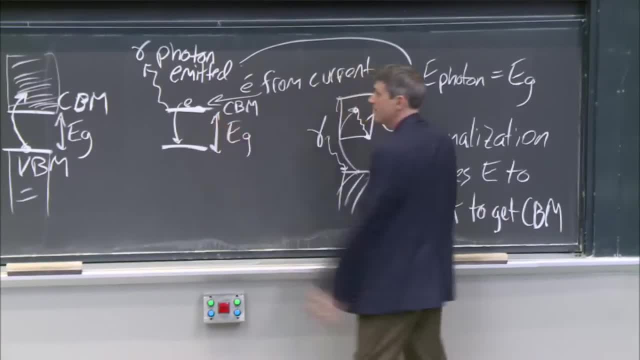 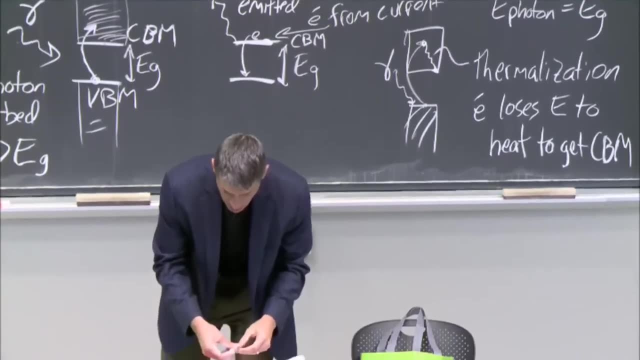 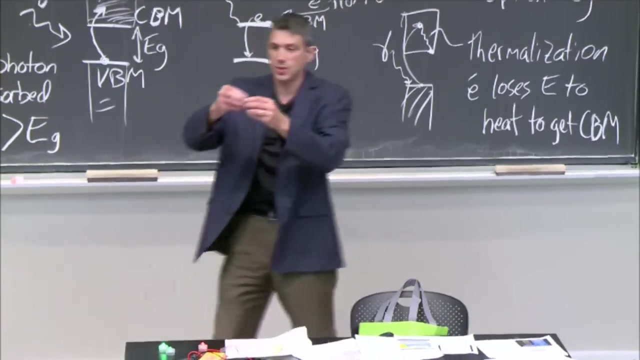 is a photon emitter right here. I've made a light emitter right, But I've also got a detector, which is what I said on Monday. So now I take an LED and I hold it and I Gesundheit. this is what's inside of the emitter. 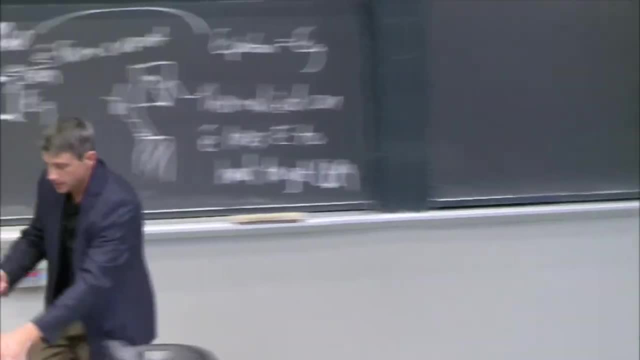 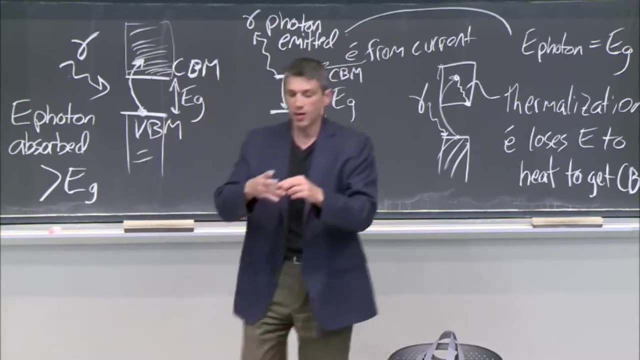 It's the same thing, It's a semiconductor, But these two semiconductors have different band gaps. That's why the light is different. They have different band gaps. Now I've got one with some band gap and I hook it up to my voltmeter and I just look. 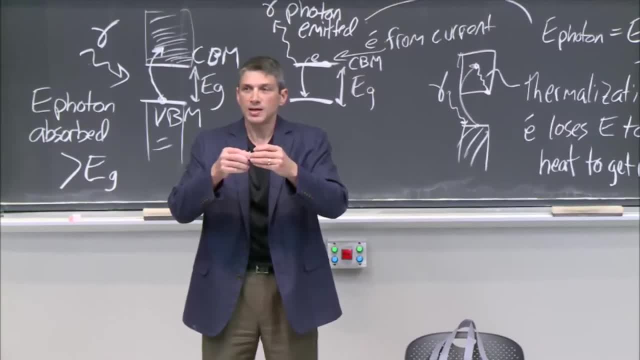 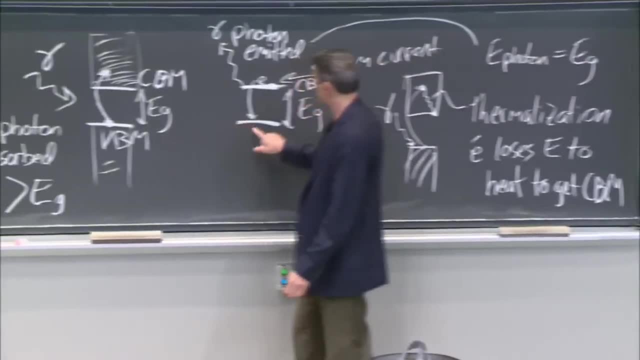 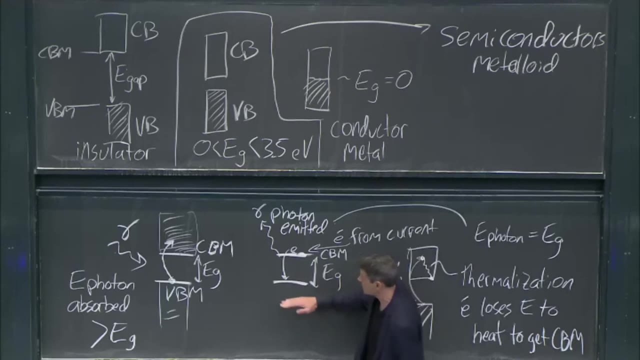 Is there a current? Is there a current or not? If this thing conducts through it, it means that electrons have been promoted from here to here, And that's something we're going to talk about today. Electrons cannot move around easily if they're in the valence band. 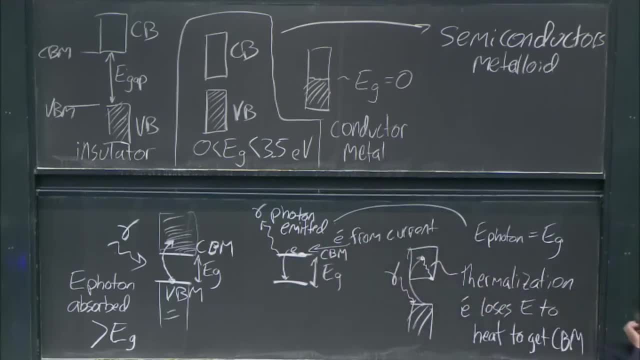 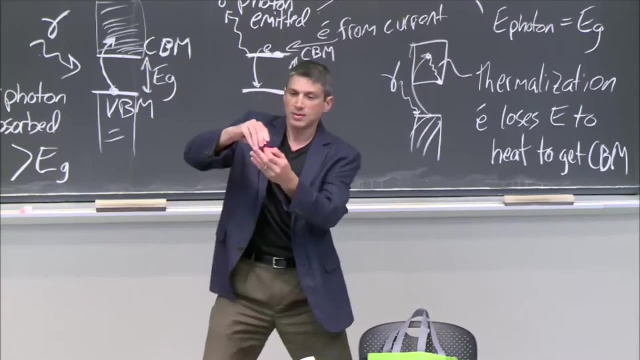 But once they're in that conduction band, they're free. How do I get them there? Well, you've got power. Shine red light on it. Does it conduct? Check the voltmeter right. I'm literally holding two semiconductors. 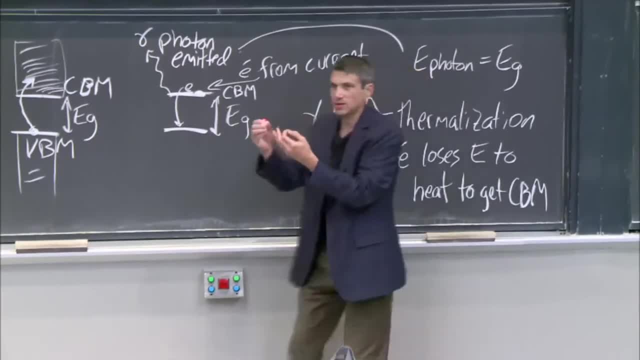 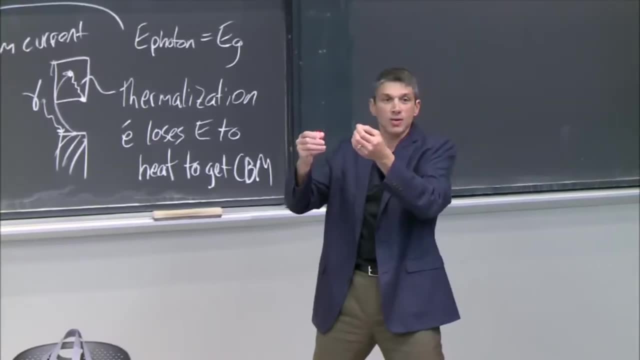 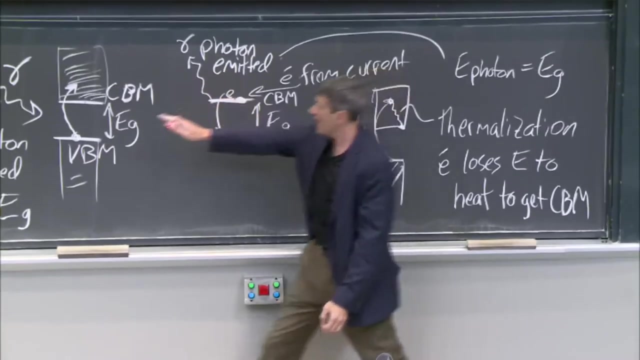 and doing these two processes right here in each hand. It's a power that I have. I have semiconductor making light, semiconductor absorbing light, or maybe not, If I shine red on this and I get no current. well, it means that the energy of the photon from a red light 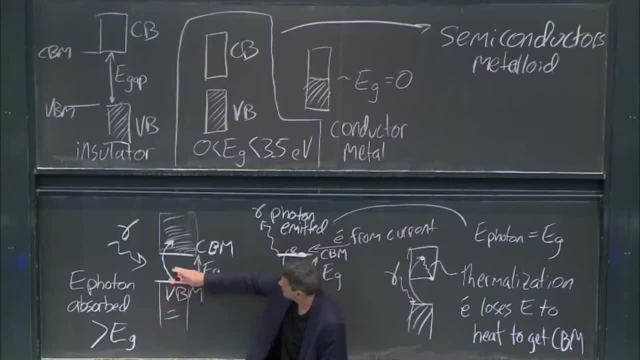 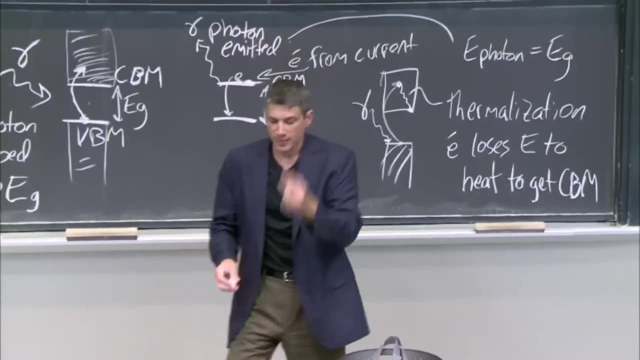 source is too low. Maybe it's able to excite it up to here, but not up to here, given whatever the gap in here is. You see that. So the semiconductor has a power. It has this powerful. Maybe I take a different semiconductor. 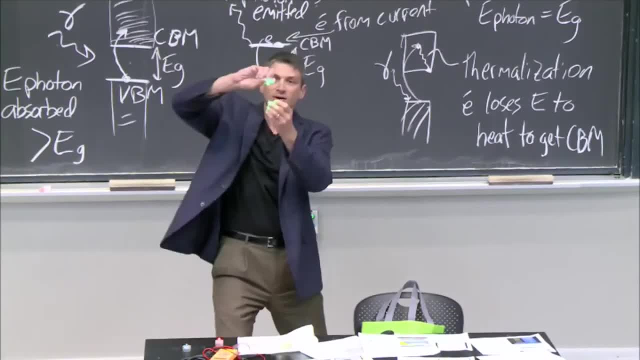 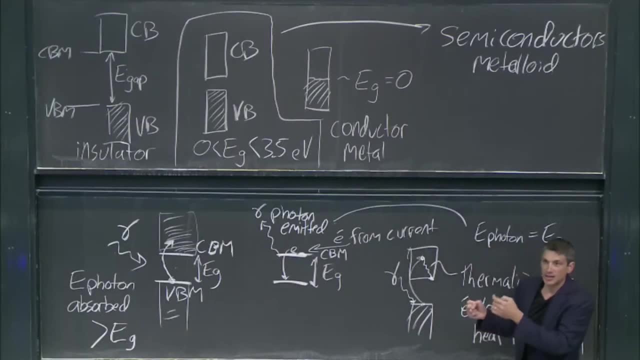 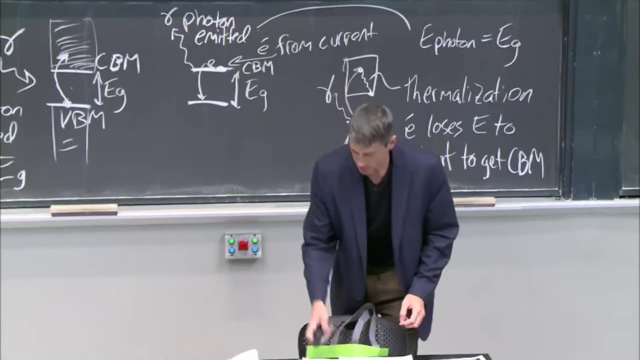 and red excites it Or maybe it doesn't, so I go to a higher energy photon right With this goodie bag. you're touching and feeling semiconductor physics and chemistry, and chemistry, because band gaps in materials are rare. You see, if you look at the periodic table, 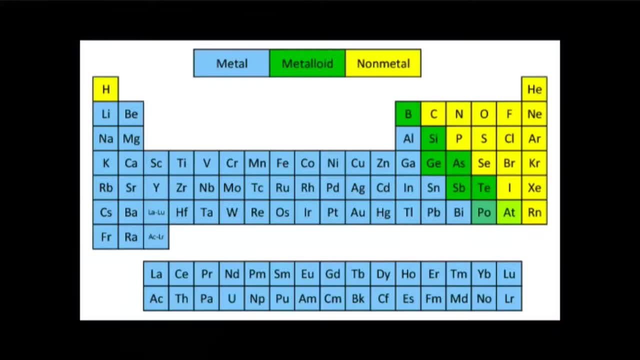 and you classify it by metals, metals and nonmetals. so insulators, conductors, and then these weird things in between. there aren't that many of them. There aren't that many of them, But, as you can see, these are really, really important. 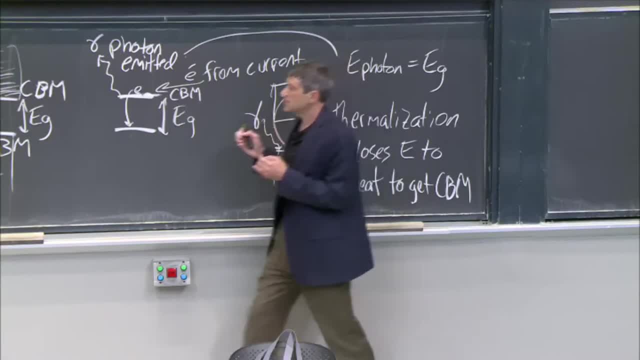 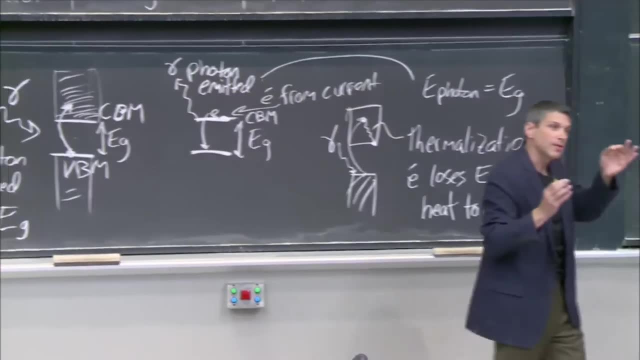 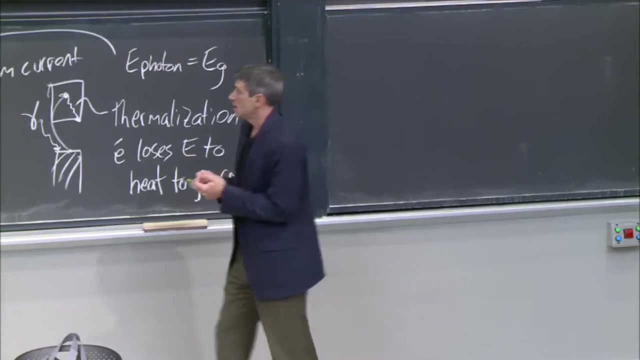 technological materials. Why? Because this is visible light. The semiconductor range here is in the range of light. we care about visible UV. So I've got an electronic material where the electrons in it can interact with currents- small currents even- and wavelengths of light. 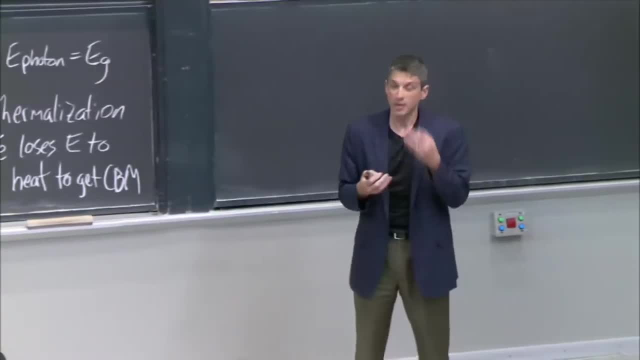 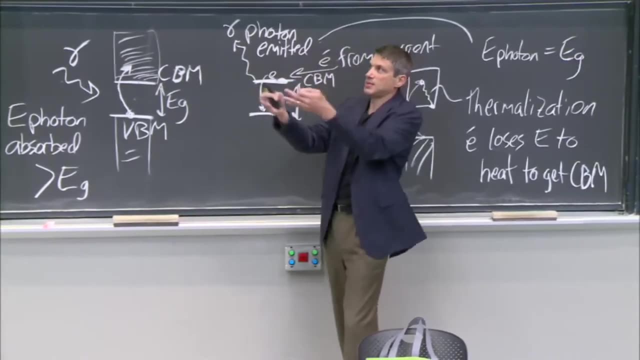 that are things we can see. You can imagine how important this could be, for example, for making LEDs, But I need a lot more flexibility in my material set, and that's where chemistry comes in. So this is one why this matters for today. 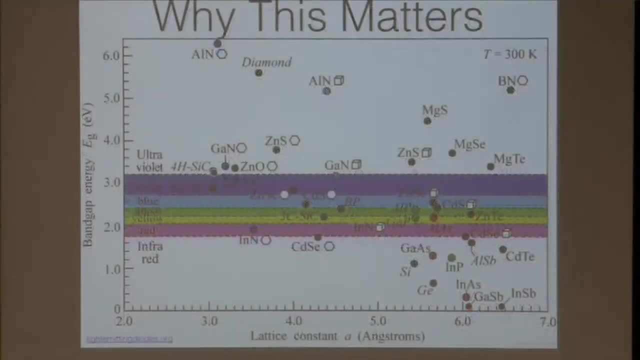 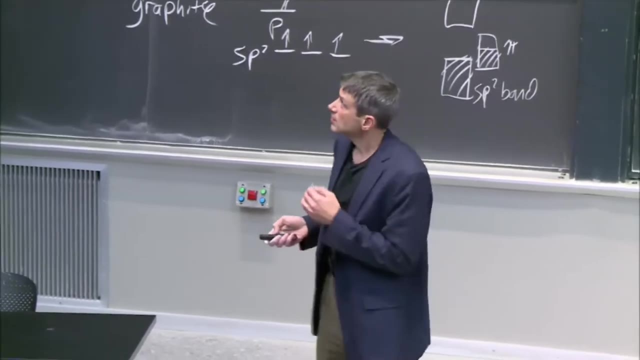 So, look, I mentioned that getting red was hard back in the day for color TV because the red phosphors were difficult to make. For LEDs, it was blue And in fact there was a lot of work around gallium nitride. 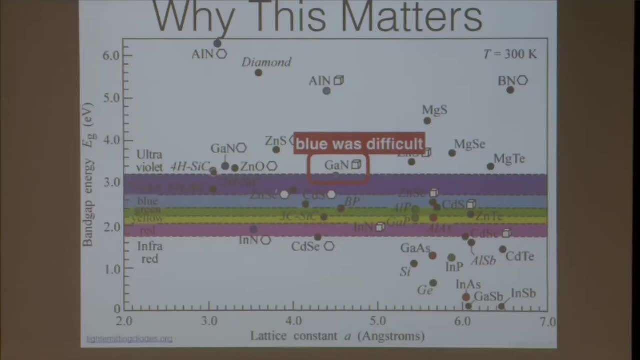 Here's gallium nitride in one structure. Oh, notice this, There's gallium nitride. It's not on here, Darn it. Gallium nitride in other structures have different gaps. Oh, there it is, There's one. 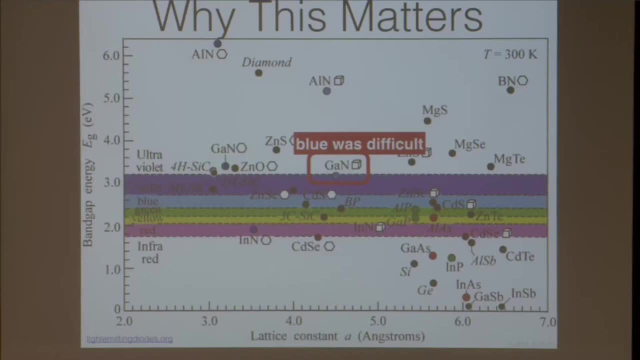 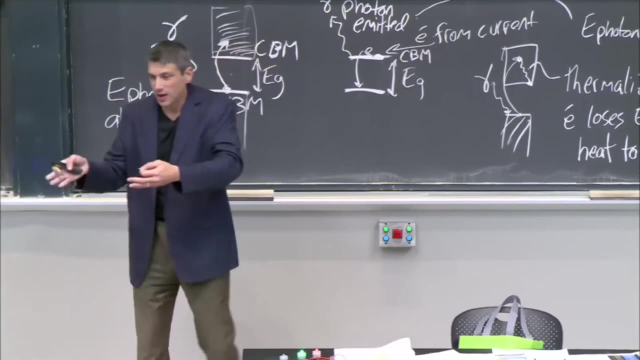 But the point was they wanted blue. They wanted blue and they needed to make a material that was both cheap to make and lasted, so it didn't degrade and gave you blue light. And that was really hard And that's what the Nobel Prize was given for in 2014.. Because without blue you can't make white light right. So there's all sorts of technologies you simply can't go into with LEDs until you get blue. How did it happen? It happened because of chemistry, Because people figured out how to take one element. 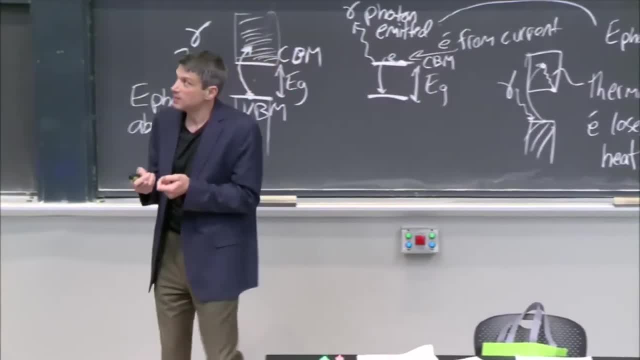 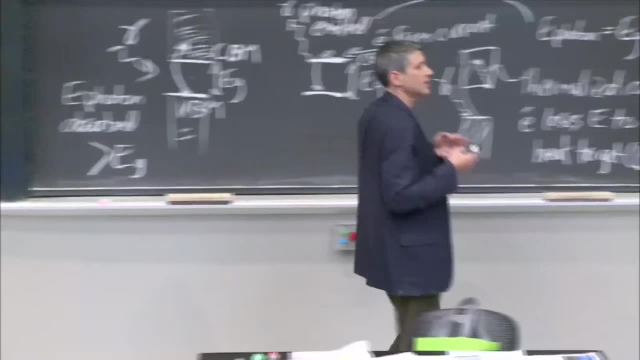 and another element and then maybe alloy them together. Maybe you take gallium nitride and you alloy a little bit of aluminum in here And now, all of a sudden, that means mixing in right. Now, all of a sudden you've got a. 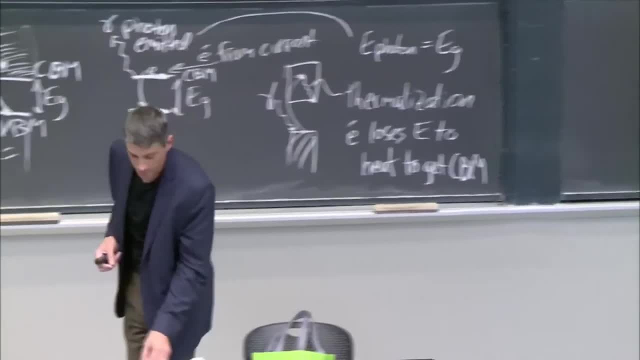 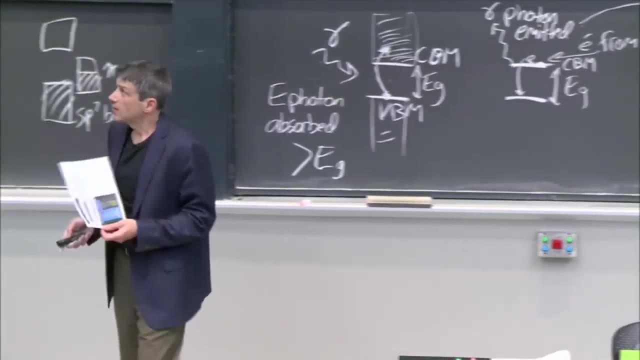 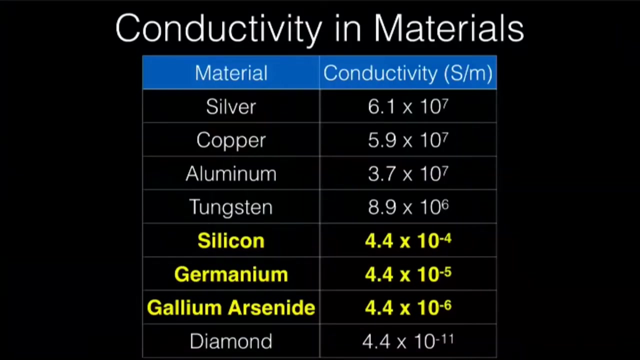 different band gap. OK, Band gap engineering is really the centerpiece of the semiconductor revolution. Now the conductivity. We've been talking about conductivity And we'll talk about metals on Friday. OK, Here we are. Insulator's really low. 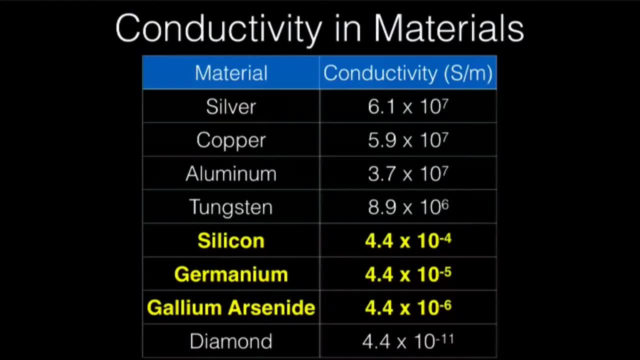 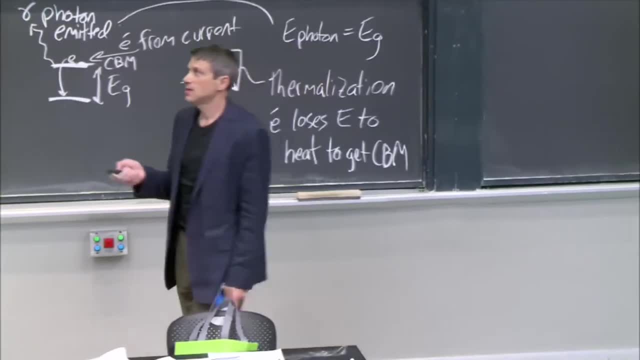 Least conducting: 10 to the minus 25th. Hook your voltmeter up to Teflon, 10 to the minus Wood right Low conducting materials. But we're interested in these And look, these are kind of in between. 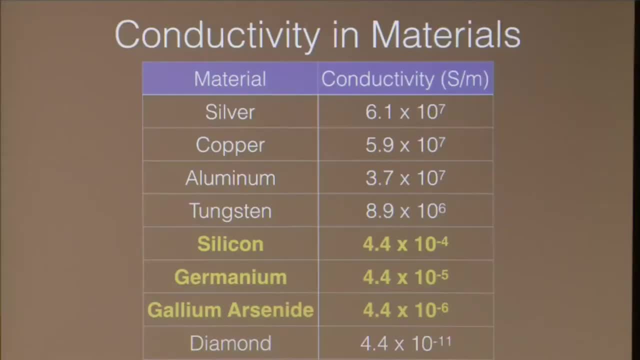 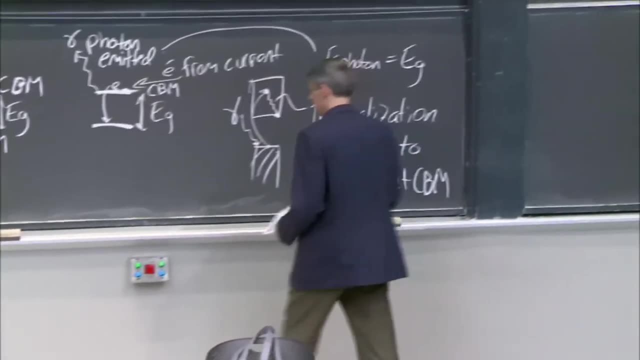 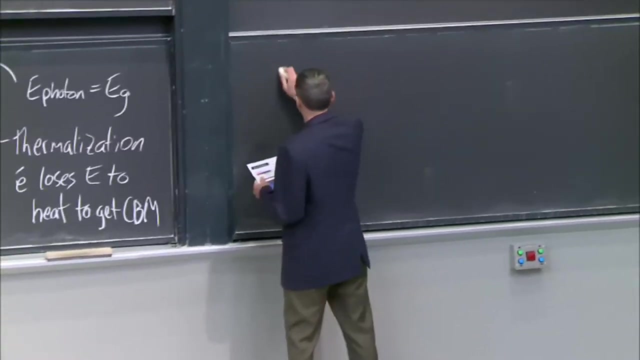 They're not very good conductors. That's why they're called semiconductors, right, But the fact of the matter goes back to what I've been saying- And this is the next point I want to talk about- which is I cannot have. 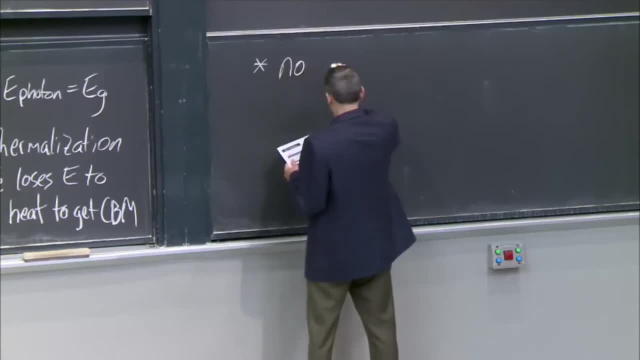 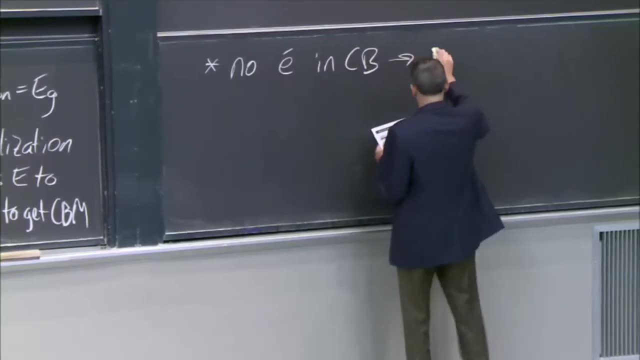 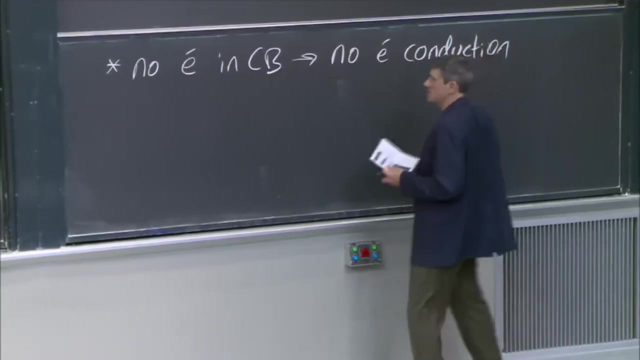 So in a semiconductor there's no electrons. If there's no electrons In the conduction band, then there's no electron conduction. Now, I've said this before. I said this on Monday, I said it already, Why not? 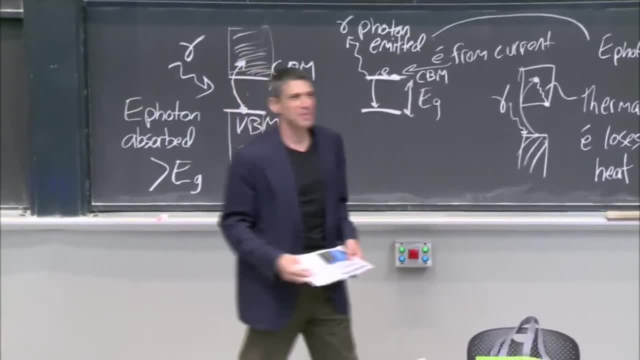 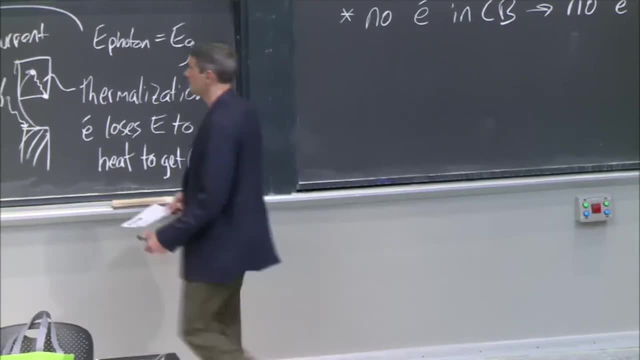 On Monday I said: well, the electrons are stuck. What does that mean? they're stuck, Stuck in the bonds, stuck in the anti-bonds, They're stuck in states. The point is here that here you've got these. 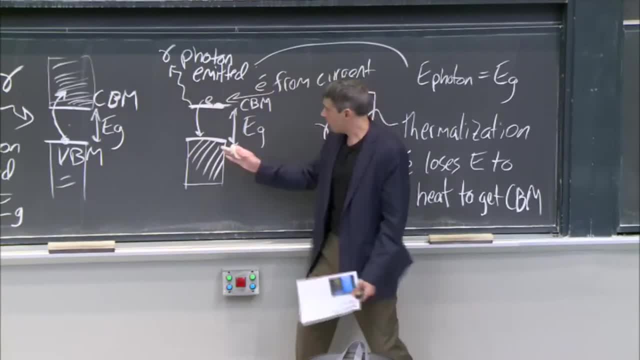 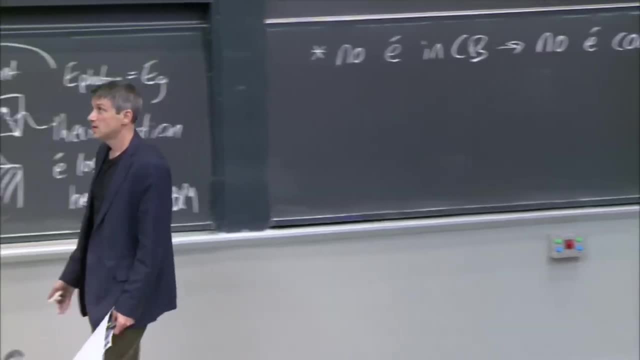 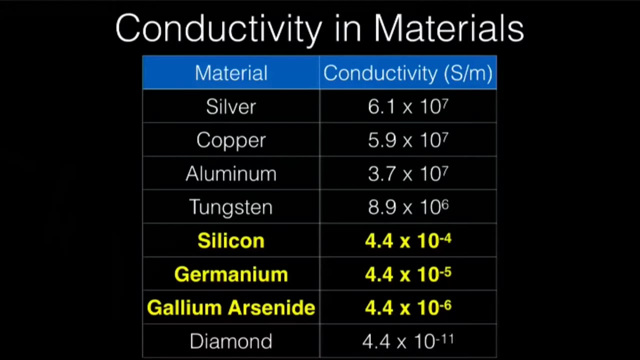 This valence band is filled. Now, if I want an electron to move through a material- which is what conductivity is, after all, By the way, Siemens conductance 1 over ohms- If I want electrons to move in a material, they need freedom. 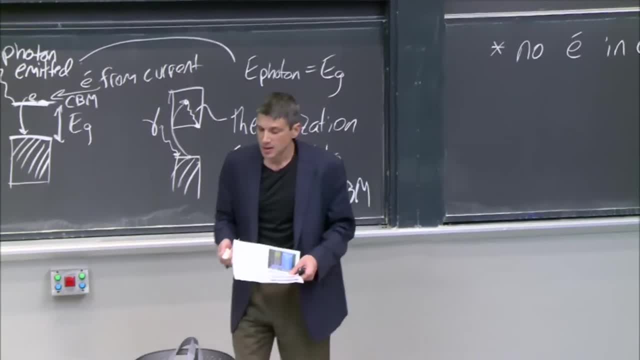 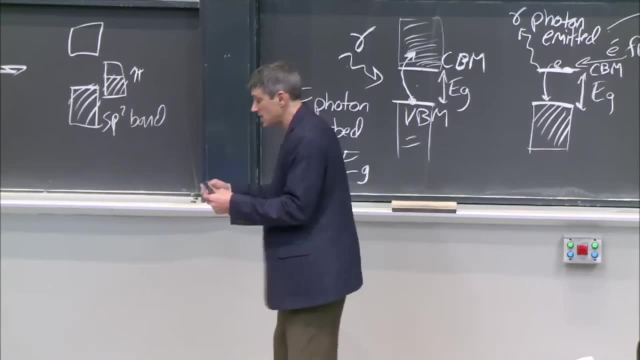 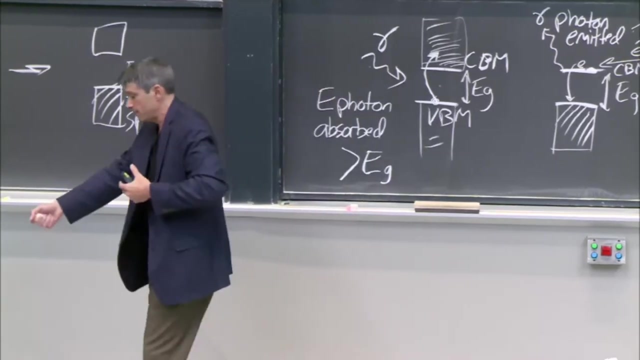 They need freedom. What does that mean? Well, it means that I'm trying to move through this wire And for an electron freedom means I can go to any state that's nearby State, A wave function, A state of probability that I can move to. 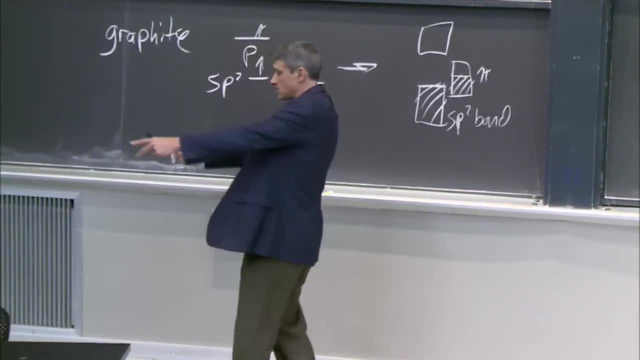 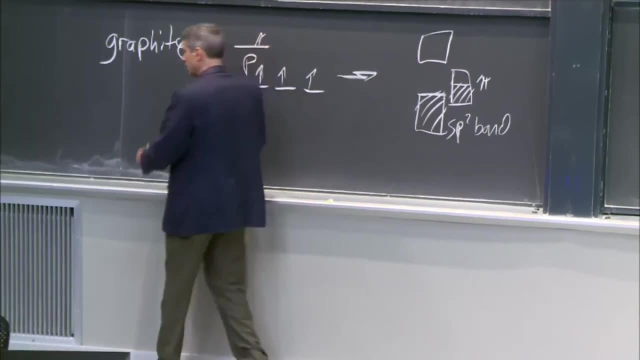 And then to that one, And then over here: Oh, there's something there I don't want to be in. I've got to go this way. That's a bad thing over there, It's scattering me. I'll go this way. 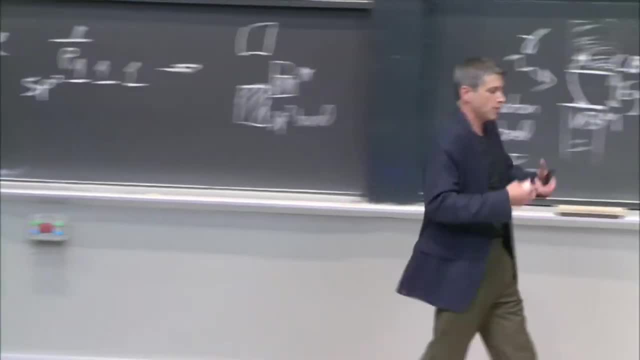 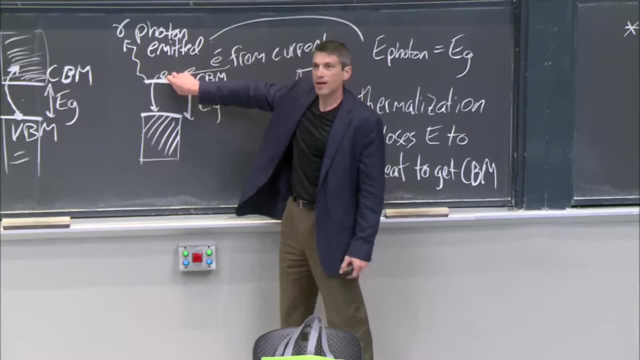 But if electrons don't have the ability to move into a free state, they're not going to conduct. That's why you've got to get the electron up here. Why? Because the conduction band. I shouldn't really fill this in. 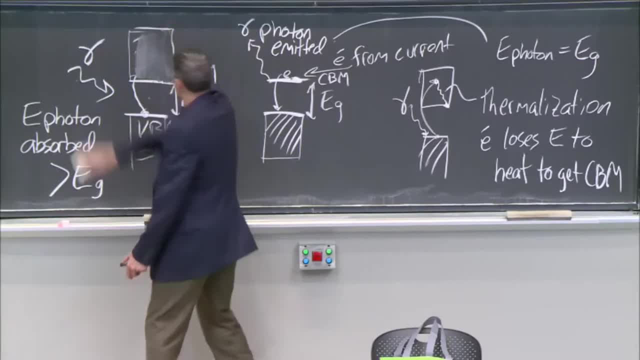 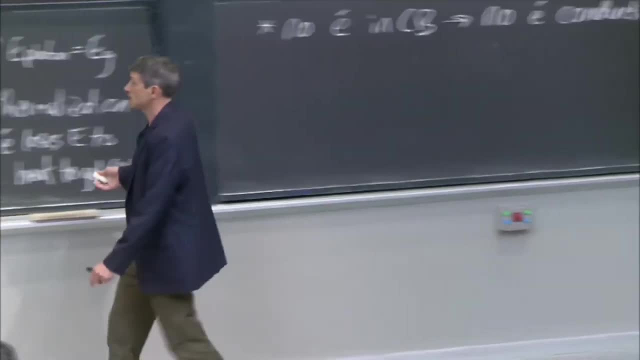 I'm just showing you empty states there. The conduction band has 10 to the 24th states: Freedom, Freedom. So as soon as an electron gets up there, it's like, oh, I can go anywhere I want I can be there. 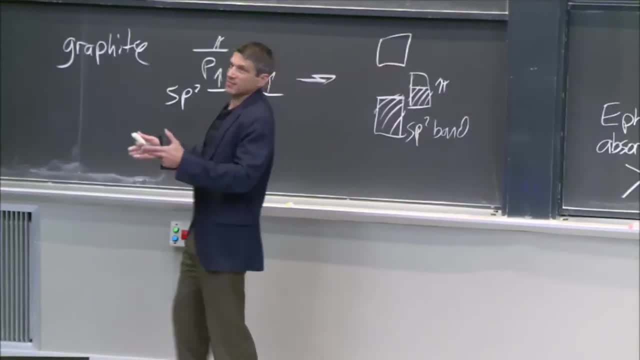 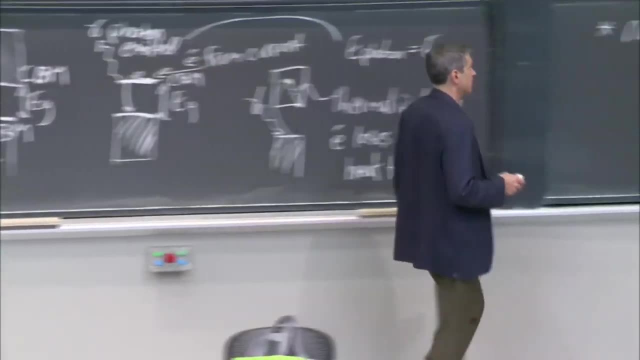 I can be there, I can move in response to this field that's pushing at me, I can conduct. I can't do that unless I have conduction, Unless I get electrons into the conduction band. But this is OK Now, this is why you can see right there. 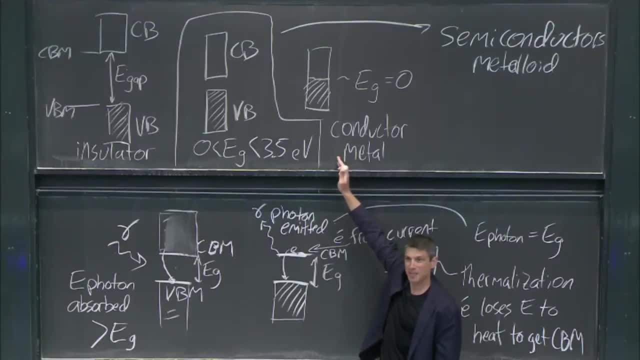 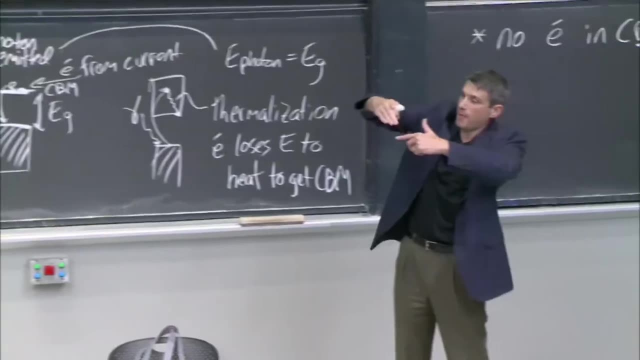 metals are clearly good conductors, based on our band picture, Because those electrons near that line, there you fill them up and they're halfway in a band. But right up above there, almost infinitesimally small energy away, is an empty state and another empty state. 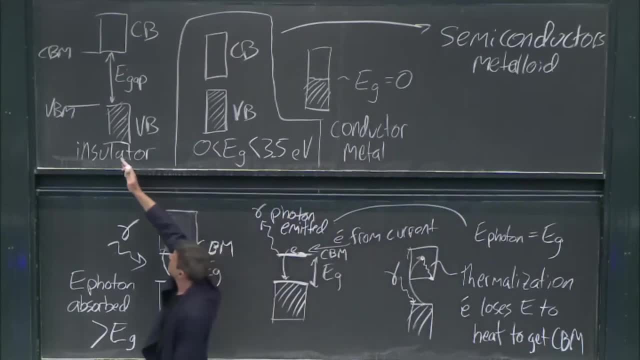 So that's why these ones- you can see it's going to be hard. I'm going to have to shine really high energy light to even get, or really high temperatures. But again, semiconductors are special because their gaps are right in that range. 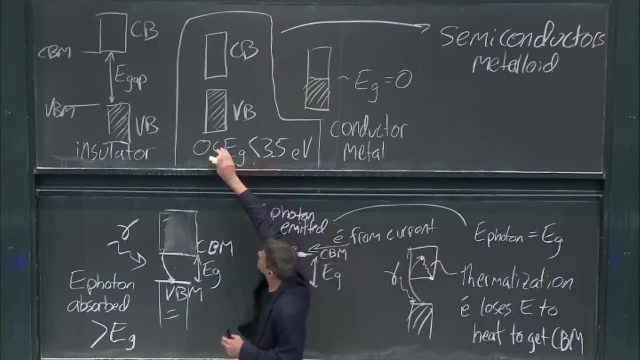 where I can get electrons to go from the valence band to the conduction band in different ways, And there's two different ways that I want to talk about Now. the first way is simply with heat, And this is why I mentioned this on Monday. 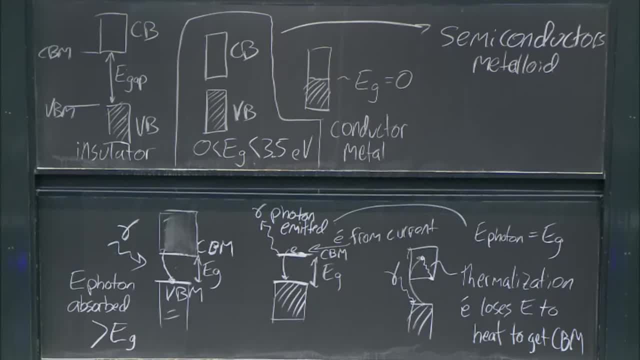 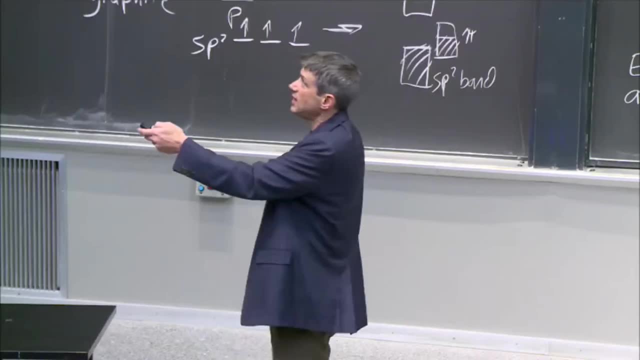 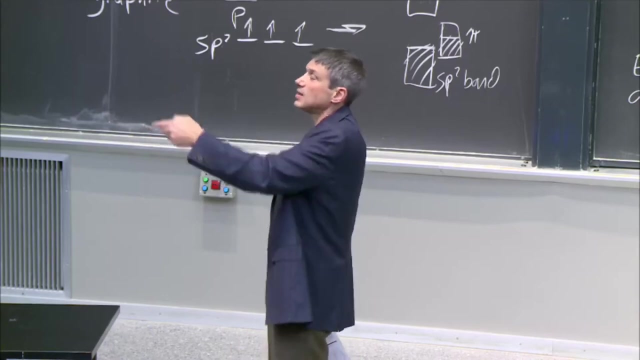 Actually, no matter what, there's some probability for an electron to have a high enough thermal energy. Yeah, Electrons get hot too right? Everybody feels the heat, And so that thermal energy can be enough to get the electron to knock it up above. 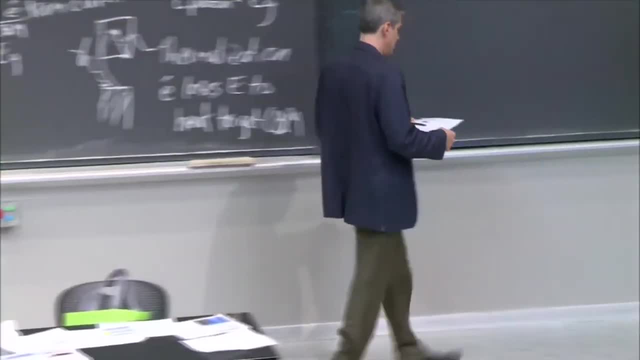 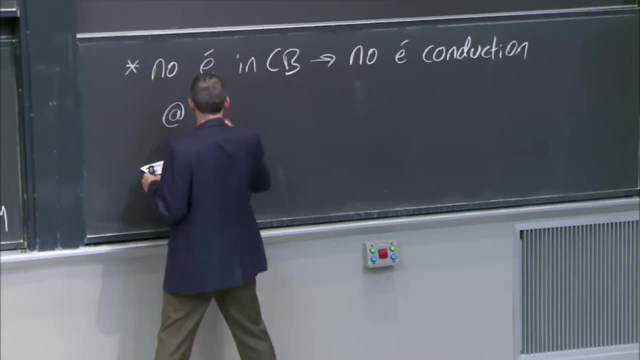 to knock it up above. So with thermal energy you can get, let's see, at room temperature for silicon. So this is the case of silicon which has a 1.1 electron volt gap, Silicon 1.1 electron volt band gap. 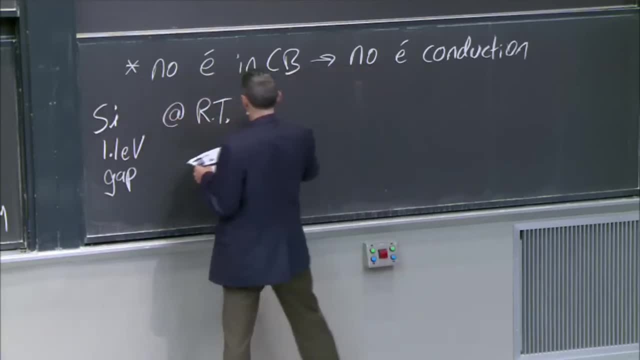 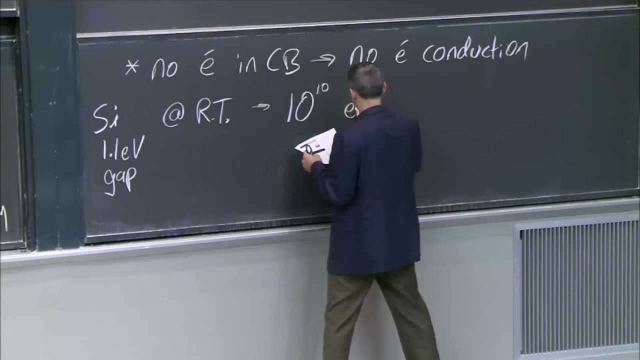 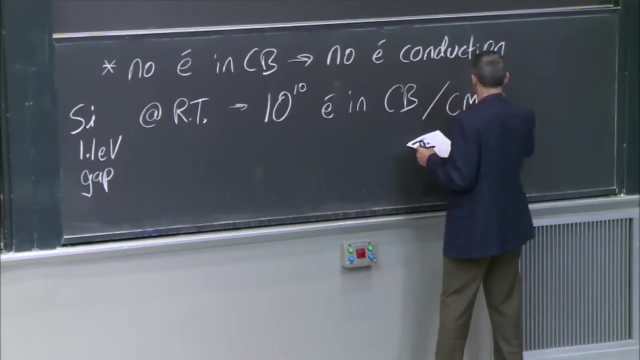 This is a really important semiconductor And for silicon at room temperature I got about 10 to the 10th electrons in the conduction band per centimeter cubed of material. This is how we think about it. We think about: how many of these do I have per volume? 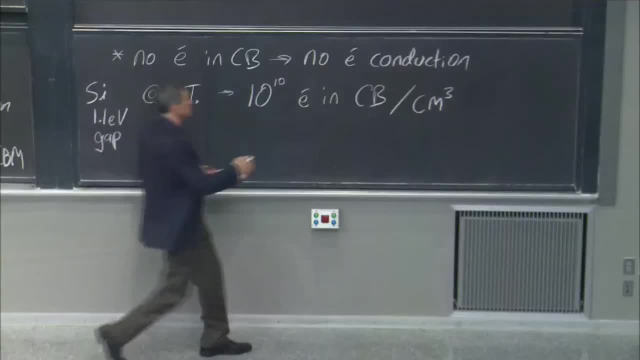 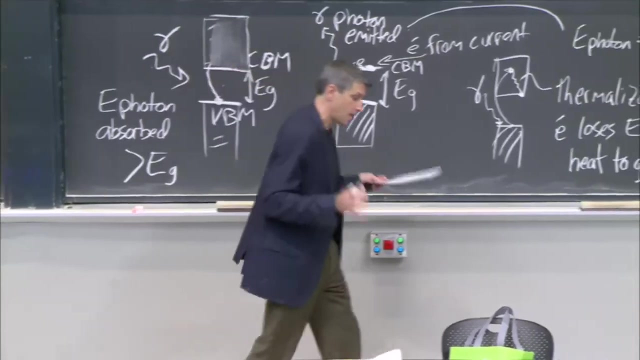 It's a good way to measure it. These are also an electron in a conduction band. also is called a carrier. So here's a for silicon at room temperature. I will have just because I can't help it, because there's that many are getting. 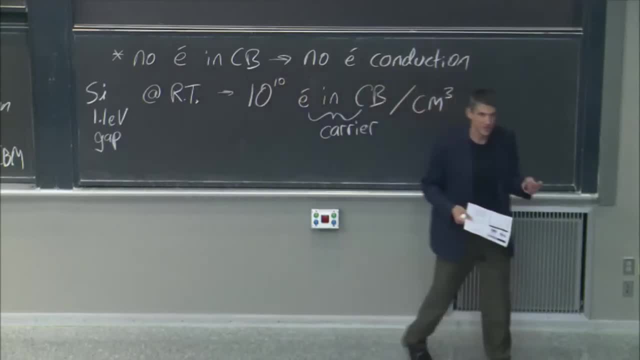 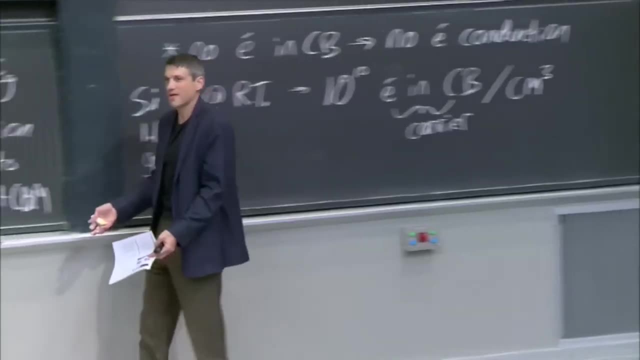 I'll have about 10 to the 10th carriers in the conduction band. Now the carrier is a carrier of electricity. That's why it's called a carrier, right, It carries electricity. So those are the ones that are carriers. 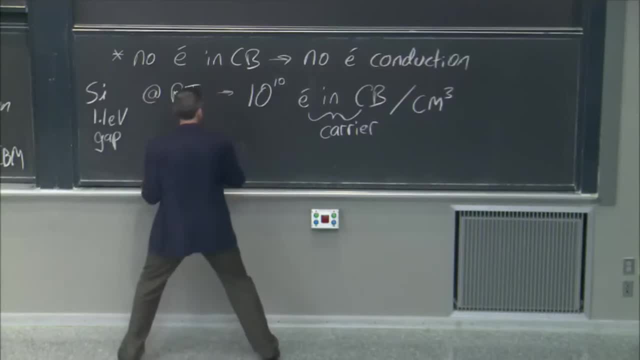 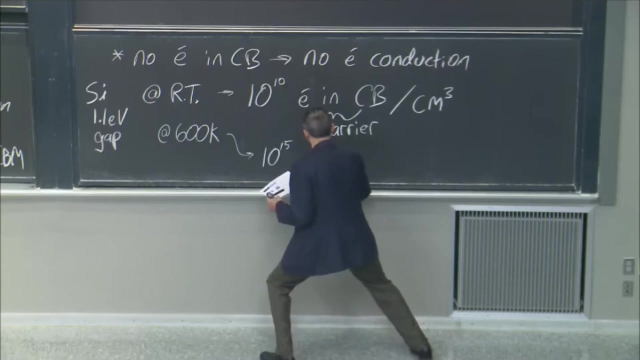 the ones that made it up, But if I go to 600, so now I'm going to go to 600. Kelvin- Oh, we only use Kelvin. Kelvin is the thermodynamic energy scale. temperature scale: 10 to the 15th. carriers per centimeter cubed. 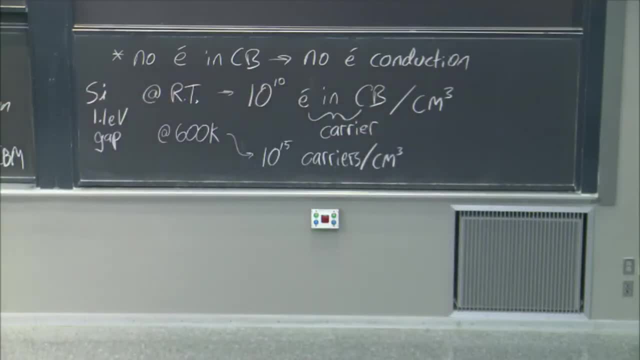 This seems like a big number, But is it a big number? It's a big number. What's a big number? we know and like in this class, The mole, So like roughly-ish. is this a big number, per centimeter cubed or not? 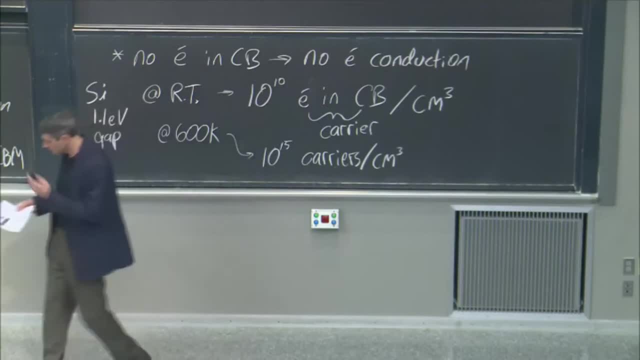 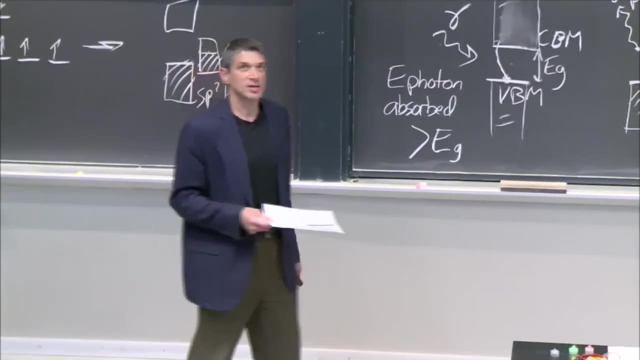 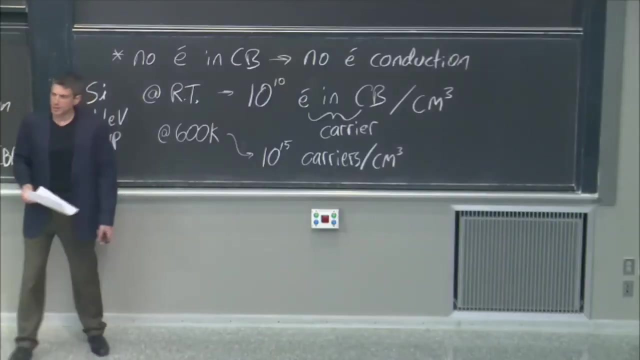 It's actually very small, right, But I need them to be there if I want better conductivity, If I want conduction in these semiconductors. I got to put electrons up in the conduction band. Remember that I just as an important point, 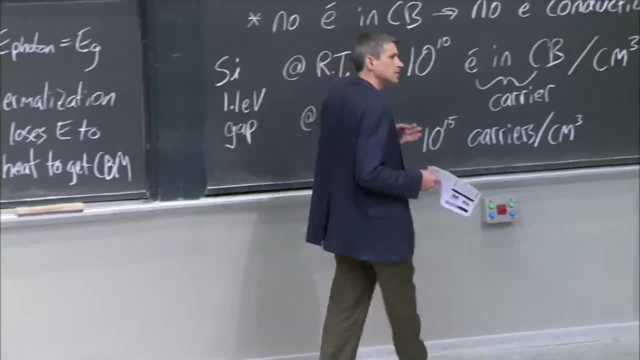 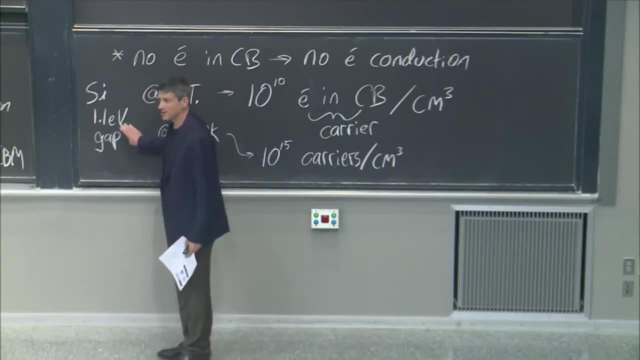 I mentioned the energy of room temperature. the thermal energy of room temperature, KBT, is about 0.025 electron volts. That seems way smaller than 1.1 eV It is, But that's because that's not what temperature really looks like. 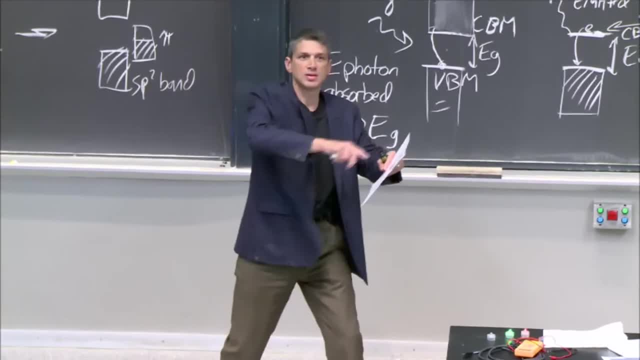 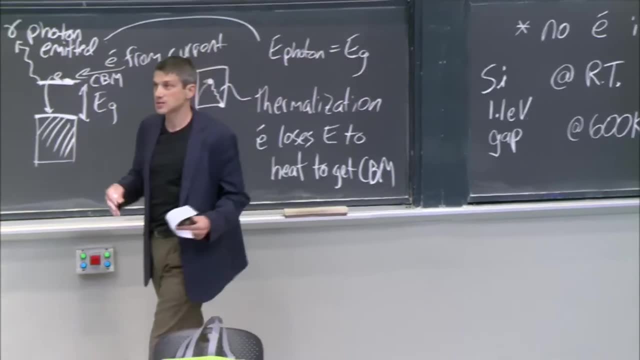 Temperature is a distribution is a distribution. Now, you don't need to know that for the band gaps. We're going to come back to distributions, Boltzmann distributions, when we talk about reactions, reaction kinetics Later. But that's why at room temperature the tails right. 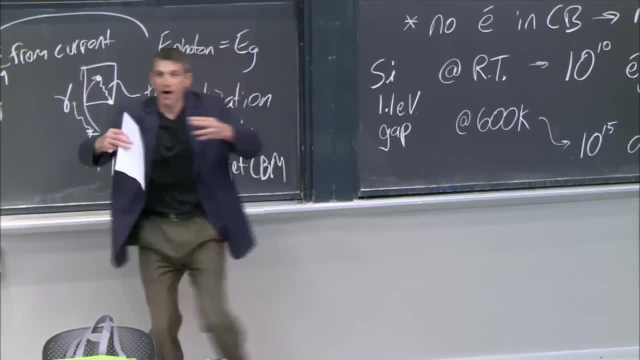 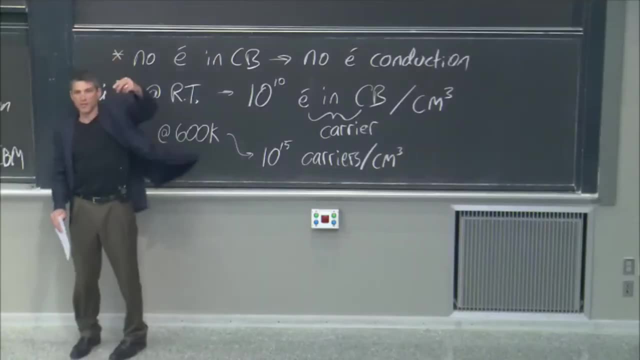 Hot means a range of energies, Hotter means a wider range of energies And it's those tails that have enough energy to get over the gap and into the conduction band. OK, It's those tails. That's why I got a little bit of electrons that get up there. 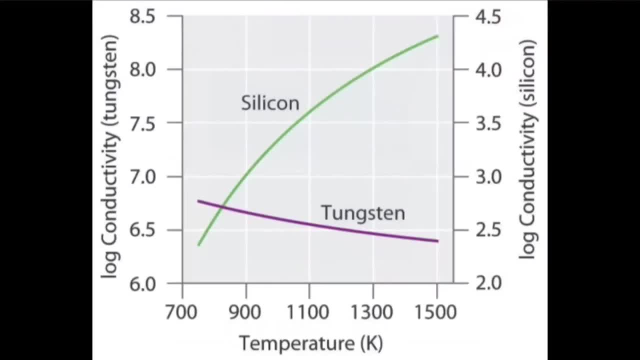 at room temperature. Now, if you look at a plot, here's a great one That way. there's the log conductivity of silicon- It's from Avril- And there's the log conductivity on this side of tungsten- That's a metal. 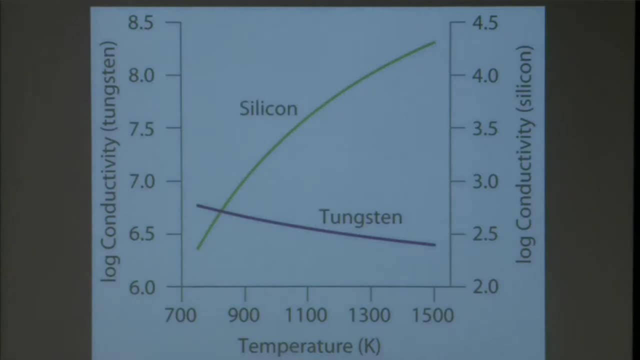 Totally different behavior. How is that possible? Well, we're going to explain the metal on Friday. Today, we're interested in this, This one. now we understand Thermal energy excites carriers into the place where they can be free and conduct right. 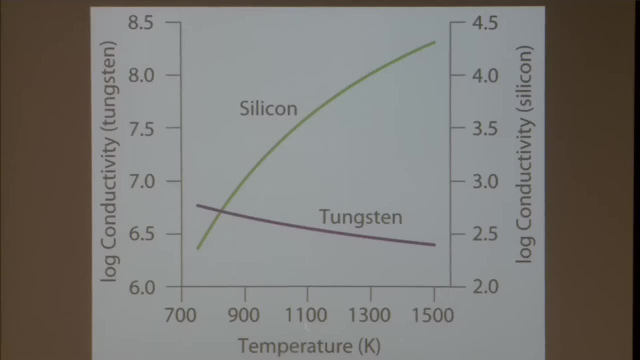 So as I increase the temperature, hotter and hotter. there's the temperature in Kelvin, right, I just gave you examples from down here, And now we're going higher and higher. I can get the conductivity up orders of magnitude higher for silicon. 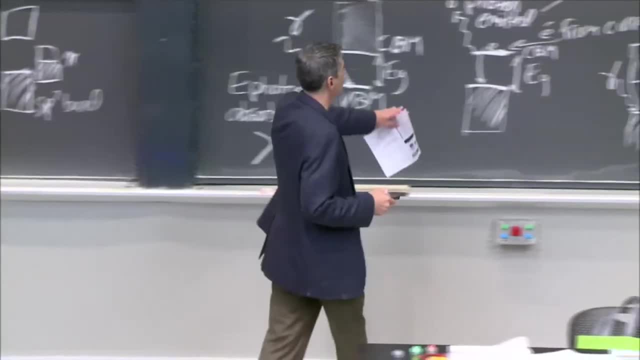 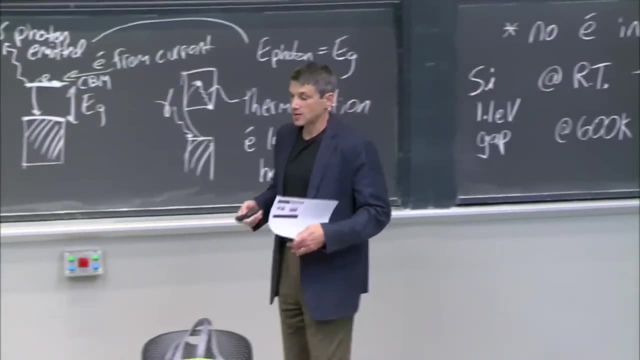 You know why? now I'm populating, I'm getting over this gap And I'm populating the conduction band. So the answer is we just need to run our semiconductor industry and our phones and our lights at around 1,000 Kelvin right. 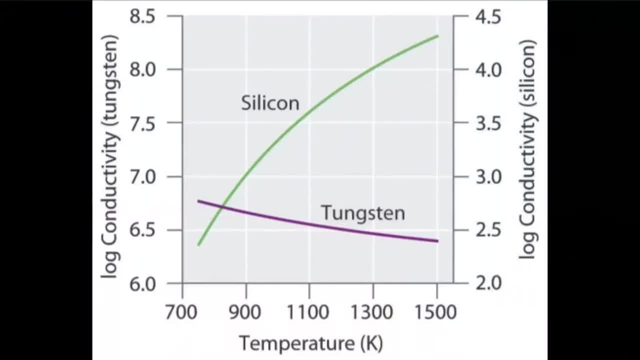 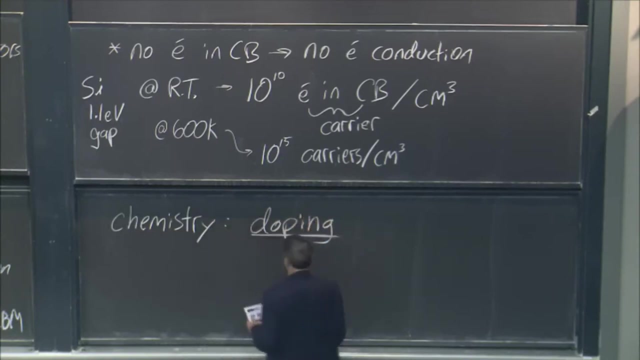 No problem. All our devices? no, Obviously not a good idea. How do we get around this? The answer, oh, such a good word, It's chemistry. Chemistry gets us, Chemistry saves us. As always, you've got to know your chemistry. 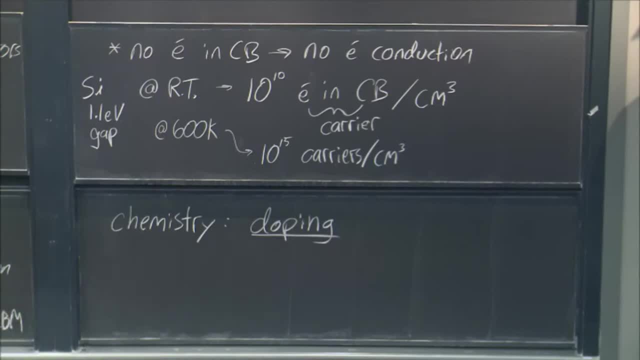 And, in particular, this is not the doping that you may read about in the news related to Olympic athletes. This is, This is This is the introduction. This is the introduction of some small amount, small amount of an impurity. An impurity is something that wasn't there normally. 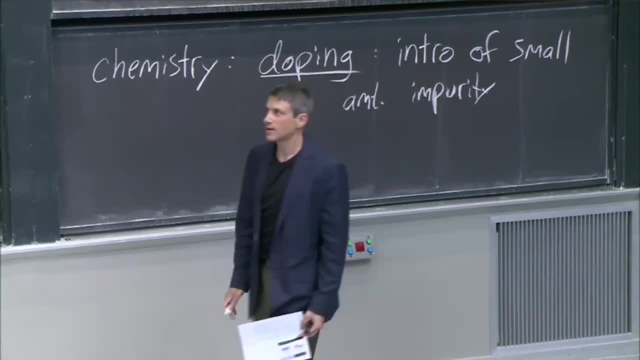 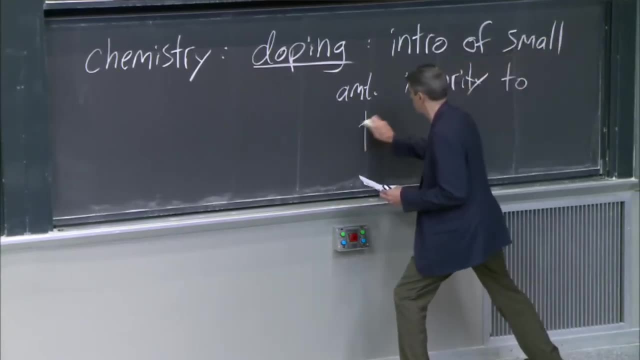 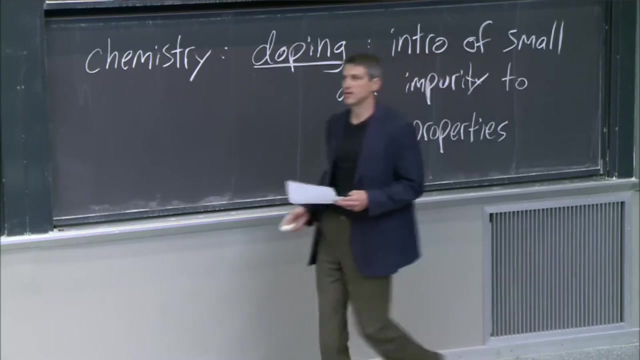 It's like something I mixed in that's not normally there, But if I put a small amount of something in it, then I can tune the properties, And in this case I'm talking about. I'm talking about the conductivity, OK. 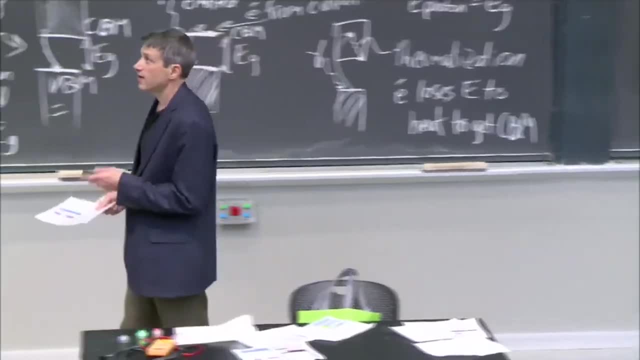 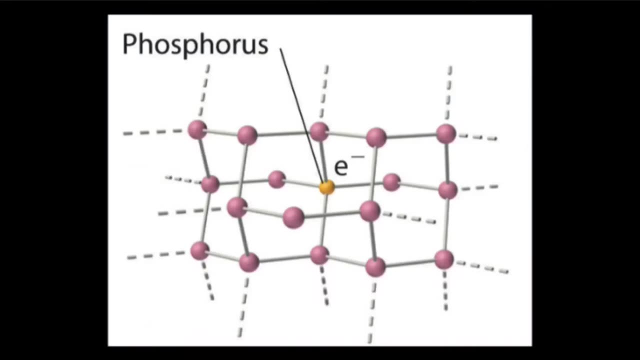 So how does this work If I look at this case? so I'll do one case here. all right, I've got my silicon atoms arranged in this solid. that gave me a band gap And again, that is due to the arrangement of them. 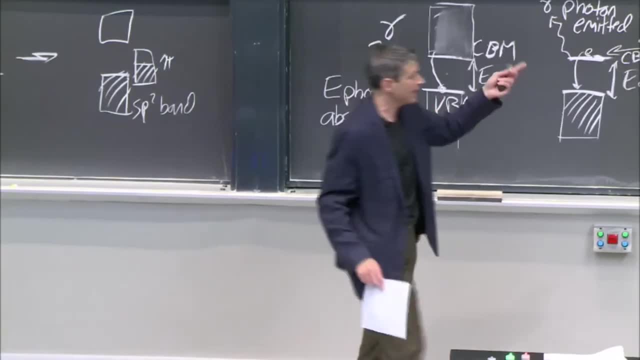 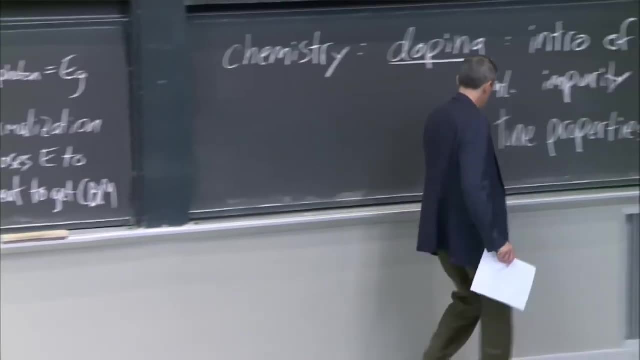 If I didn't arrange them in this particular way, I might not have that band gap, I might not have the same band structure. All right, It depends. But this is what I get for the silicon arrangement when the band gap is 1.1 eV, which. 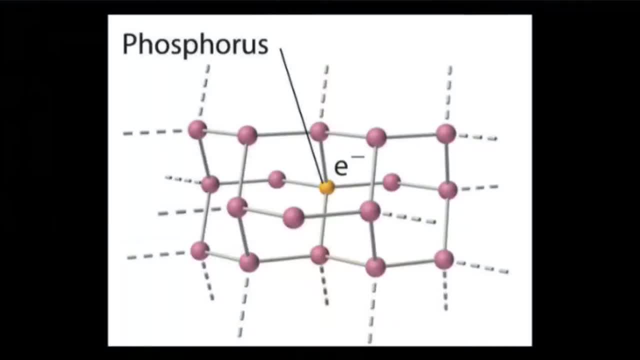 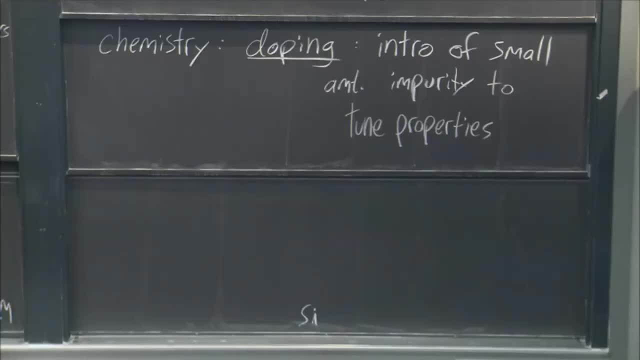 is the one we use in most of our electronics. all right, But the thing is, I want So this would be silicon, This is just silicon by itself. Valence band, And here's the conduction band: Cb, Vb. 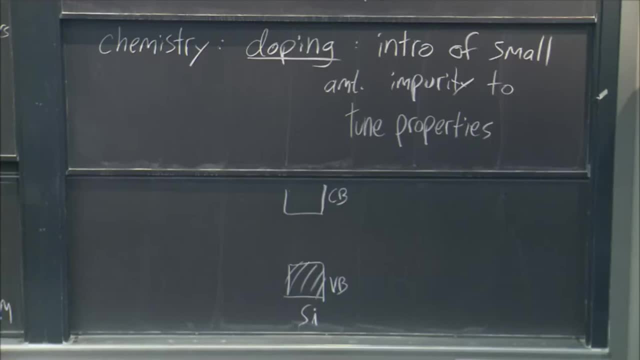 Now I want to add The electrons into this material, And so you can just kind of imagine how this would work, right, If I just look at a Lewis dot diagram for silicon. let's just forget about the structure for a second OK. 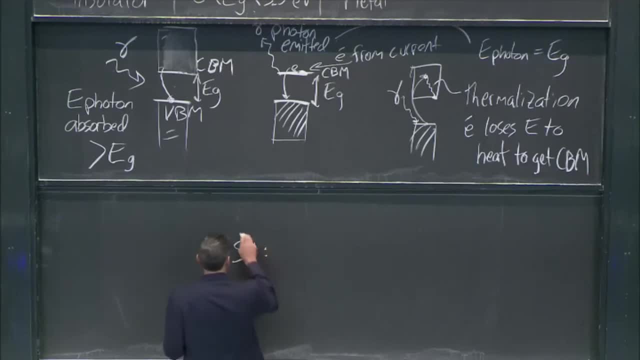 Silicon has these four valence electrons, So you can imagine silicon might look something like this: right And OK, I'm going along and I'm going along. It's tetrahedral and stuff. But now I'm going to take one out. 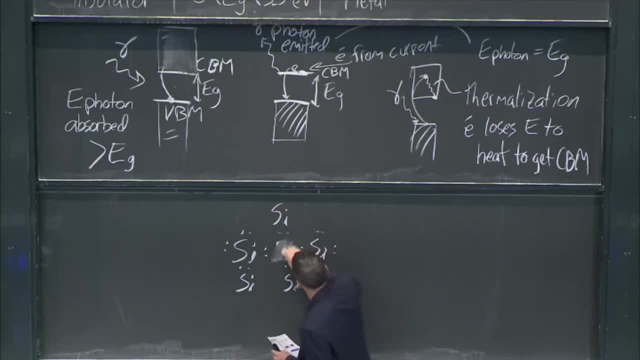 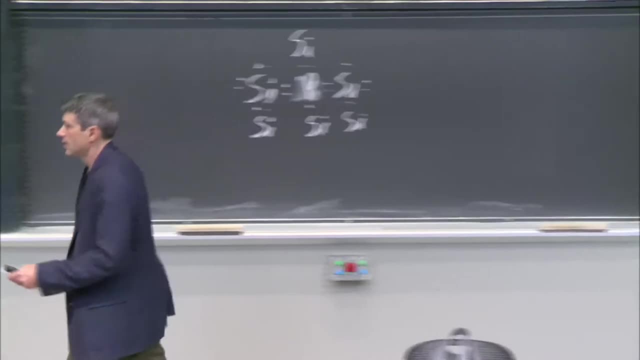 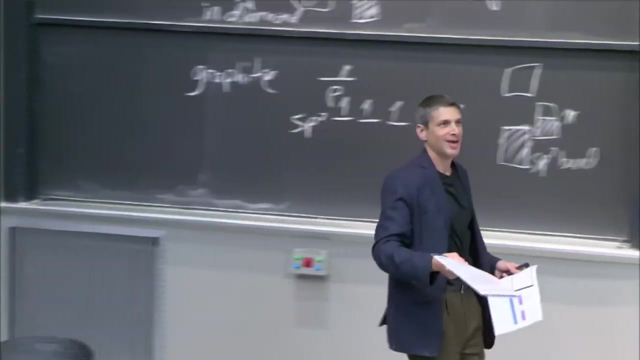 and I'm going to take this out and I'm going to make it phosphorous. Well, what is phosphorous? It's wait, where did it go? Panic. And then I'm recreating what happens for you guys. I found it. 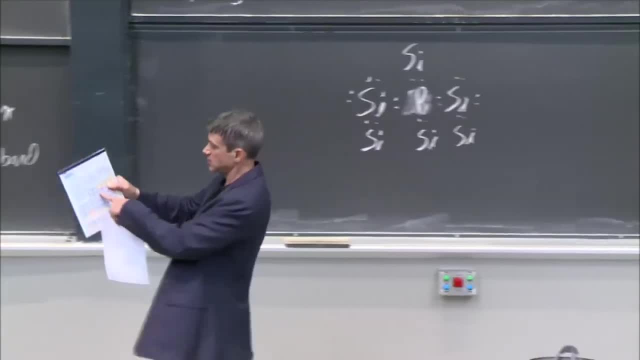 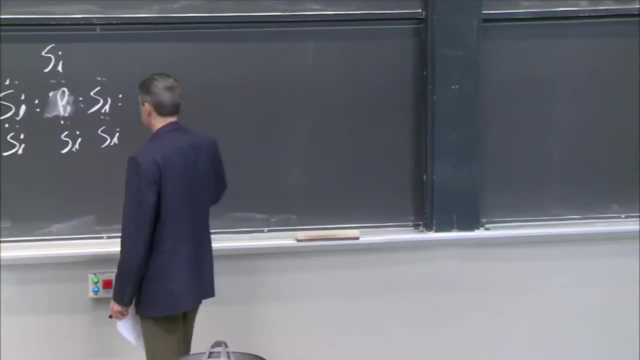 Oh, that was close, But phosphorous is right there. It's right next to silicon. It's group 15 instead of 14.. It's got one, But it just has one extra electron, right, So maybe it could do the same thing. 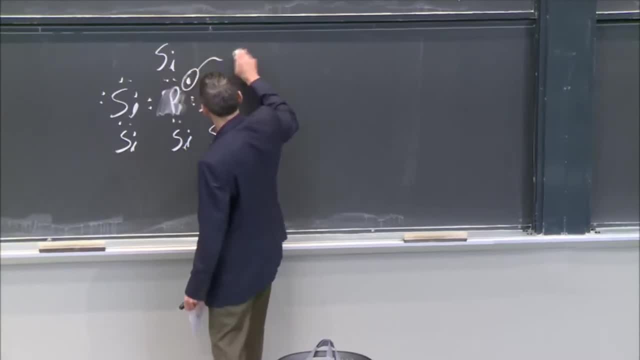 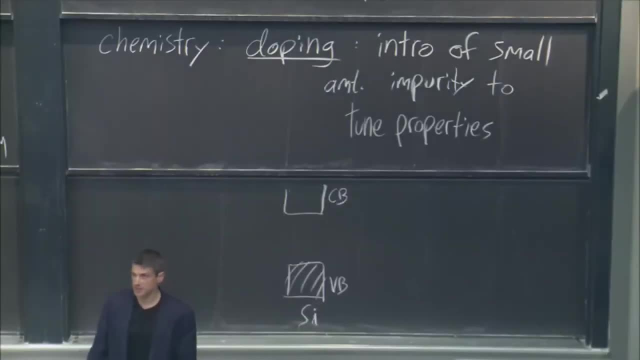 But then have this one extra electron. That's doping. Where does it go? It's all about freedom. It looks down. It says: wait a second, There is no states here. I can go to No states. I can't go anywhere here. 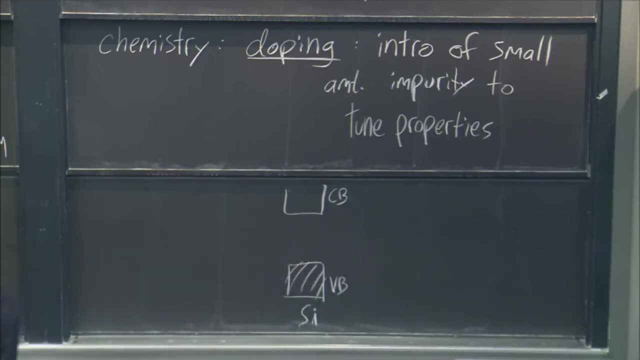 So I will have a state, Because I have picked phosphorus carefully and because of the way the chemistry and the bonding works with phosphorus in silicon, this will introduce A state near the conduction band, And that's the key. So now we've got the valence band. 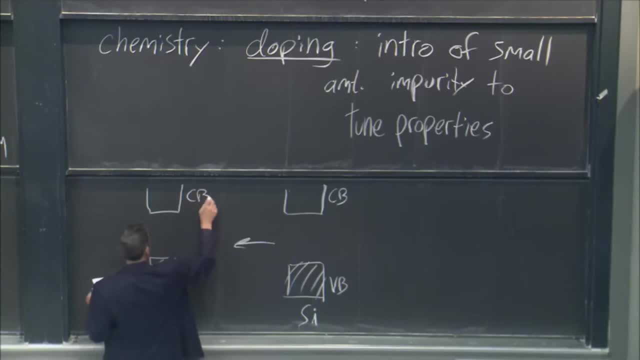 And we've got the conduction band. And what's happened is there's a new level here that is called the donor level. That level is where the extra, extra p electron goes. It can't go in here, remember. This is all filled, right. 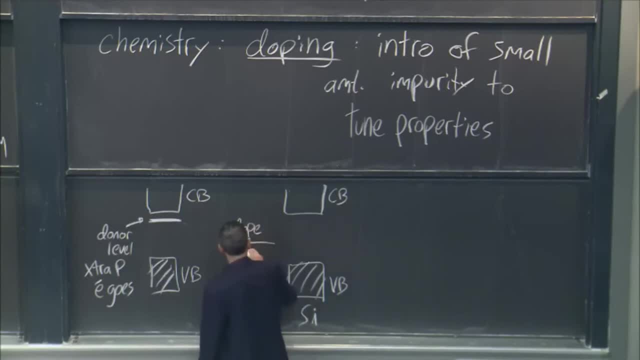 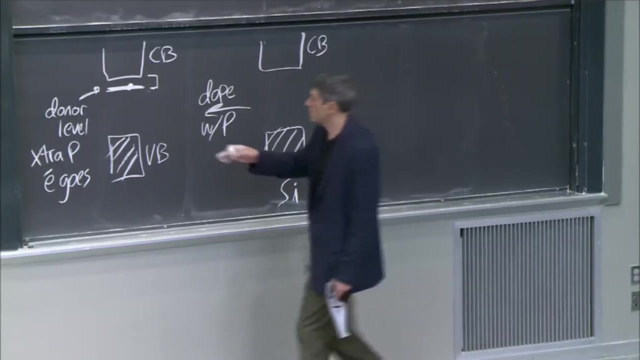 So now I've doped with p, But look if I've got an electron here. now this difference in energy is really small. It's really small. I've engineered it this way. I've thought about this. So if I put phosphorus in here, that extra electron- 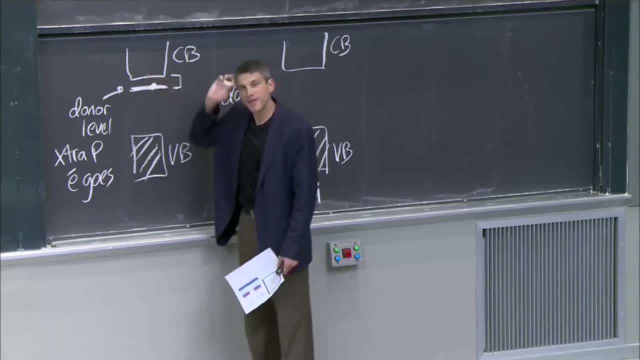 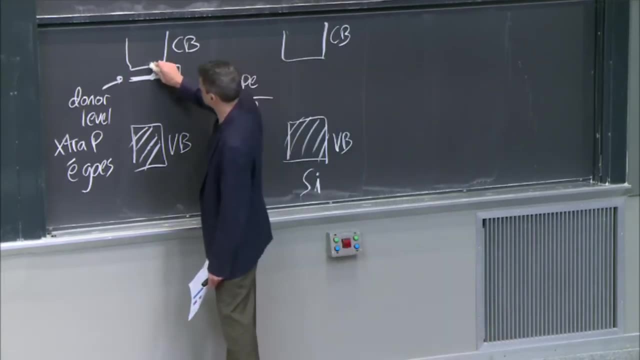 isn't sitting far away anymore from the conduction band. In fact Now it's so close that room temperature just kicks it right on up So effectively it's going to go up here Because that's a small delta E between the donor level. 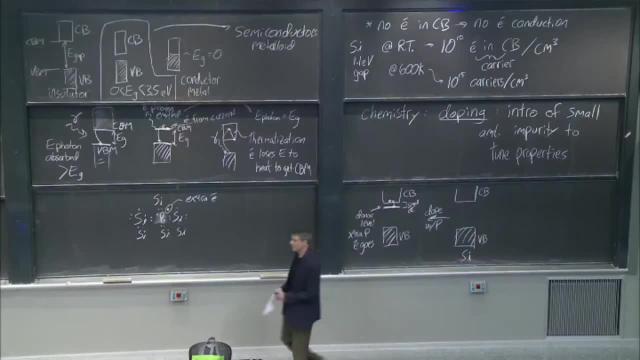 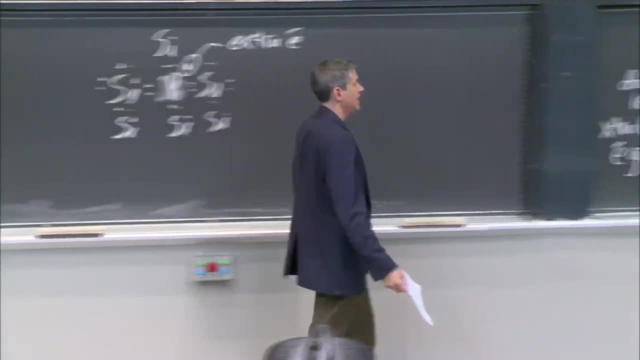 and the conduction band. This is how doping works. This is how doping works. So I put a phosphorus atom in. There's an extra electron that comes out of that. The extra electron needs a state. It gets a state That's called the donor state. 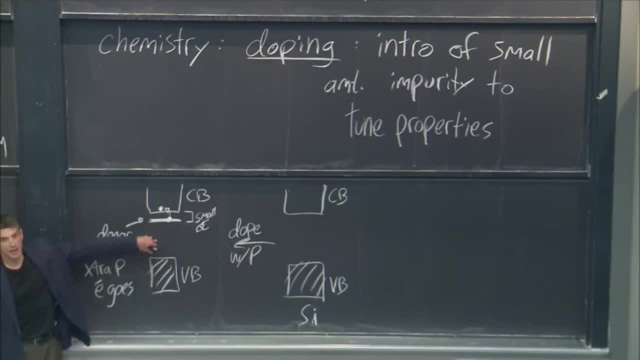 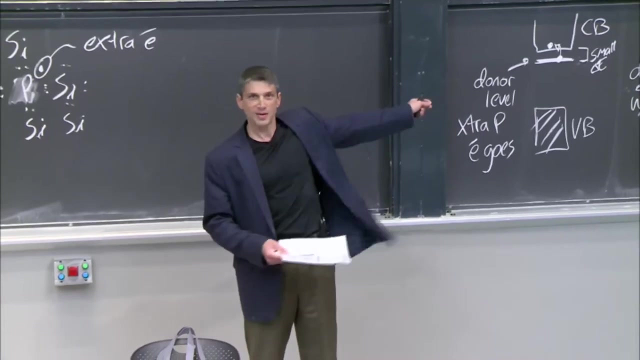 Donor makes sense right Because it's donating an electron. So I put an electron into the conduction band Right. Once I get the electron into the conduction band I'm home free, Because now I've done what temperature was doing before. 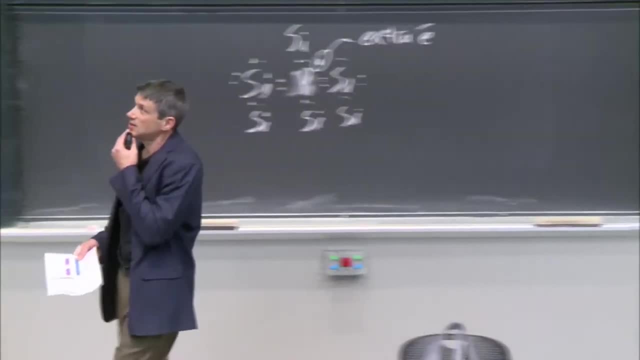 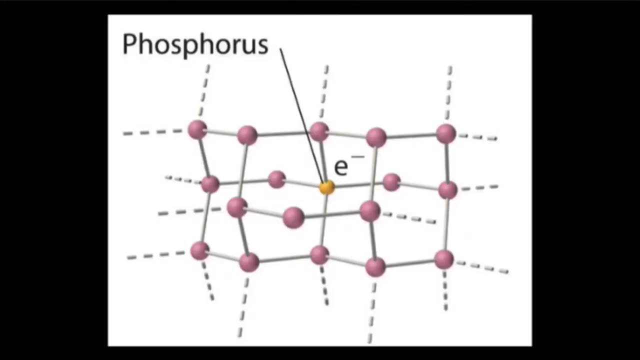 but I did it with chemistry, And so you could ask questions like this: right, How much phosphorus do you need to substitutionally dope? Substitution meant just what you should. Substitution was: I took a silicon atom and I substituted it. 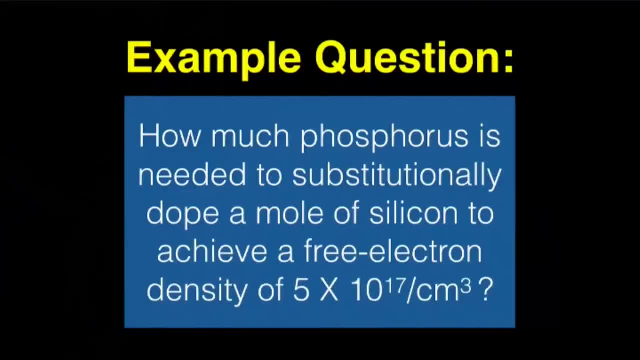 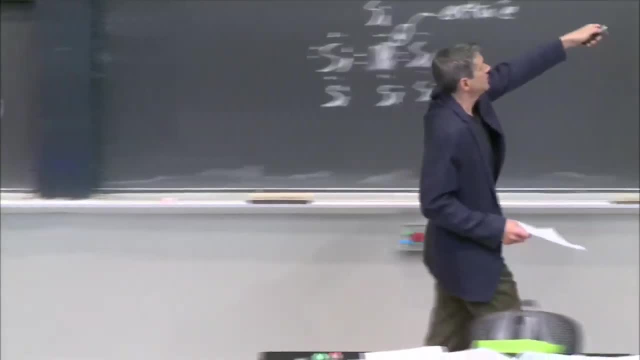 That's substitutional doping. To substitutionally dope a mole of silicon and get a free electron density of 5 times 10 to the 17th. I'm going big here Because look, temperature, gesundheit, Temperature. OK, maybe I'm willing to run. 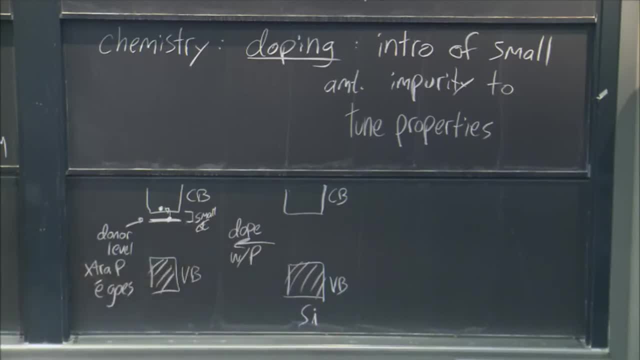 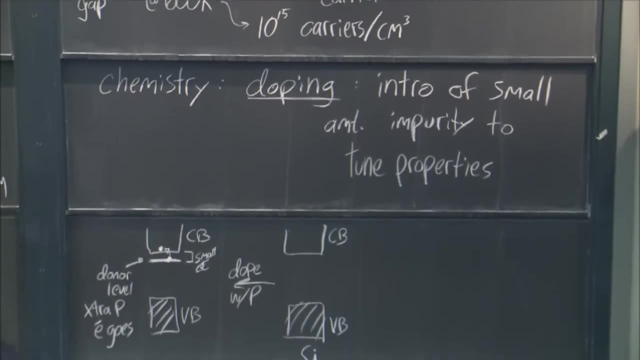 my semiconductor in a really hot room, my phone at 600 Kelvin. I'm still only at 10 to the 15th. I want 10 to the 17th. now, How much phosphorus do I need? You can solve that problem. 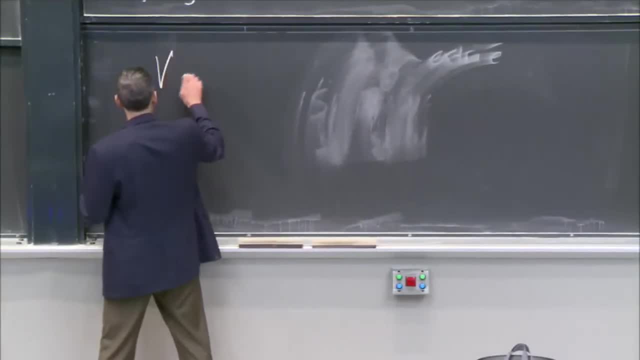 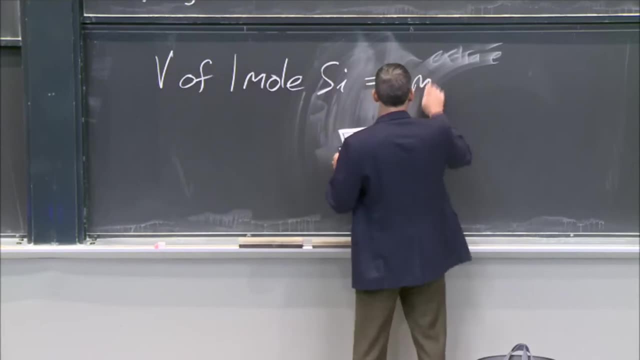 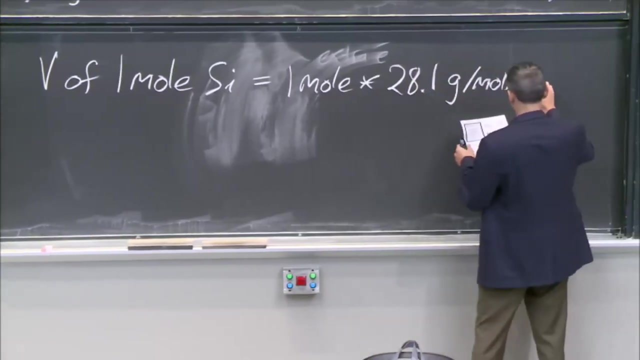 I'll just write down, OK, A couple of the steps, right? So the volume of one mole of silicon is one mole times 28.1 grams per mole. Oh, and I got the density on there too, right, Divided by 2.33 grams per centimeter cubed. 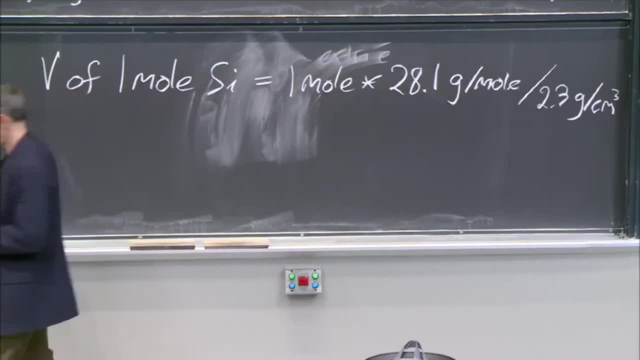 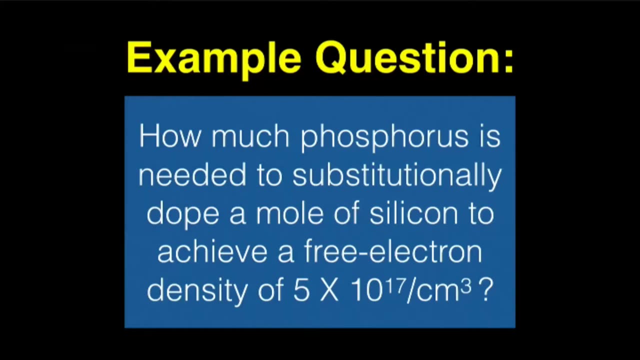 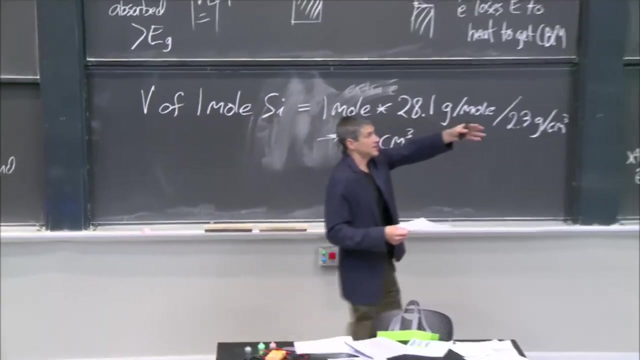 How did I get the density? I looked it up in the periodic table, And so one mole of silicon is going to give me 12 centimeters cubed of silicon. One mole of silicon is 12 centimeters cubed. I need 5 times 10 to the 17th electrons. 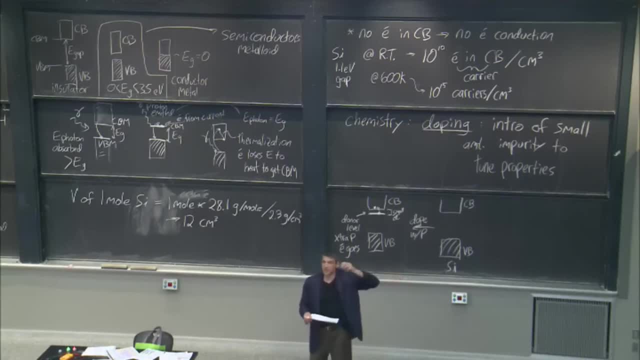 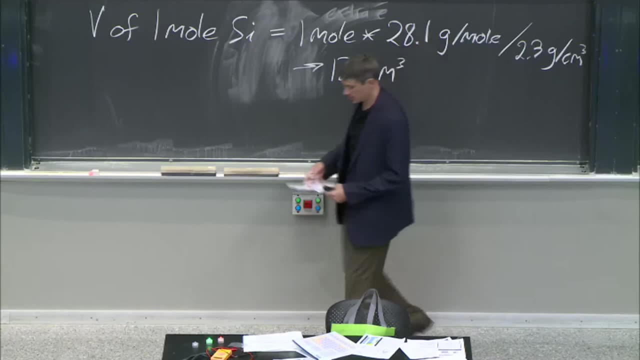 in the conduction band per centimeter cubed. That's why you see why per centimeter cubed is a good measure here. So that means I need 12 times that total. So I need 12 times that. so I need 5 times 10 to the 17th. 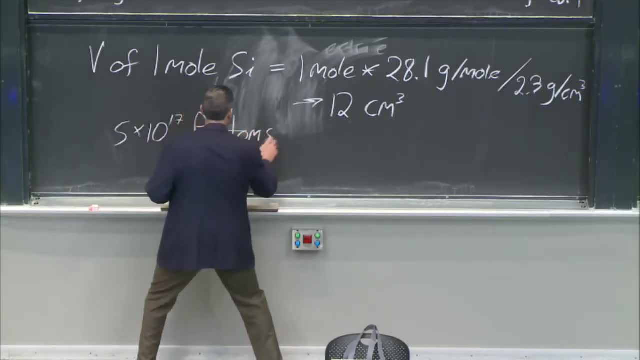 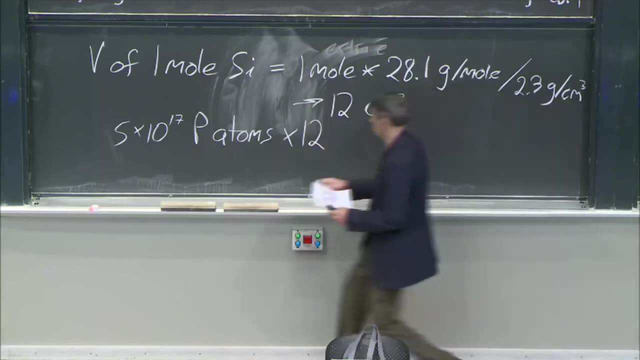 So I need 5 times 10 to the 17th p atoms. Why do I need that many p atoms? times 12, right, It's 5 times 10 to the. let me just write my units here, to be very careful. 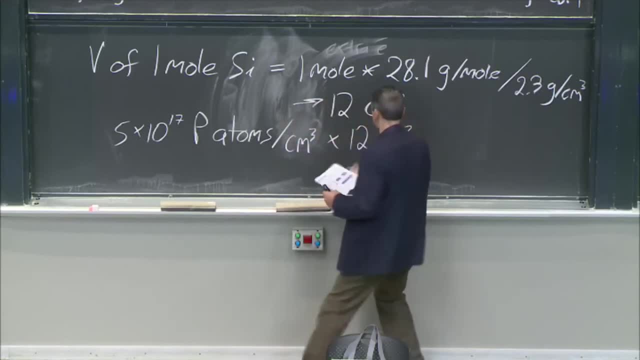 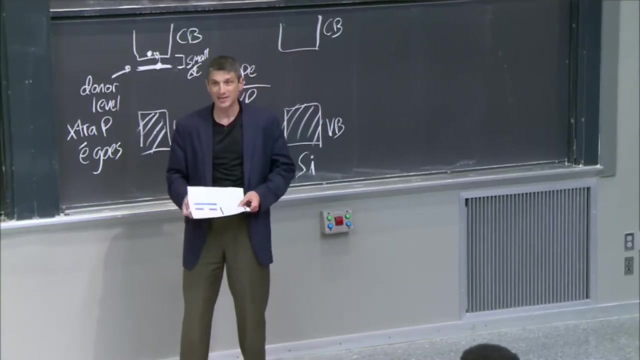 p atoms per centimeter cubed times 12 centimeters cubed, That's how many p atoms I need in this mole of silicon to get. But it's 1 to 1. Because each p atom, Those other electrons are in the bonds. They're not going into the conduction band. It had one for one. One electron went to this donor state, went into the conduction band per phosphorus atom. So if I want that many carriers, if I want that many free electrons, I need that many atoms. 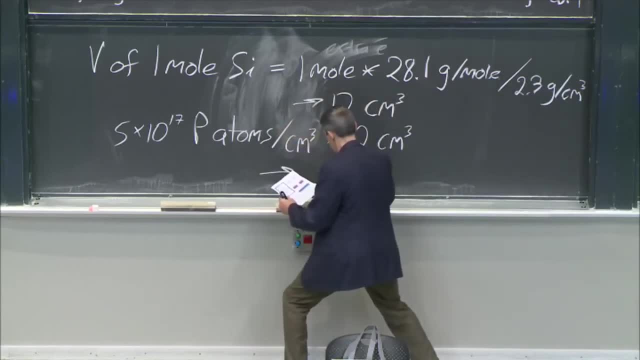 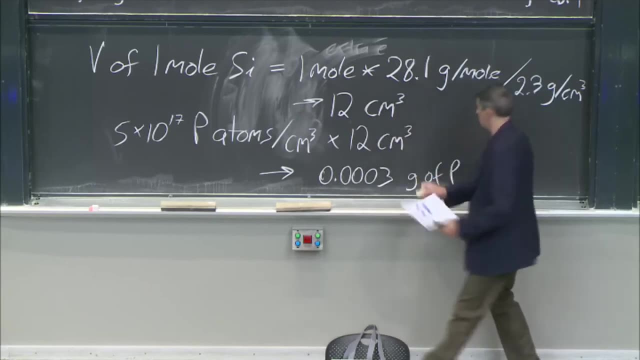 Well, you guys can look up the phosphorus grams per mole and you can get that this is 0.0003 grams. That's really not much. You see why it's called an impurity. right, You see why it's called an impurity. 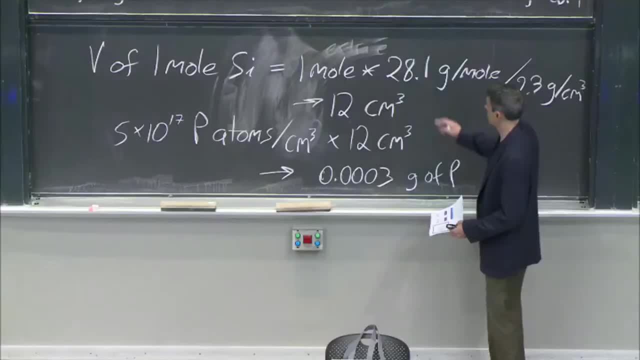 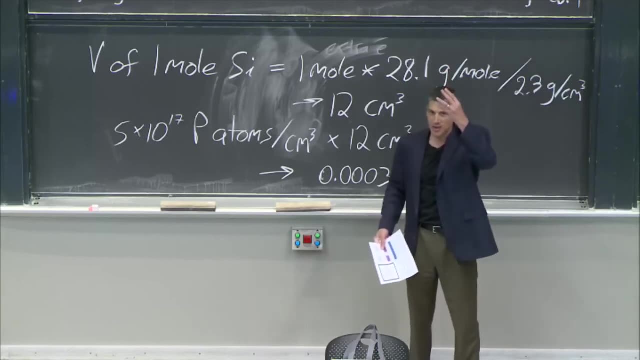 That's not much. I have all this silicon and I only need 0.0003 grams of phosphorus, And I've bumped up the number of carriers by orders of magnitude. Not only that, I've done something really important as well. 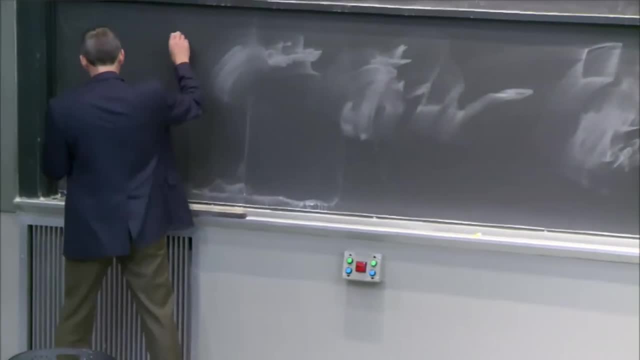 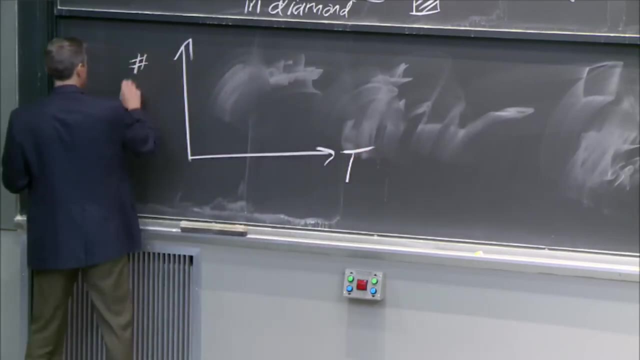 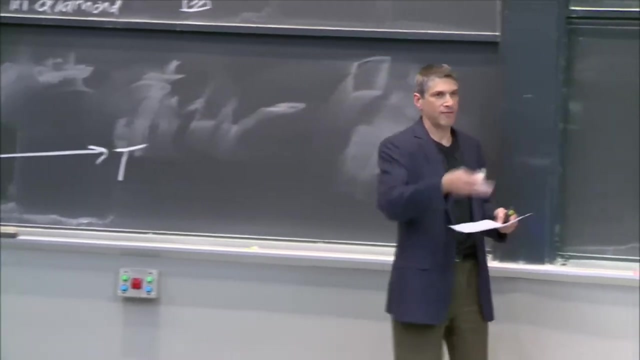 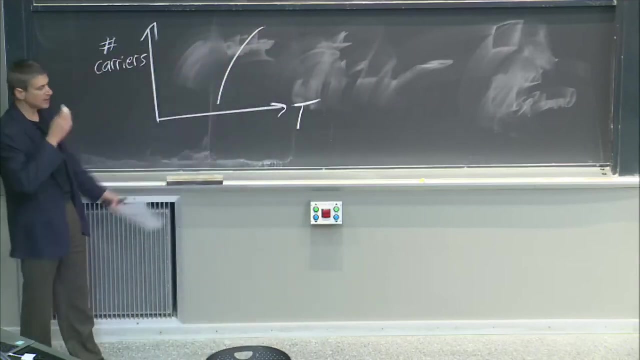 And you can see this, Because now, if I plot something like, You know, temperature versus number of carriers, Well, you saw the graph for temperature before, right, It was like this: That's the graph from a couple of slides ago. 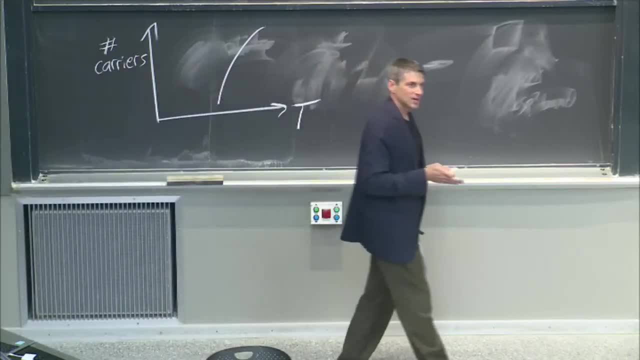 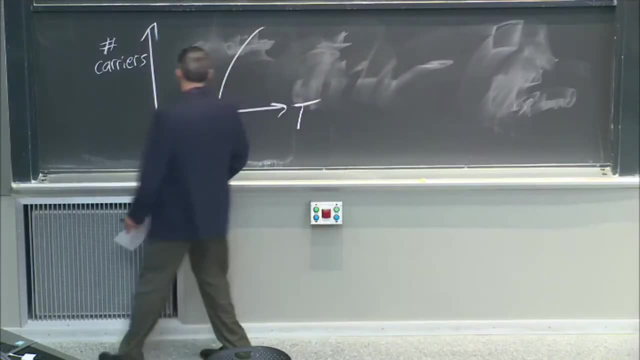 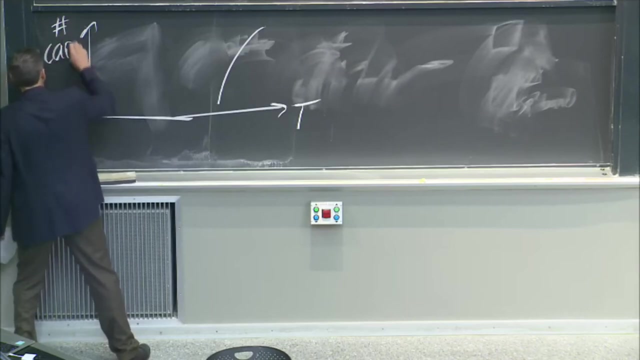 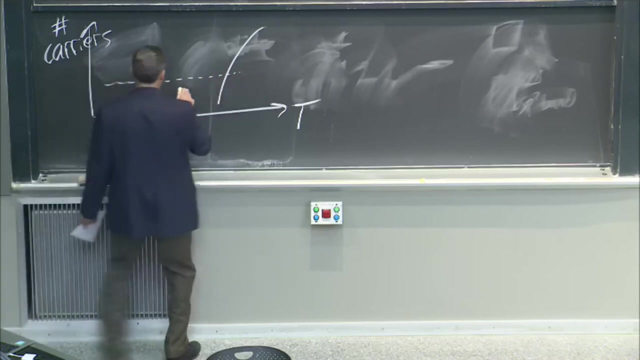 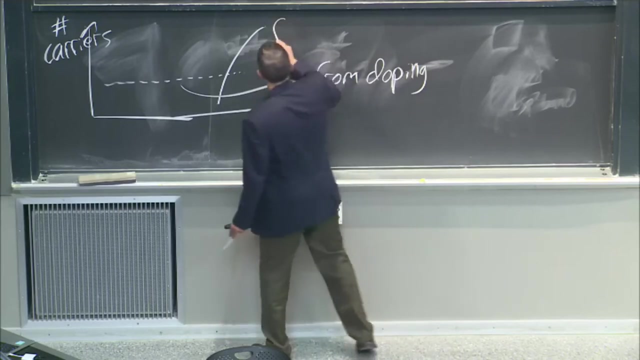 But now if I do it with chemistry it's flat. I can choose at any time Until the temperature gets really hot. I could give myself more room here, because that's kind of the point. right Number of carriers. I can make this now flat from doping, from temperature. 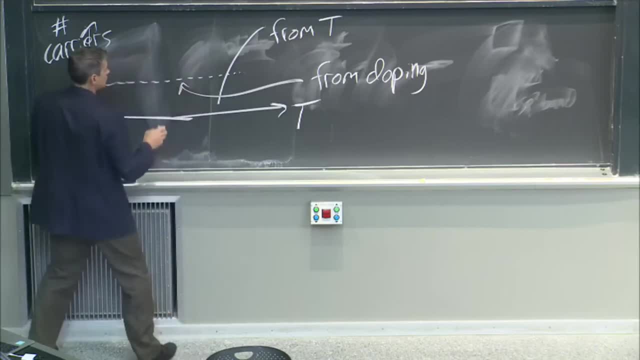 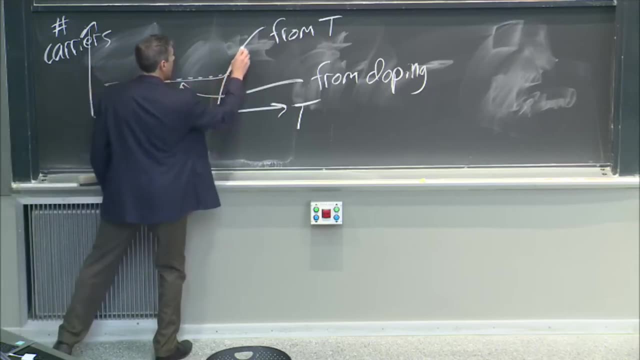 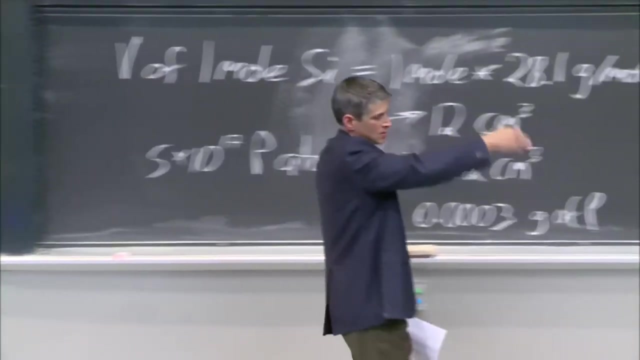 And so you can see. OK, at a certain point, at a certain point the temperature goes up, up, up, And at a certain point the temperature is going to be so hot that I'm adding electrons even beyond this. But you saw what temperatures are at 1,000 degrees Kelvin. 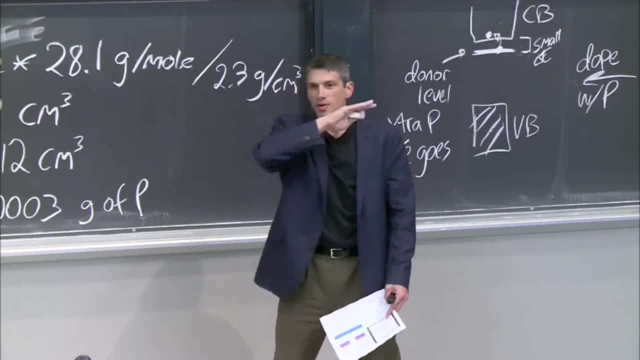 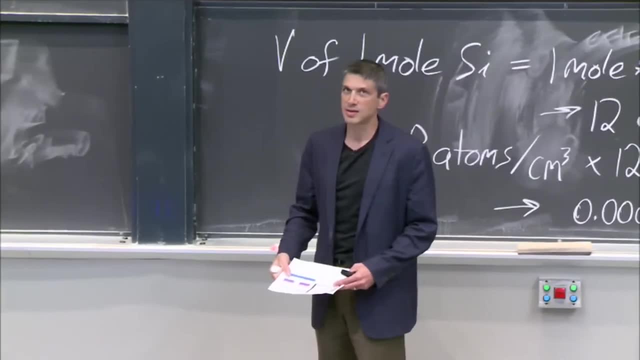 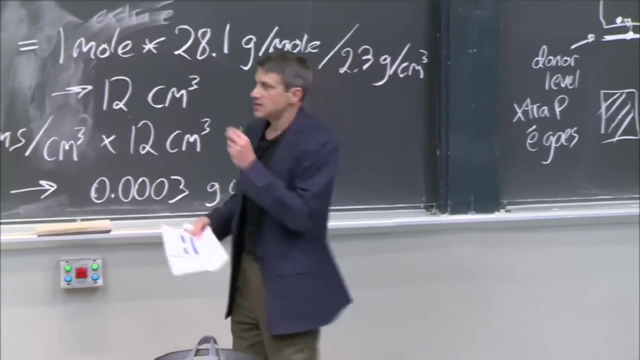 No, this allows me to have a predictable flat number of carriers in the conduction band, no matter the temperature. Just think about how important that is. This is why semiconductors were kind of discovered in the 1800s, But it wasn't until physicists and chemists 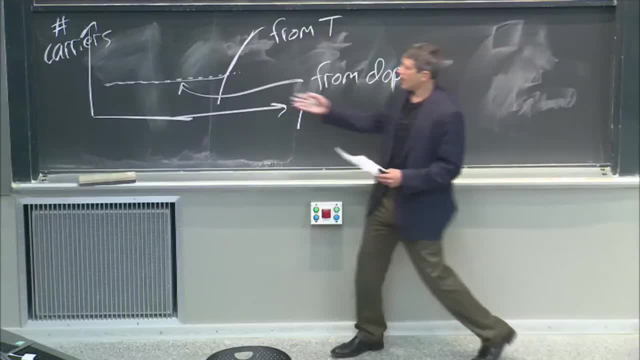 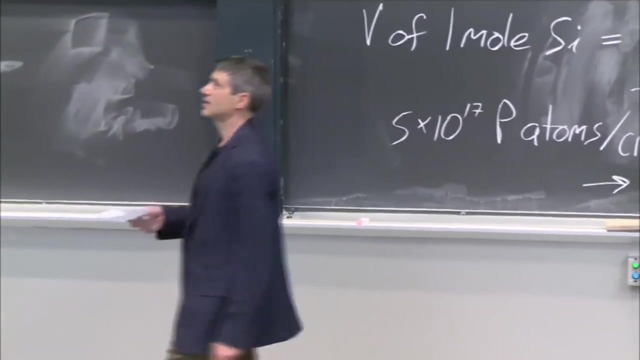 were able to control the band gap and how to put carriers in and out of it until they could really work on the semiconductor revolution, which is what led to Snapchat. Snapchat is still used. Yeah, I knew that Slack. OK, now you can do the same thing going the other way. 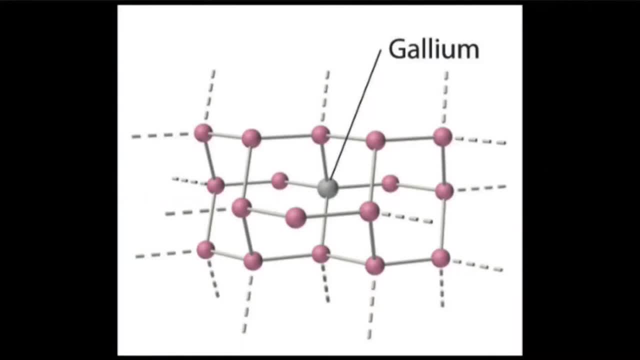 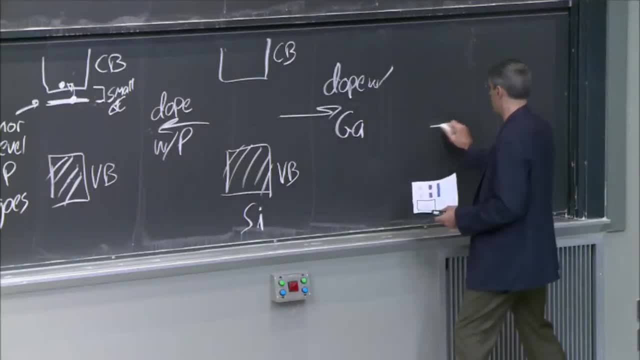 You can do the same thing going the other way, Because if I now put gallium, so if I dope with gallium, well you see, gallium has one too few electrons And so if I dope with gallium, what I have, 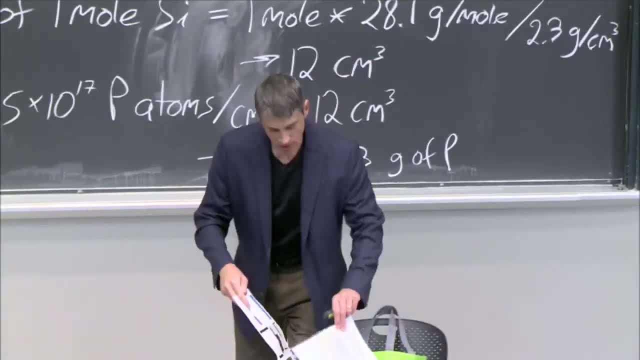 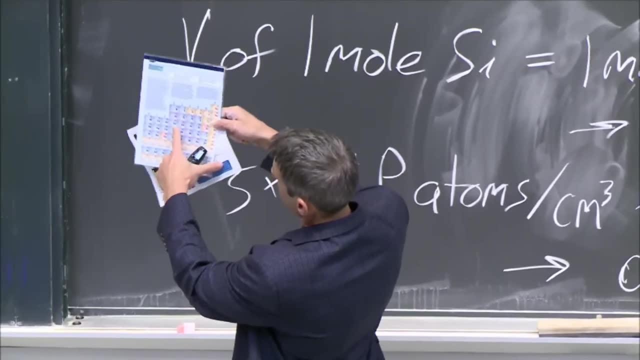 so the gallium is there. Where is it? It's on the other side. Where's silicon? OK, silicon, right. Phosphorus is over there, group 15. Silicon is group 14.. Gallium is group 13.. 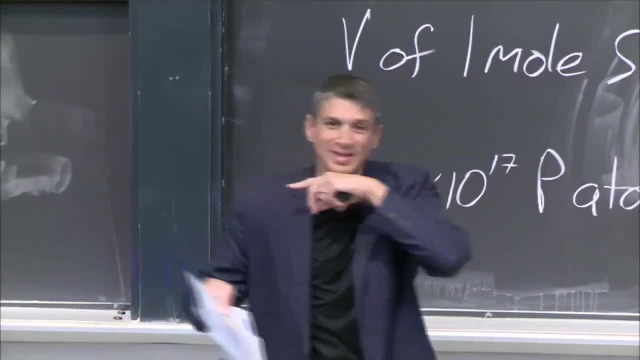 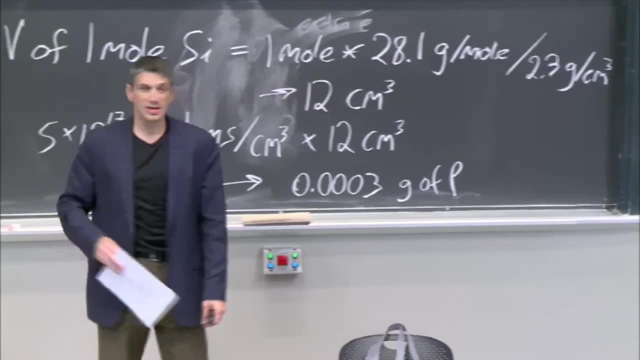 One fewer electrons, But it really wants to make those four bonds. The material isn't happy if you break one right. And so what does it do? It steals an electron, It takes it. It says I need an electron to be happy. 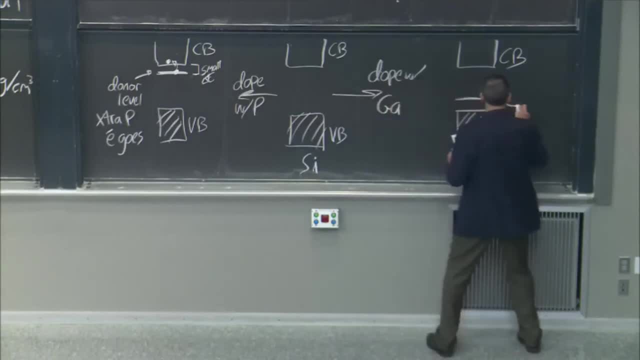 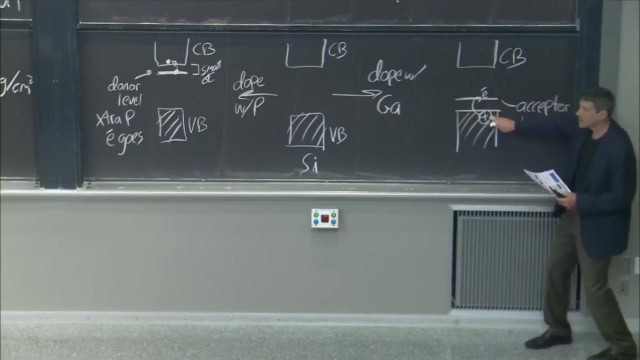 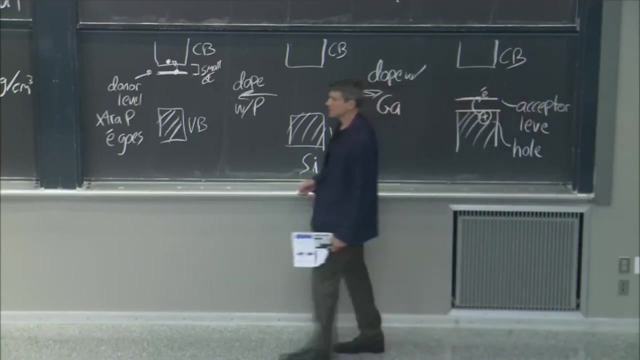 So it takes one out And that's called an acceptor level. acceptor level where what's happened is the gallium has actually pulled an electron out of there And that leaves behind a positive charge. This is called a hole. That's called a hole. 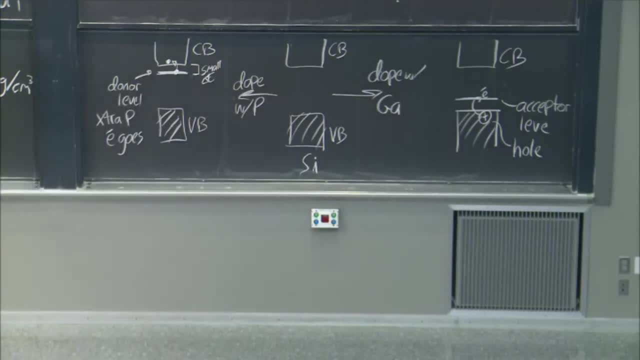 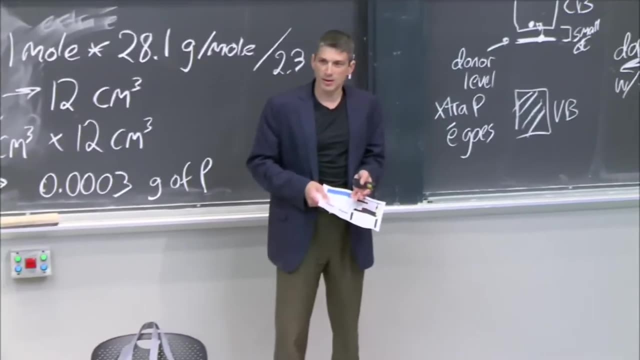 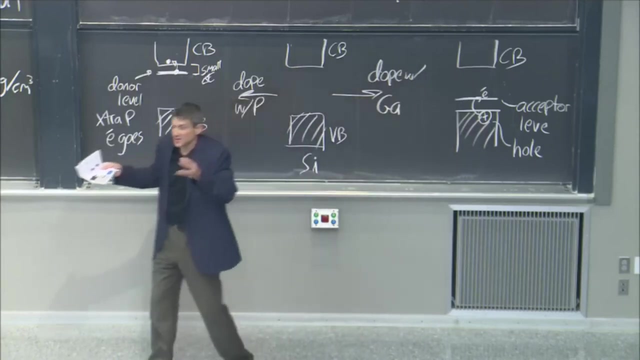 A hole is. think about it. If I take an electron off of an atom, it's positively charged. If I take an electron out of the VBM, there's a positive charge in there. That's really important Because these positive charges effectively. 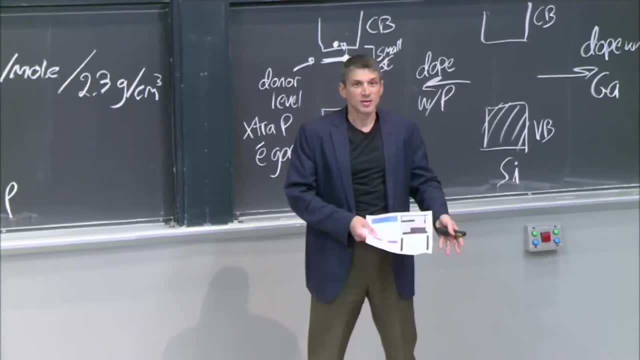 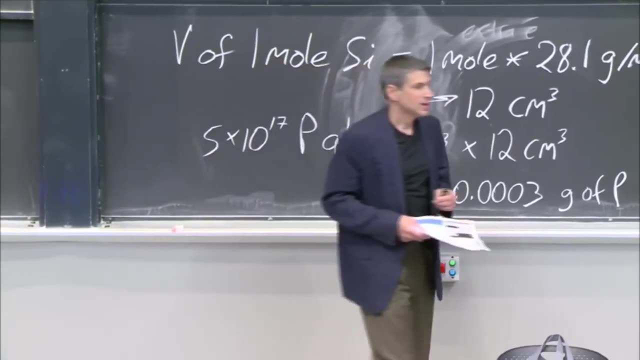 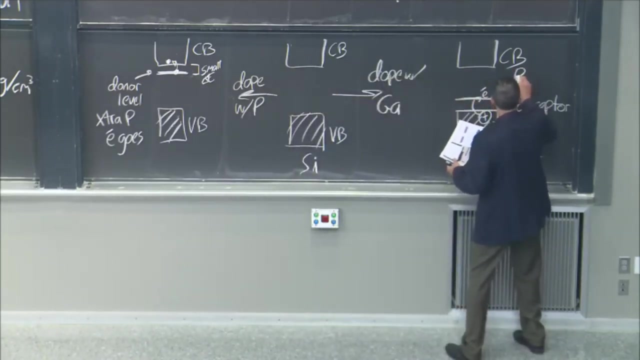 are like electrons, They're like negative charges, but they're positive, So they also can conduct. They also can conduct right And that's really important. So these are two different types And you can imagine the brilliance of the naming. 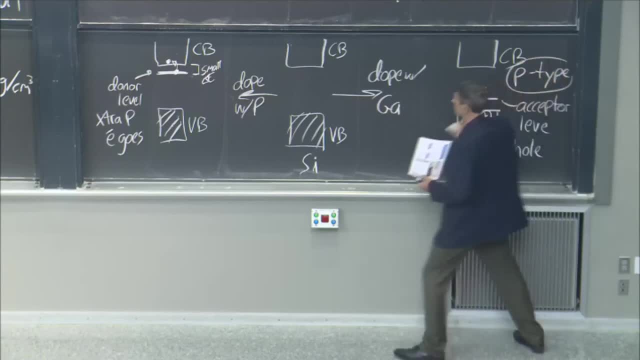 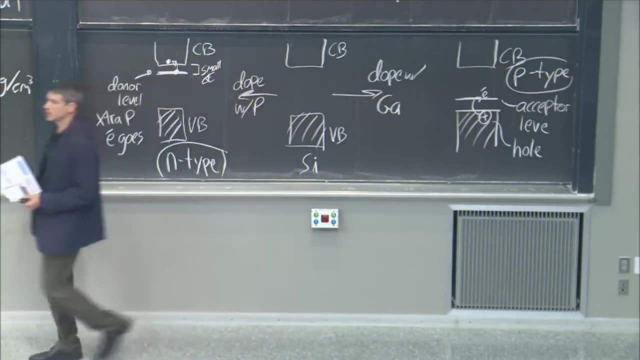 These are p-type because it's a positive charge And these are n-type because it's a negative charge. Those are n-type semiconductors. What does that mean? I've used a little chemistry, sprinkled a little something with extra electrons. 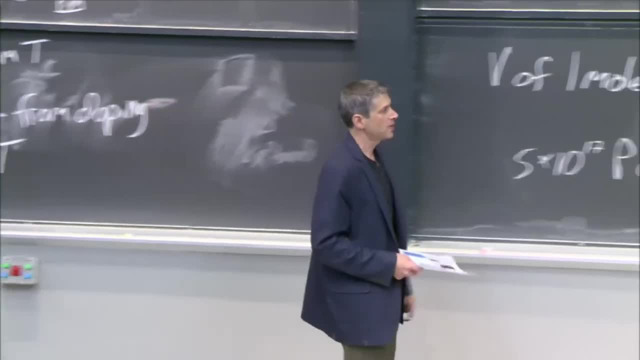 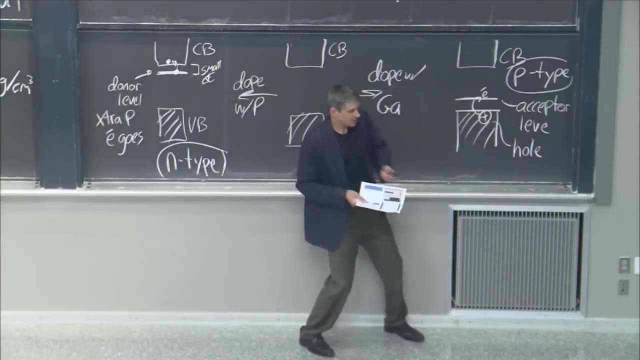 It's got negative charge in the conduction band p-type. p means positive. It means that I have introduced states here. because I needed an electron, I said I need an extra one. I'm going to grab it from somebody, I don't care who. 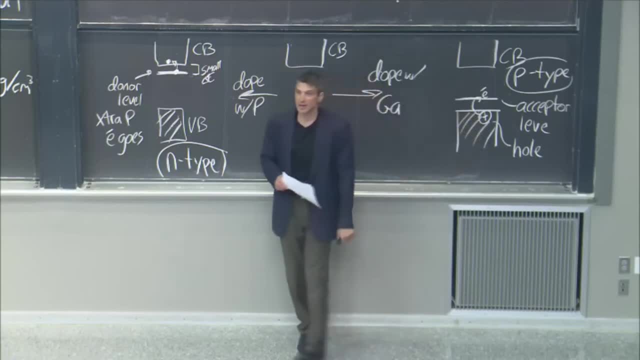 And so you create a positive charge in the valence band That can conduct electricity, just like a negative charge in the conduction band can. This is what the entire semiconductor revolution has been based on, And really so much of the focus was. 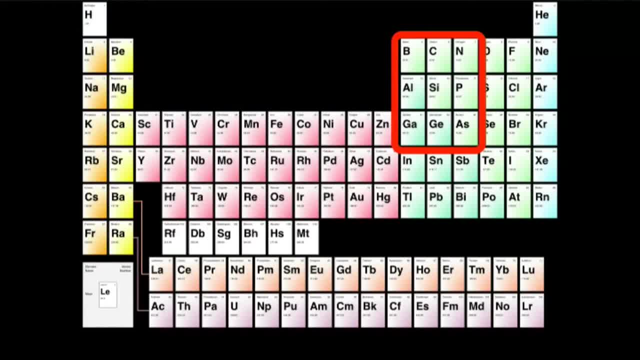 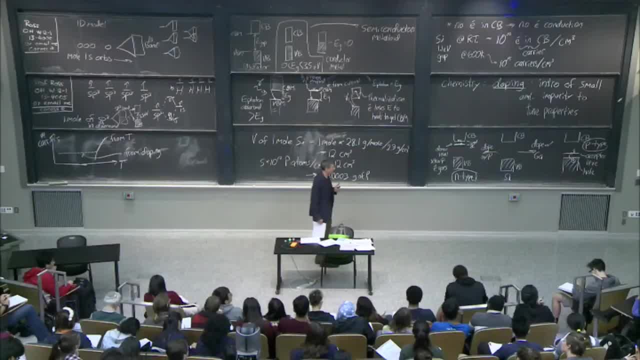 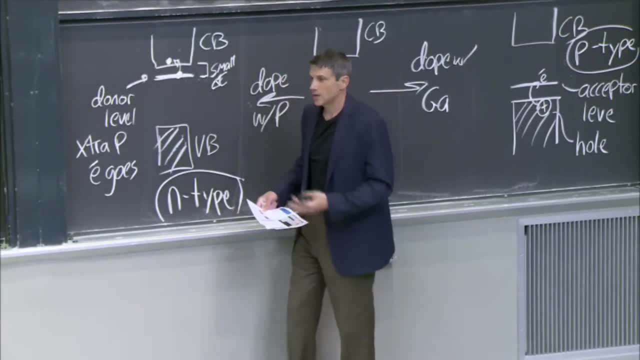 on simply taking these elements, in particular silicon and germanium, but then many, many more. as I showed you in the LED graph, many, many more have been used to engineer these seemingly simple properties- the band gap and the doping, And so I'm not going to go through this in detail. 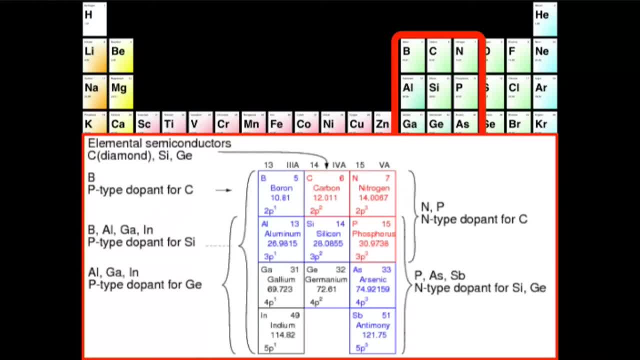 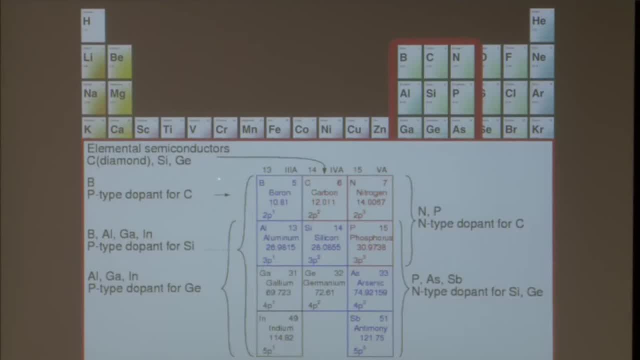 I'm just leaving it here, so you have it. But you get charts like this. So here you have. OK, carbon is up there. And what can you dope? Well, if you dope it with boron, you can see that it's p-type. 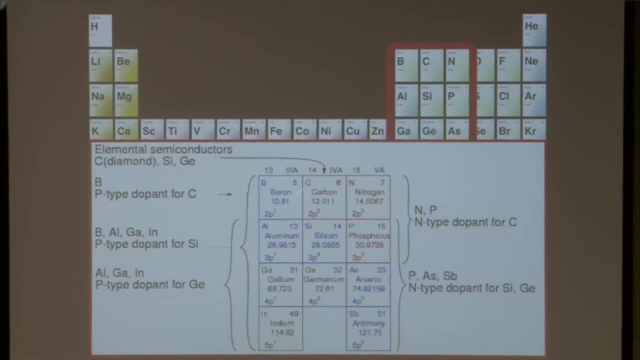 You see that, Because I've got one fewer electron than carbon, So I'm going to grab that from the valence band. create a positive charge, p-type. I could also dope silicon and germanium And I say carbon, silicon, germanium. 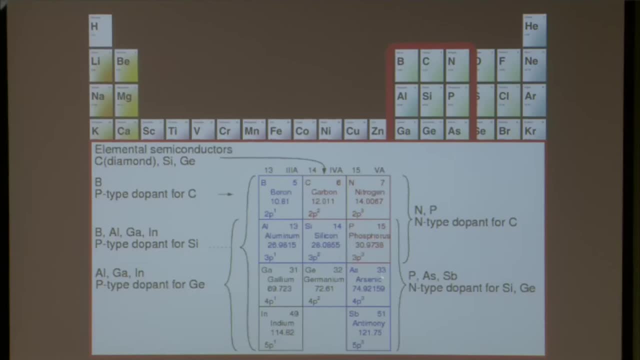 So I'm looking at this middle column doping it with either side. Why can't I put? Why can't I put aluminum in carbon? Why didn't they list that? Well, because there, if I try to put an aluminum inside the carbon network, the network gets all messed up. 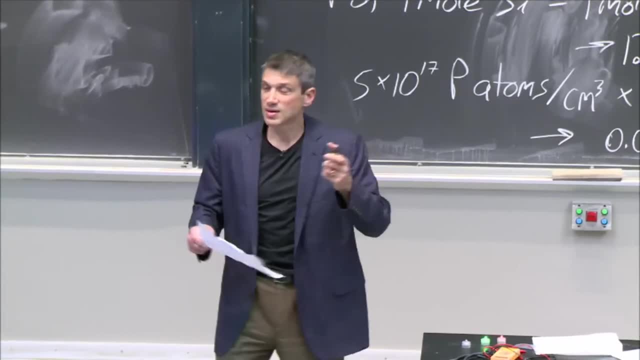 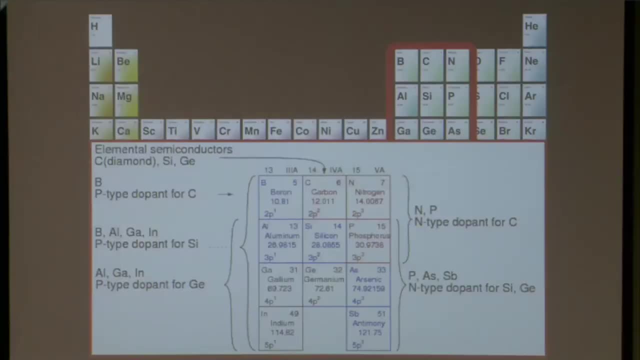 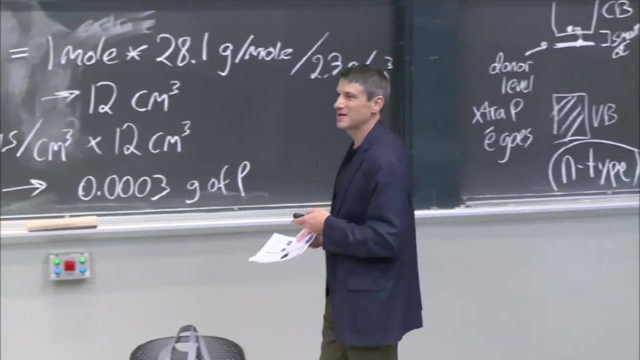 It doesn't fit. So that's also important, Can it fit? But it's through this that the semiconductor revolution started. It's only through this, this kind of control and this knowledge of atomic orbitals- really, if you think about it- and the structure of the atom. 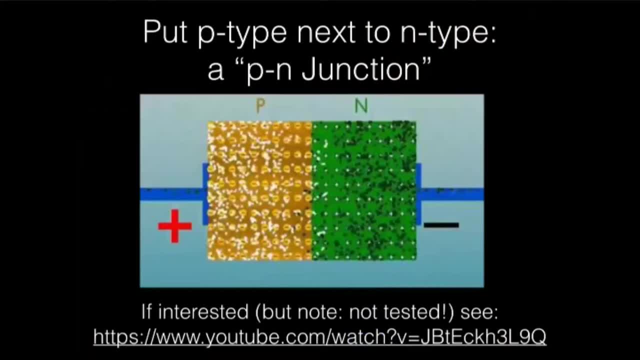 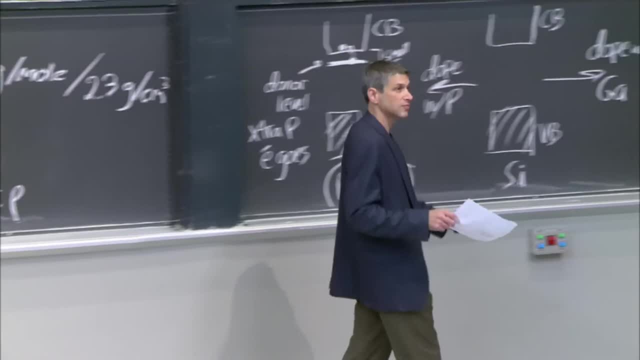 Now I'm not going to talk about transistors, But this did lead to the development of the transistor. If I take, there's a really nice video there. It's like eight, nine minutes. I suggest you wait until your Friday night social. 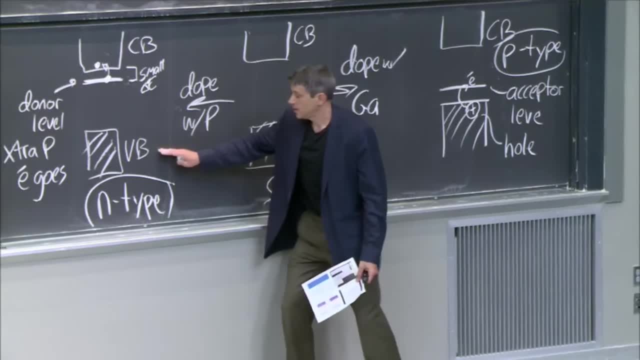 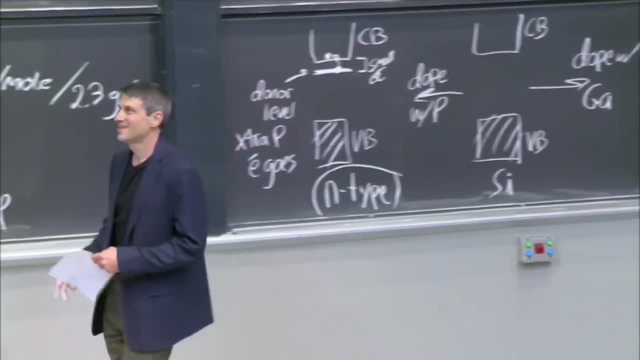 But if I take a p-type and I take an n-type, and I take a p-type and I put them together, some really important things happen, So important that it led to this, which is the very first transistor. That's the transistor. 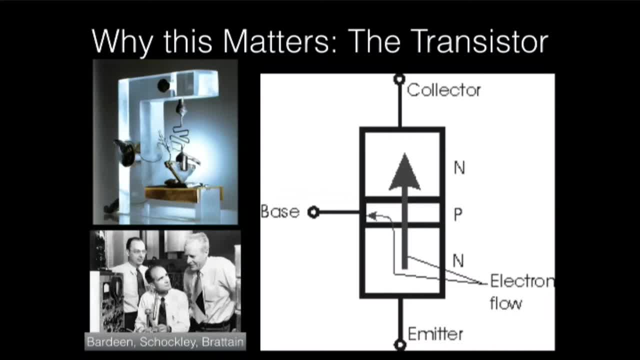 It's a dope semiconductor one type next to a dope semiconductor another type. Now those are the three people- Bardeen, Shockley and Bertain- who won the Nobel Prize for this work, And that's the first transistor. 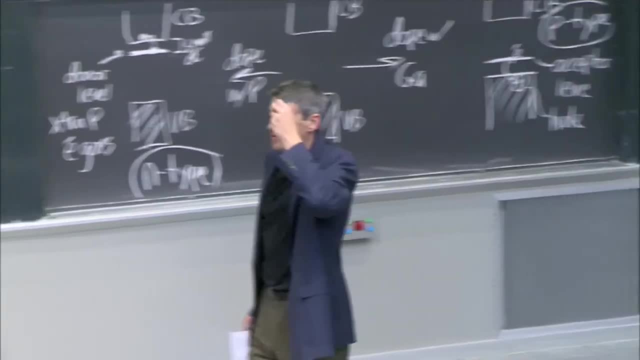 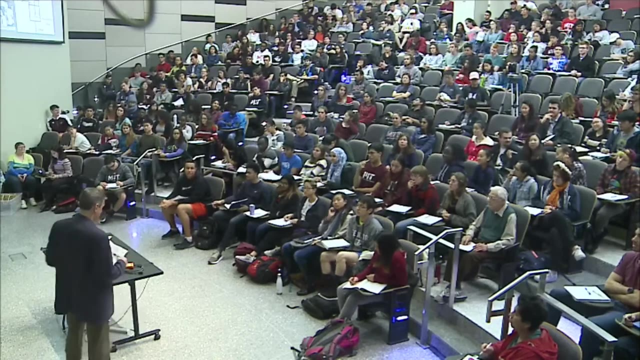 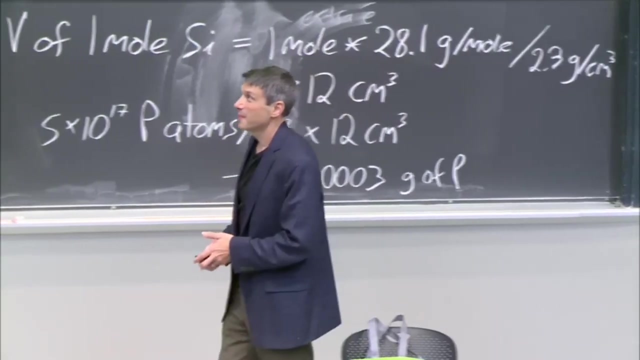 Does anybody know how many transistors we make today Per second? That's the only time metric we can use. Yeah, it's something around 10 trillion. We make 10 trillion transistors per second today. This is a big deal. 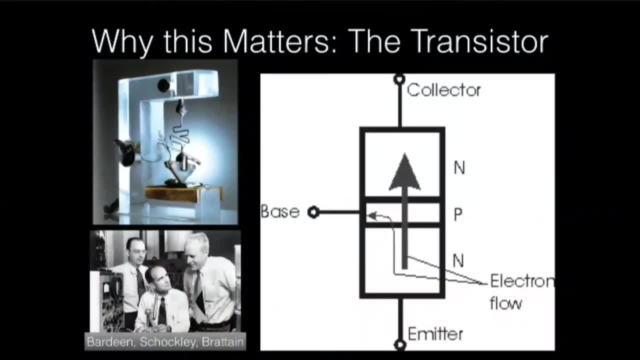 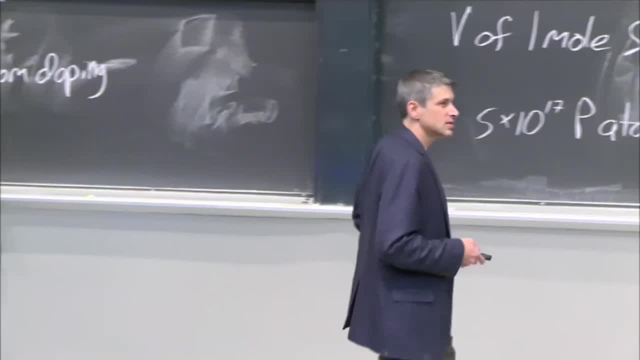 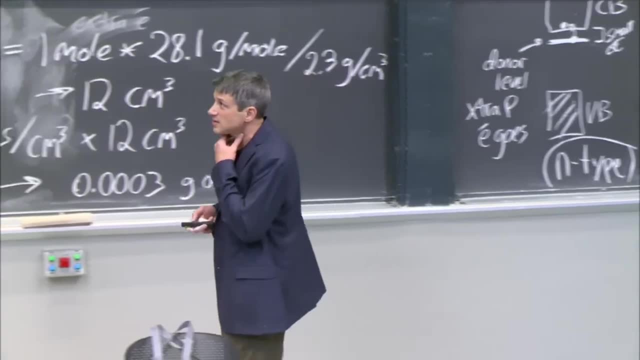 This started it all, and it's all about chemistry and then the physics of this device. right. This led to diodes and photodiodes. This led to the whole revolution, And what I want to point out here is that this also led- it called on- chemistry. 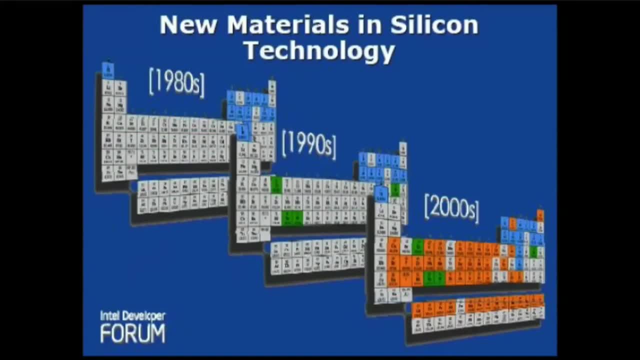 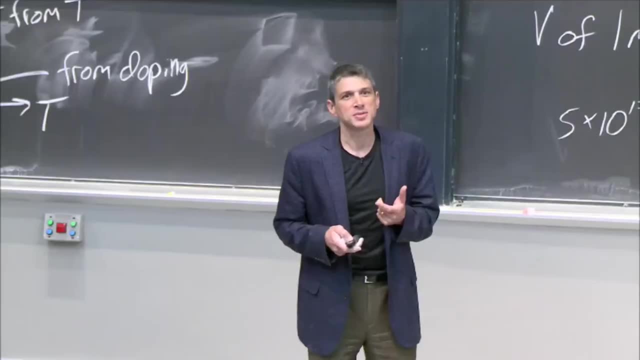 So I love this chart. This is at the beginning. Unfortunately they didn't update it, But this is an Intel chart that they used to show, And what they're showing is: how are they making chips right? How much of the periodic table do they? 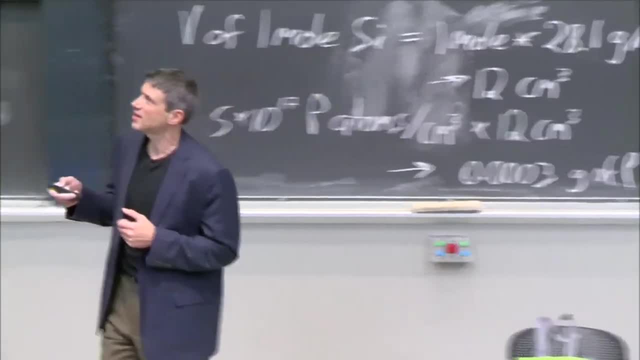 need to make the current chip Well in the 80s there's almost nothing lit up here. There's a little bit over here that you can't see- stuff we just talked about. But look at the 90s and look at the 2000s. 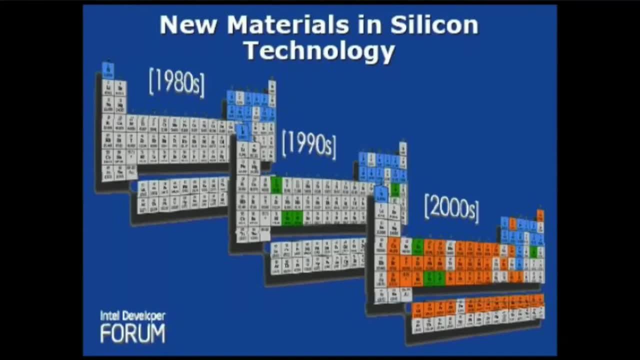 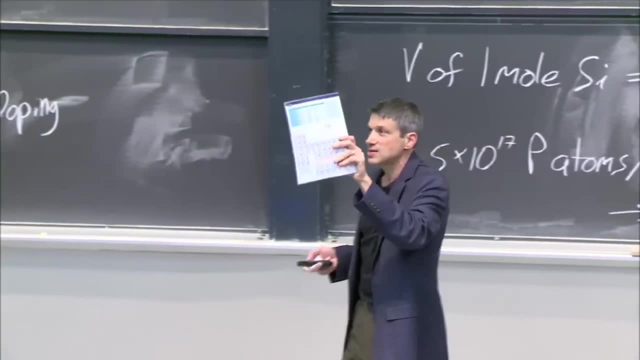 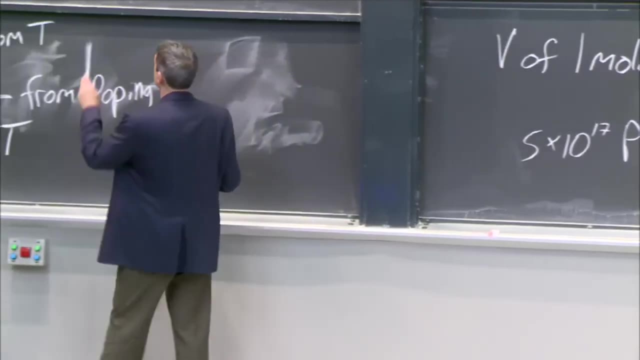 And today it's 75% of this- It's literally 75% of this- is in your phone. Why? The reason is exactly what we've talked about today: because they need more and more and more flexibility and ways to tune the band gap and the semiconducting properties. 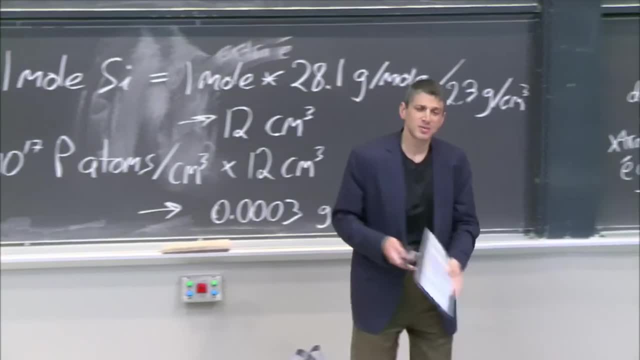 of these materials and the doping. Why do they need new ways? Because they're making them so darn small. They're so small it gets harder to figure out how to do it right, how to do it in a way that's also stable. 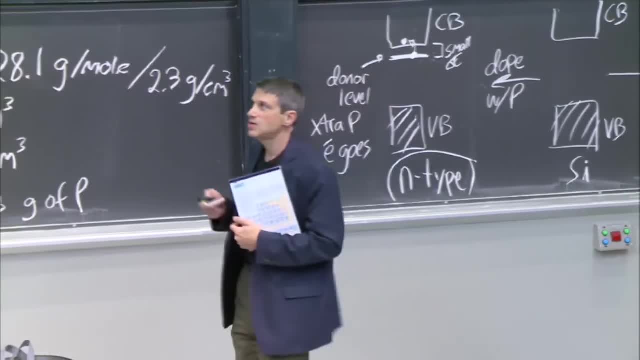 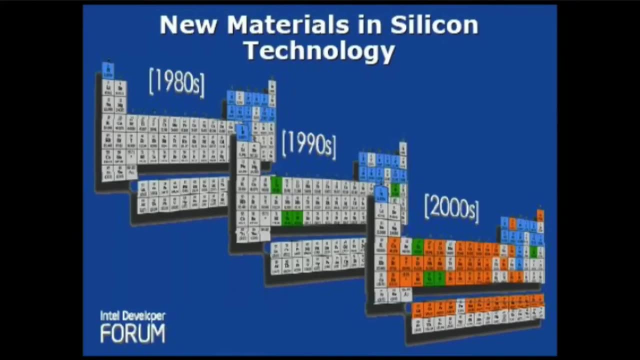 over time, for example. right, So they need new chemistry. This is a call to action, This is a call to the field of chemistry, And chemistry responded, And there's the data on the cost. I thought that was kind of cool. 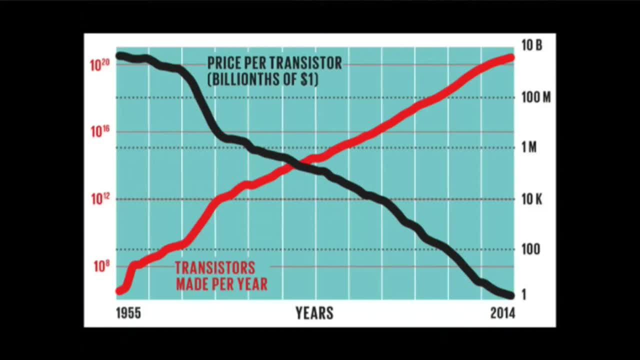 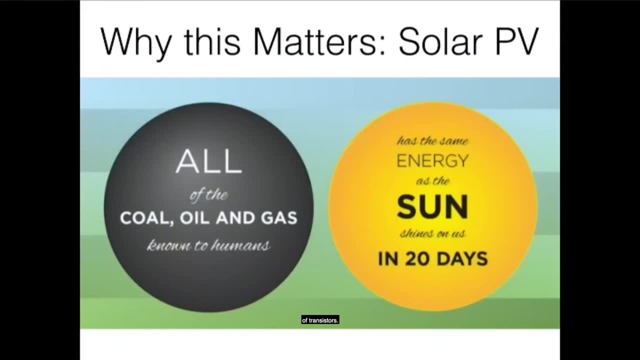 OK, so these are orders of magnitude of cost and number of transistors. And I'll just say one more why this matters: Because the semiconductor is also the same thing we use to take electricity from the sun, to generate electricity from the sun. 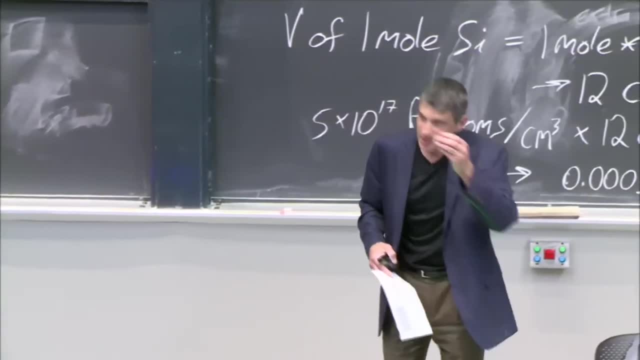 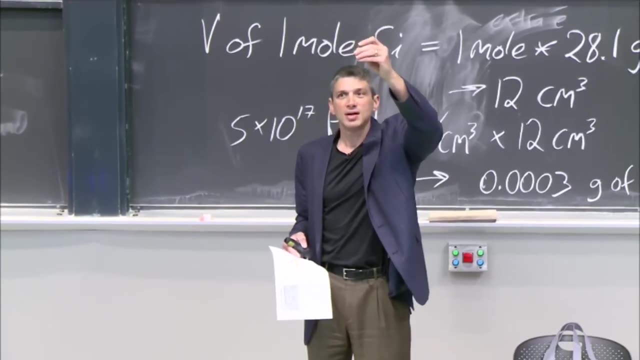 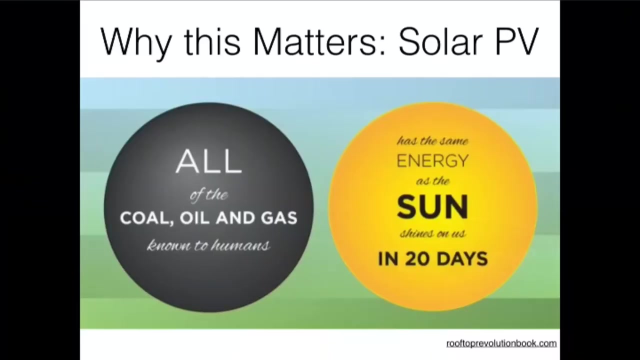 You can imagine You are doing that in your goody bag. You're literally using this semiconductor to generate electricity by shining light on it. Why is this important? Well, I like this comparison: All the coal, oil and gas known to humans. 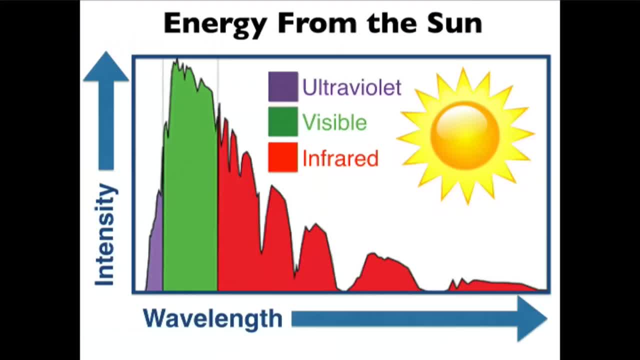 is what you get from the sun in about 20 days. This is the sun Now. we've seen the sun before. This is how we see it in our class. The sun is a spectrum of different wavelengths and intensities, And this is already on planet Earth. 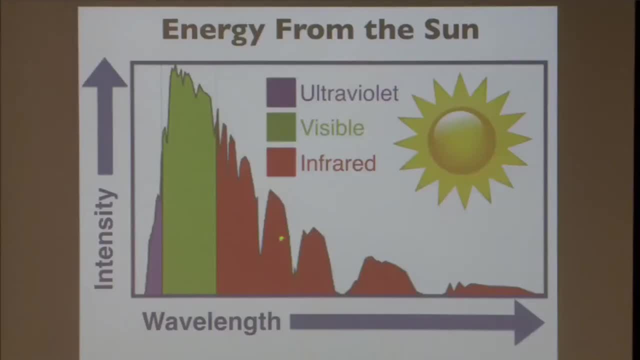 Because you can see, those chemistries that are in the atmosphere have already absorbed. Remember ozone down here helping us with UV radiation, And out here you've got a lot of water and other things- CO2.. Those are absorbing. That's why it doesn't look smooth. 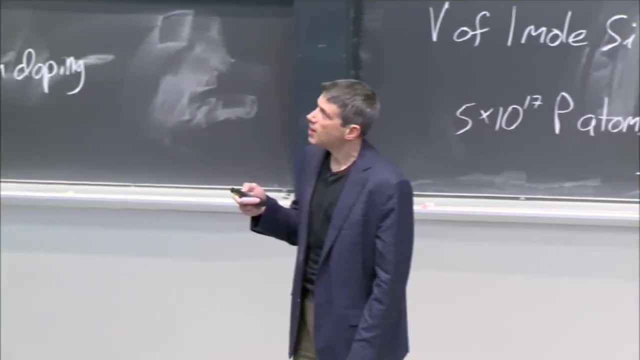 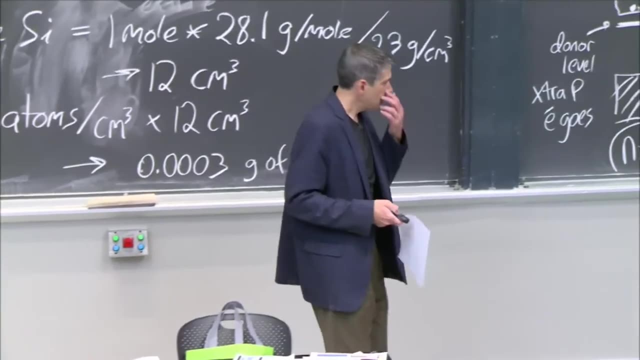 But the point is, I want a semiconductor to absorb as much of this as possible. If I want a good solar cell, I should absorb as much of this as possible, But the problem is that it's a constrained optimization problem. So let's see. 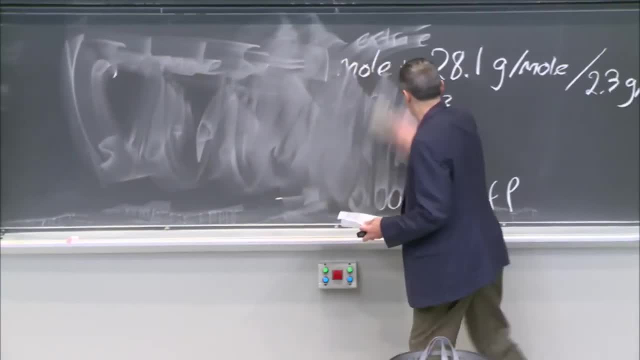 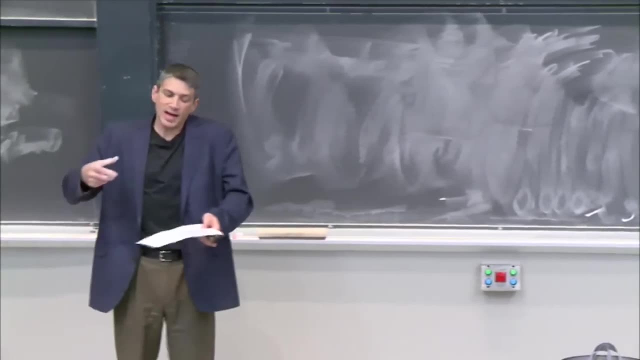 I'll just use this If I have a. you know I'm now. this goes back to Bohr, by the way. Remember Bohr absorbing light. It's just now. I've got an actual solid. I don't have an atom. 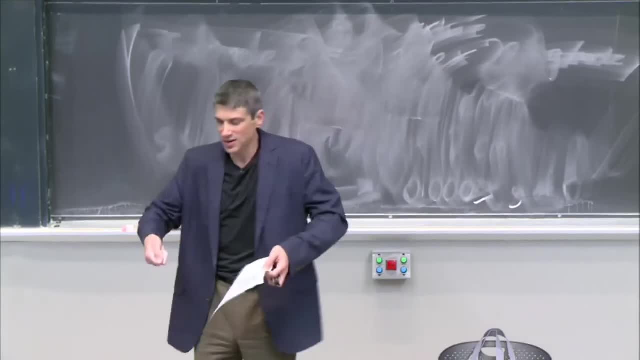 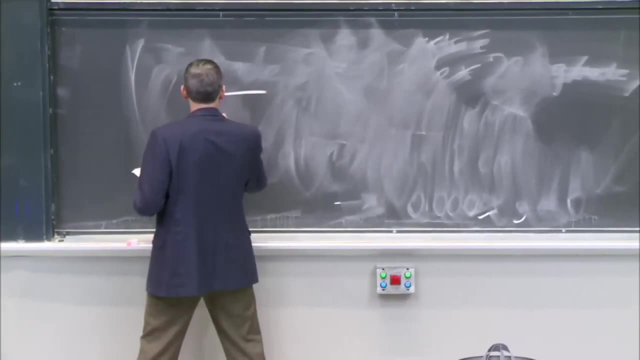 I've got a solid, which is what you need. if you want to generate a current, I've got to hook leads up to it. My solid is a semiconductor And you can imagine say: well, if my gap were really really. 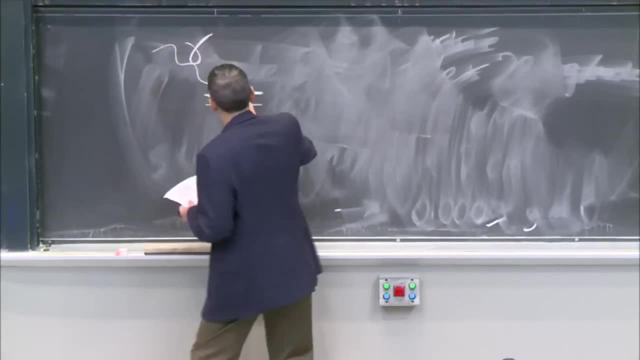 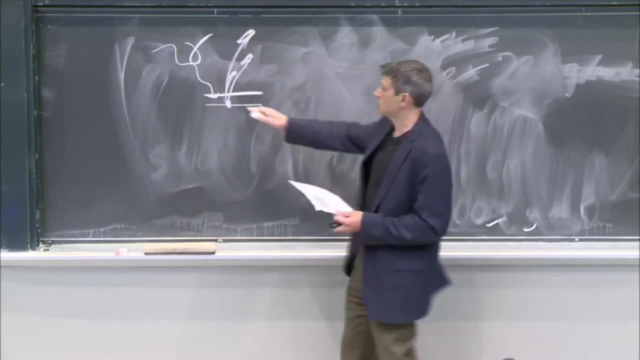 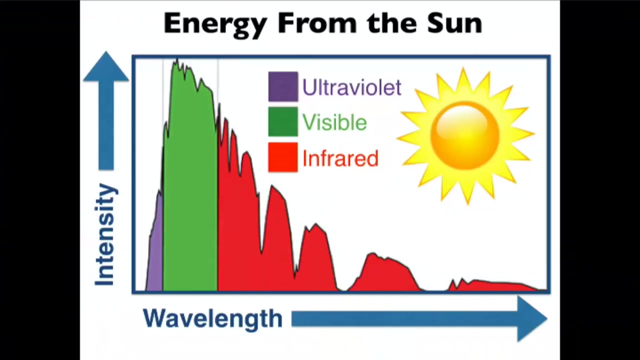 tiny, then any amount, almost any amount of this spectrum would excite electrons And I might grab most of that spectrum, I might absorb most of it. But the problem with that is that then all of these will thermalize, like I said in the beginning. 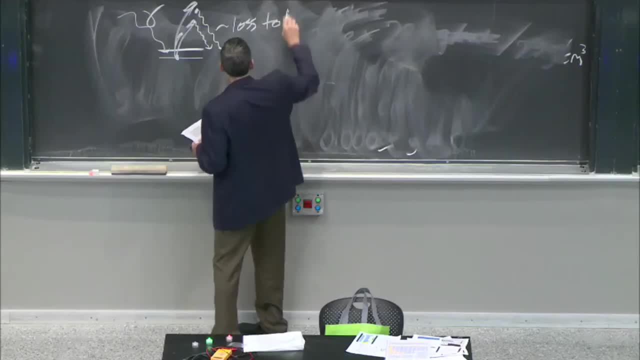 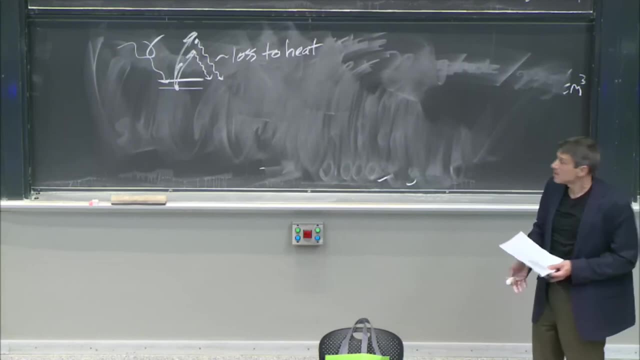 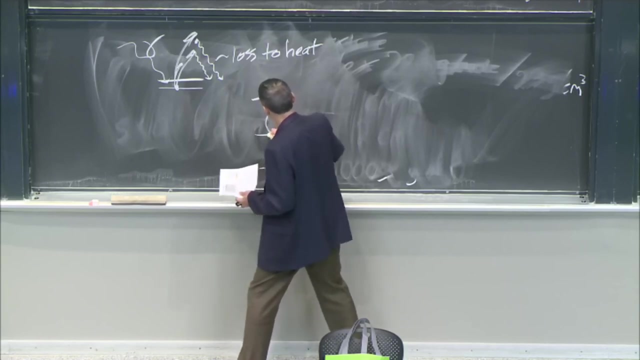 Lost to heat. lost to heat. So if my band gap is really small, I absorb a lot of the light, But I lose most of it as heat. But if my band gap is really big, then there's so much of this light that I cannot absorb. 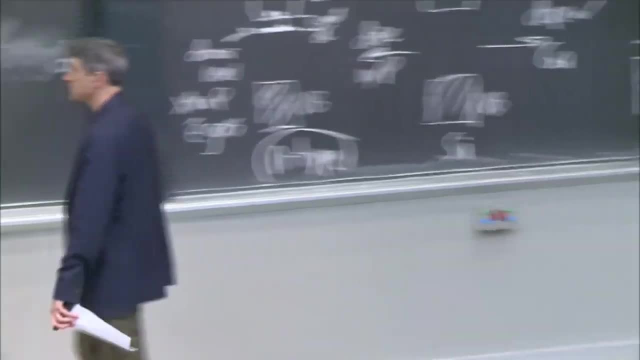 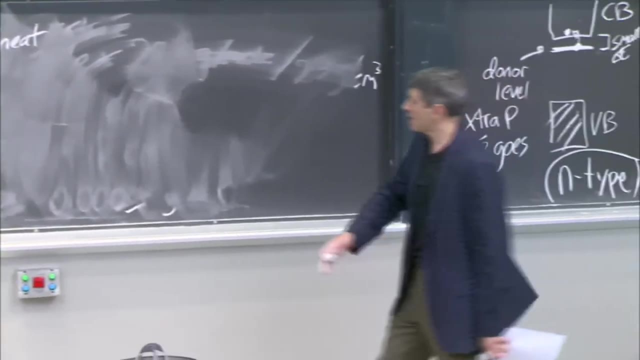 By the way, also the voltage that you get out of your solar cell is essentially this band gap. So if I get to really really small band gaps, I have almost no voltage. That's bad too, But if my band gap is too big, you think? 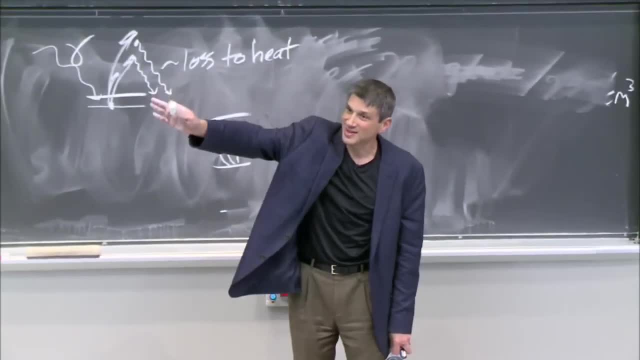 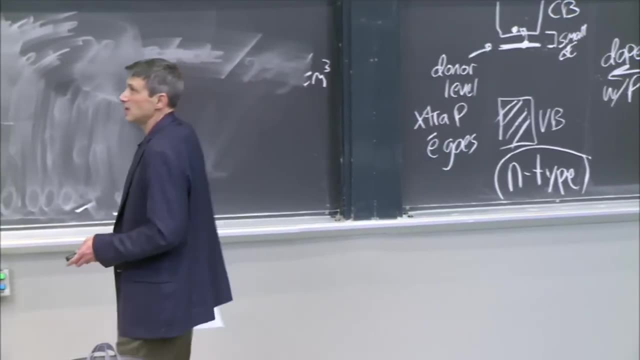 oh, I'll get a high voltage. No, you won't absorb any photons, So it's a constrained problem. It's a constrained problem And you can actually solve this And you can plot. in fact, here's a little animation. 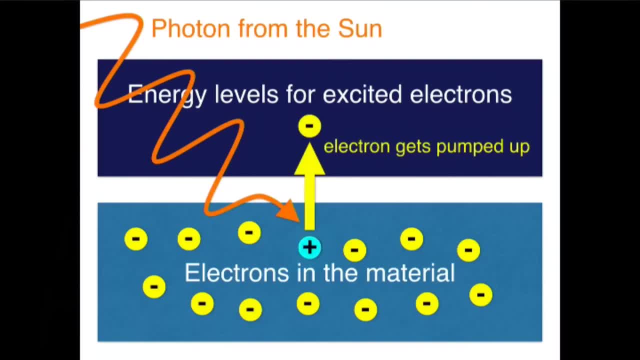 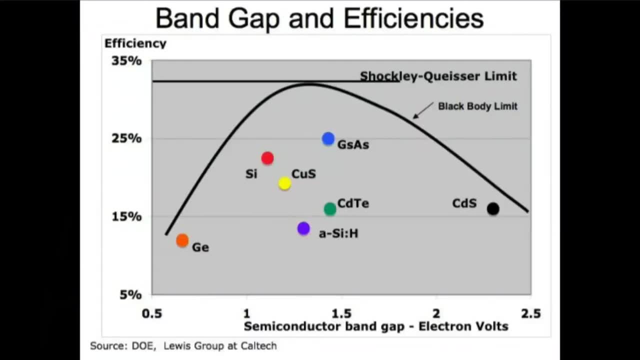 Oh, energy comes in from the sun. It excites an electron. This is how PowerPoint sees. it Leaves behind a hole and you get them out. That's the solar cell And this is the chart I wanted to show you, Because, you see, if I take this constraint into account, 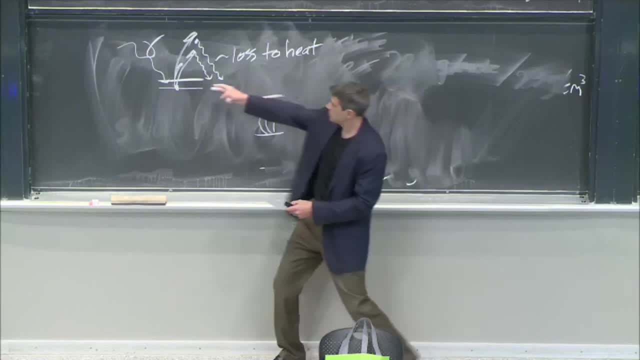 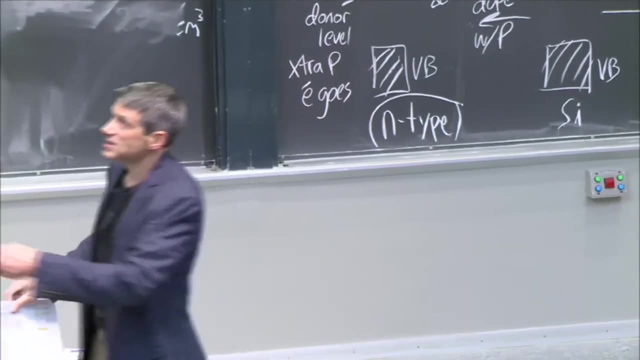 that I don't absorb light if the gap is too big. but I do absorb light and it all goes to heat. if the gap is too small, it means there's some sweet spot. There's some sweet spot And that's what is plotted here. 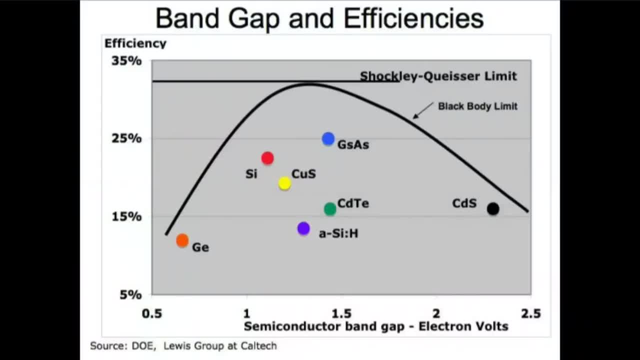 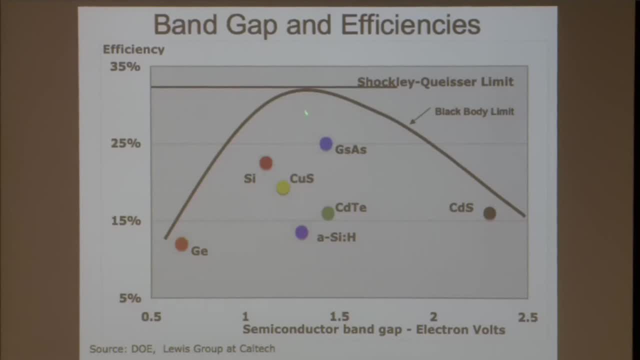 This is the band gap of a semiconductor And this is the maximum that that solar cell efficiency could be. That's the maximum that it could be for that gap. So you can see, the sweet spot is right. there is right there. That's a thermodynamic derivation called 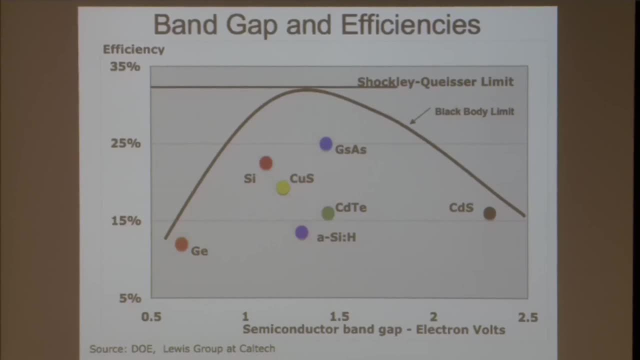 of the maximum efficiency you could ever get out of a single material And notice if you put the materials here- silicon is 90% of the solar cells you buy today- And notice that it's not quite at its maximum potential. It's also not quite in the middle where you'd want.